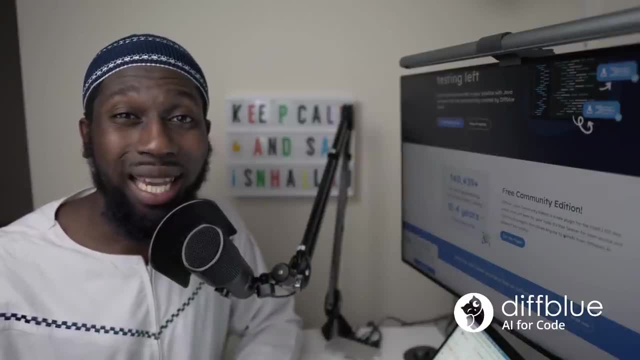 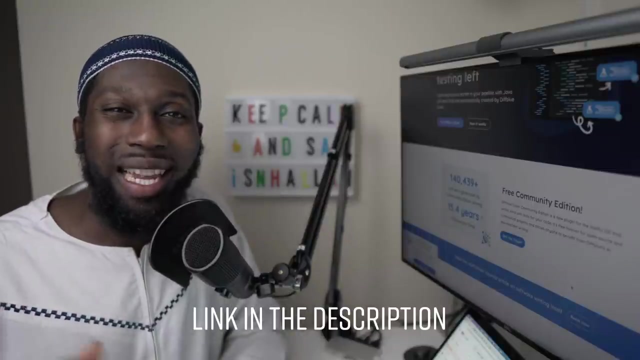 crash course And for those watching this video, you can get a license upgrade. allow you to write unit and integration tests for Java, commercial or open source projects. The link will be in the description of this video. This is all for now. Let's begin. 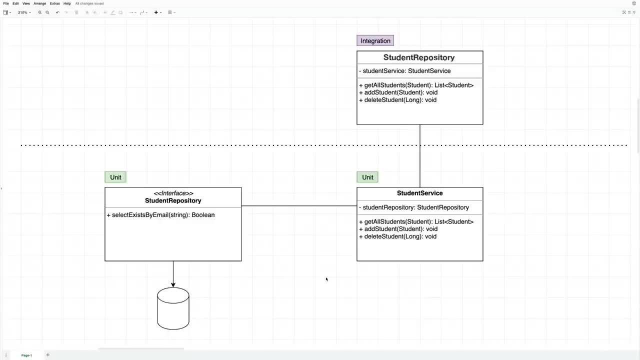 In this section, let's go ahead and focus on testing. So right here I've got the UML diagram for the application so far, And what I want to do here is to break it down for you Super simple, So you understand exactly how. 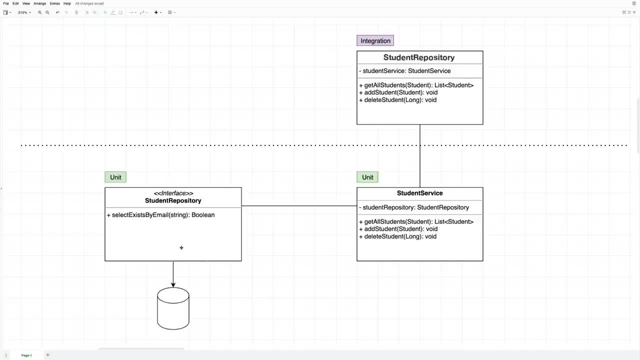 to test your applications. So in here, remember, we have the student repository and this is an interface And we have one method right here called Select. exists by email And then it takes an email of type string and then returns true or false And the plus sign in. 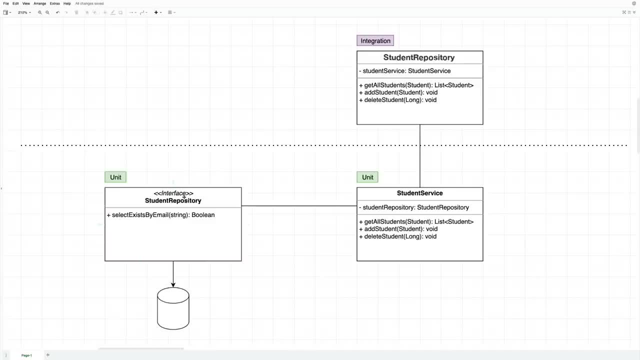 here means that this is a public method. Now remember, this interface right here is responsible to talk to our database right here. And then we have the student service And this service right here has a private field. So you can see that the minus sign. So this means a private field. 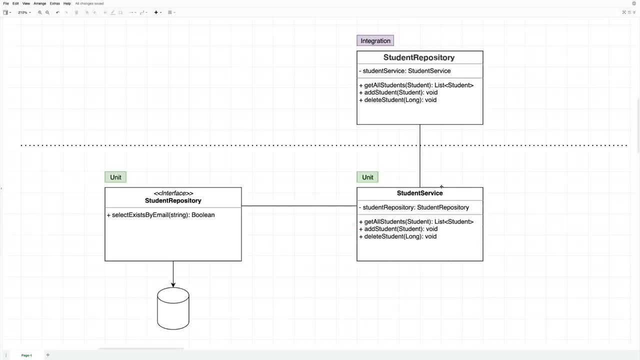 of type student repository. So this service uses this interface right here And then it has three public methods: Students, which takes a student, and then returns a list of student. Then we have add student which take a student and a return type is void And finally we have delete. 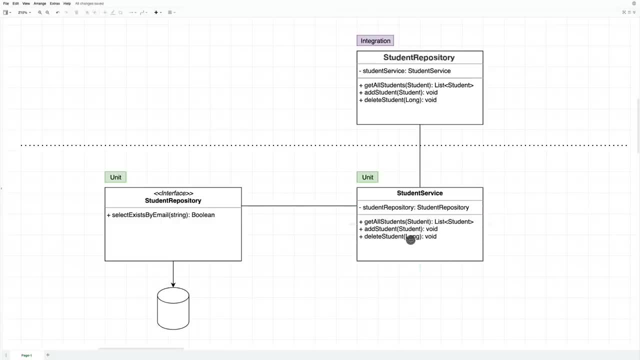 student, which takes the ID of type long and then returns nothing, Right? So this is void right here. So, both student service and student repository, These are the units, And I'll tell you why in a second. So these are the units that we want to test. 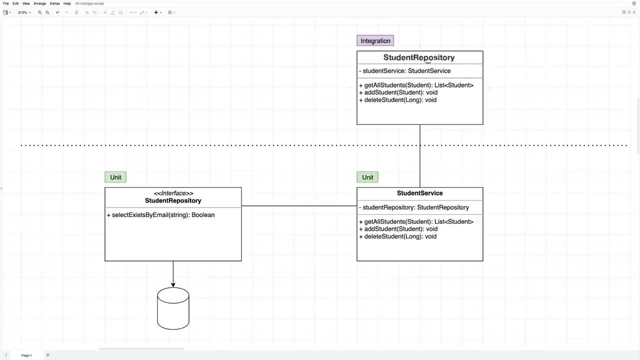 And then in here we have the repository. So this repository, remember, it's responsible for taking all the requests from the client. So this is our API in here, And this is why I named this as integration, And you'll see why in a second as well. But basically, 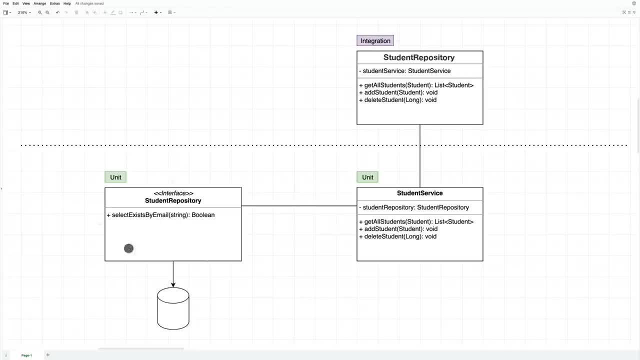 what we need to do is: let's start from this side, right here, where I'm going to show you how to test the repository, And then we're going to move into the student service, And then I'm going to show you how to properly test. 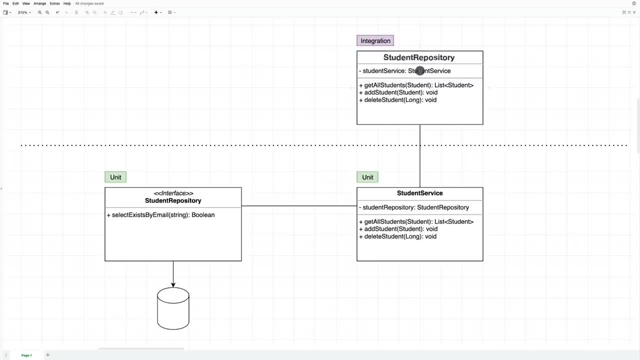 the repository as well, So the student repository. So testing is something that you should really master and you should know how to test your applications properly. If you are serious about programming and writing good quality software, then testing should be one of the things that 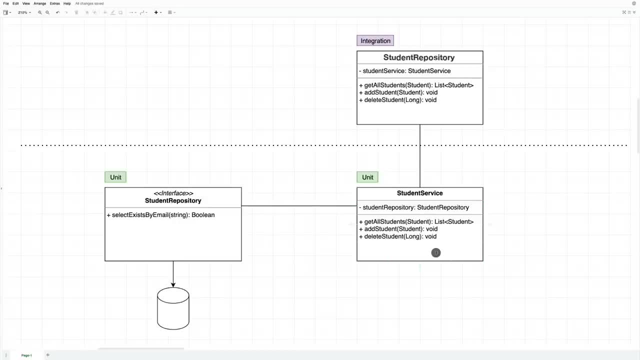 you have no second thoughts. It should be something that you have pleasure doing, and you'll see that testing is not that difficult. So previously I've worked in companies where they didn't do any testing And, to be honest, the code quality was. 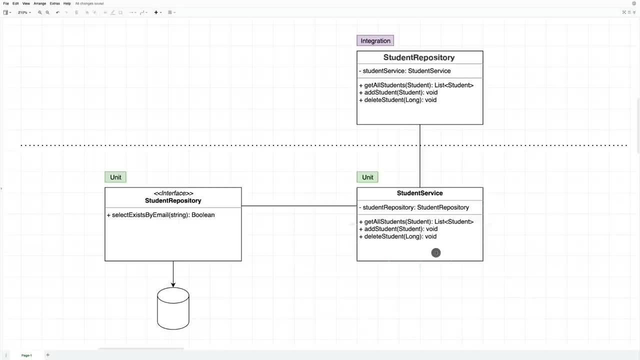 really bad, And deploying the application to production or to any environment was really frightening, because having no tests gives you no assurance of the quality of your software. So if you introduce a new feature, then you don't know whether you have broken anything. So that's. 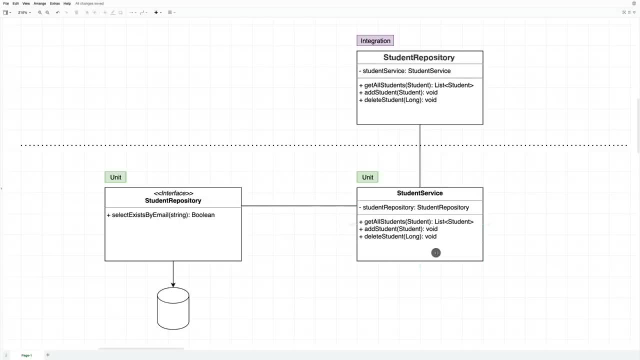 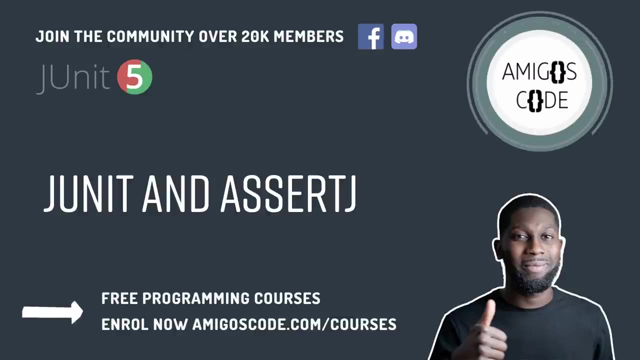 the power of testing. So I want to make sure that you fully understand how to test your applications. And next, let me go ahead and show you exactly what we need in order to start writing tests, In order to write tests in the Java world. 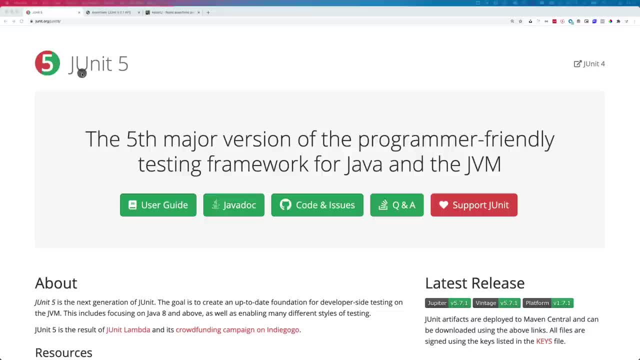 you will most likely be using JUnit five. JUnit five is the fifth major version of the testing framework for Java and the JVM, So they say that JUnit five is the next generation of JUnit, And this is because from version four to version five there was a massive refactor. 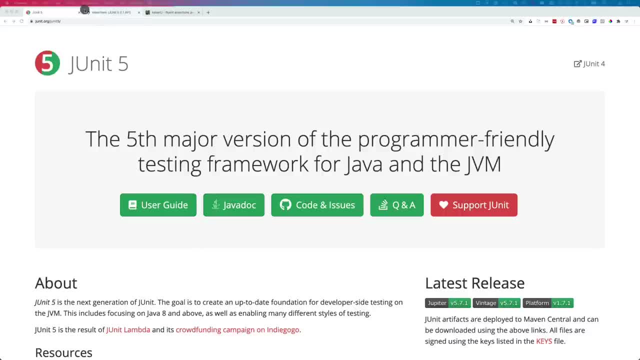 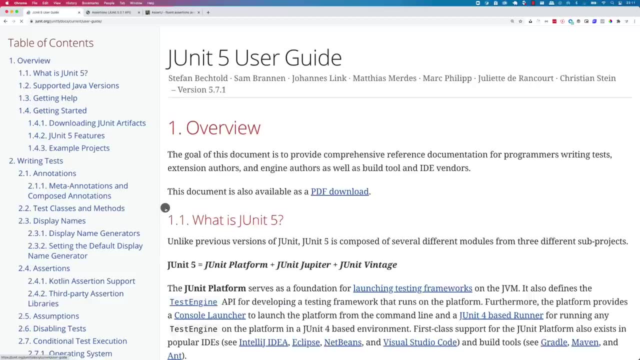 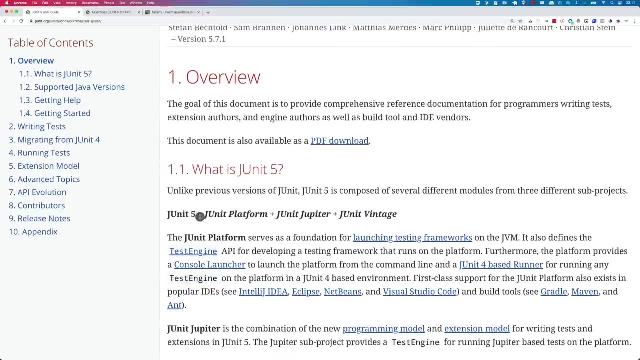 and improvement. Now, in here I'm going to click on user guide, and you can find the link under the description of this video. So let me click on it And right here they give you an overview of JUnit. What is unit five? So it's equal to the. 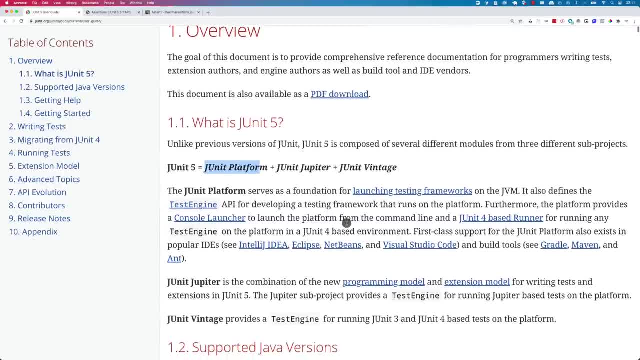 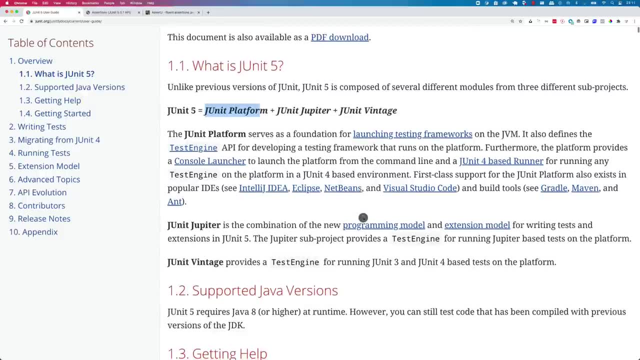 platform, Jupiter and vintage, And right here the platform serves as the foundation for launching testing frameworks on the JVM. Then we have the Jupiter, So combination of the new programming model and extension and extension for writing tests. So these are like the annotations that you'll see in a second. And then we have 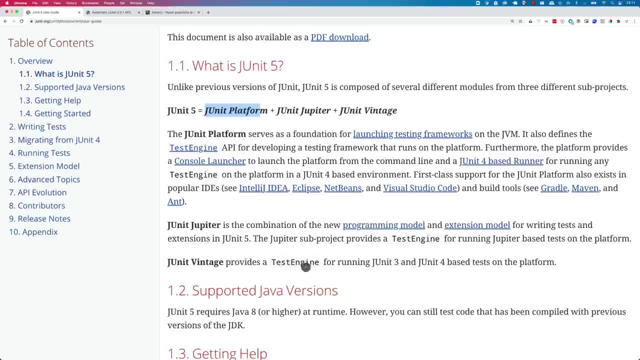 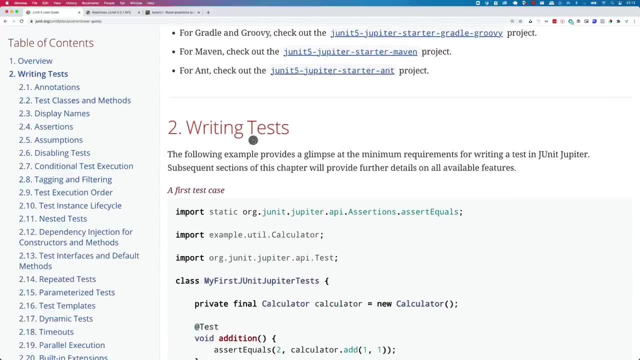 the vintage, which is basically a test engine for running JUnit three and four base tests. So these are the older versions of JUnit. So right here, if I scroll down, you can see that we have this section. So writing tests, and have a look. 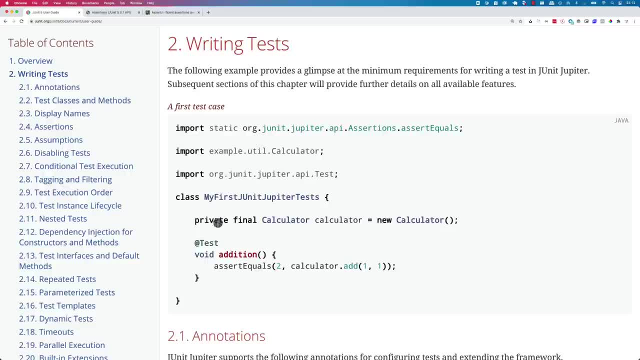 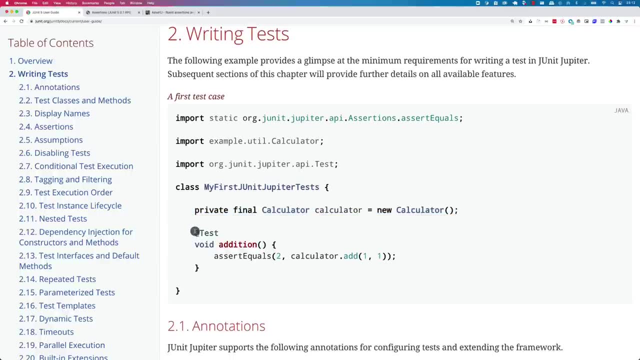 So this is how you write test: So you have a class and then you have your under test- So in this case calculator- And then you have a method in here, So void, you give it a name and then inside you'll be performing. 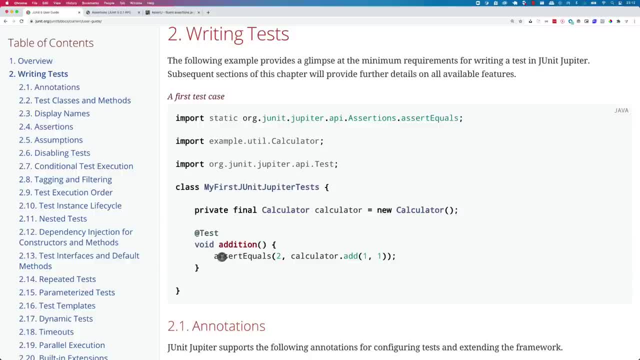 one or more assertions. So here you can see that assert equals, And then this is the expected value, And then the actual is when you invoke the under test class, In this case calculator add, and then one plus one And this should equal true. 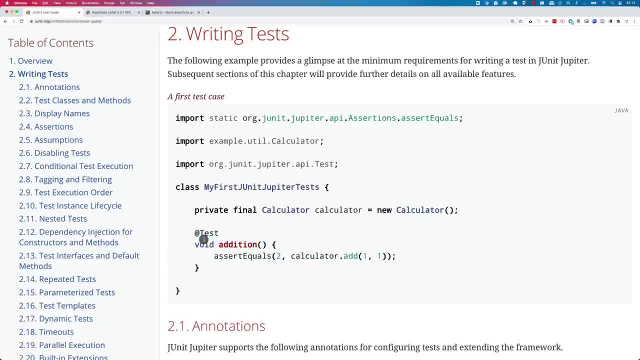 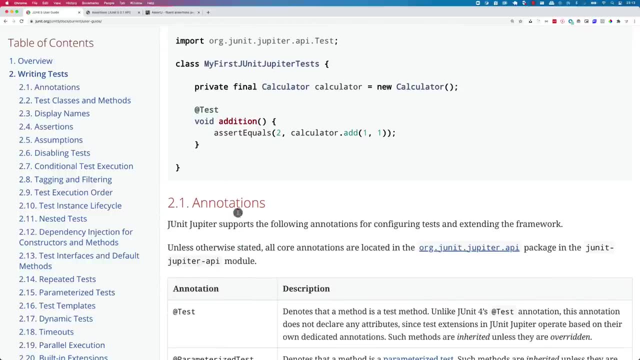 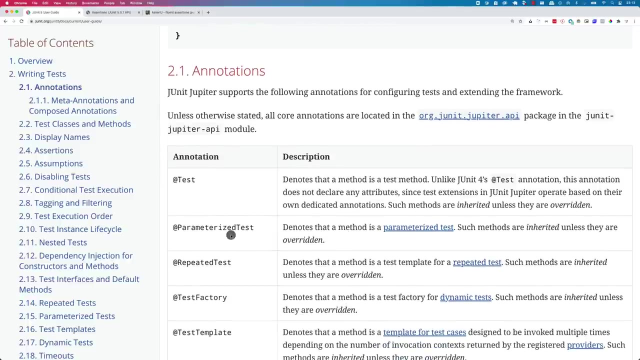 Therefore, this test will pass. So in here you have a bunch of annotations And in here you have a bunch of annotations that you can use. So at test the notes that a method is a test method. And then you have parameterized tests, repeated tests, factory template. 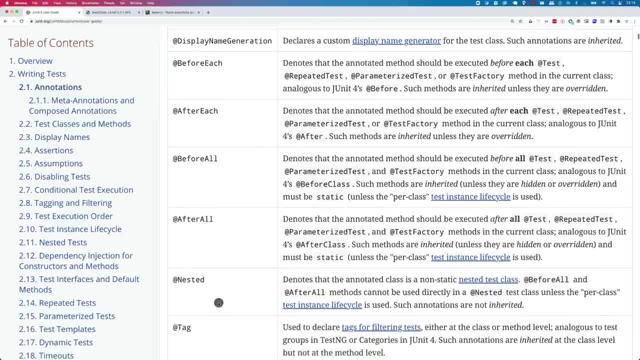 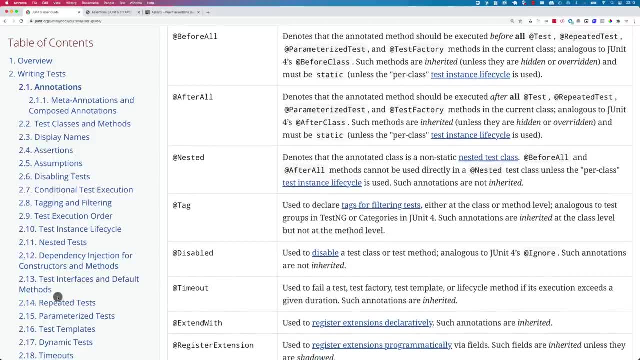 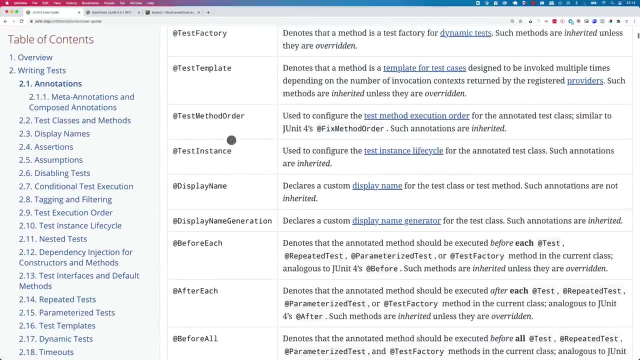 display name before each, after before all nested tags on and so forth, And you can even disable a test as well, including timeouts. So right here you can go and basically just read about all of this documentation And one thing that I want to show you here: 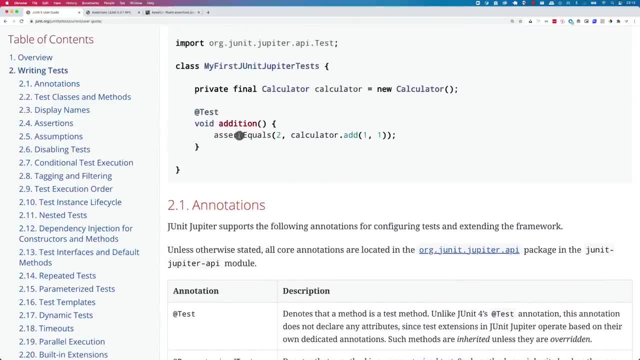 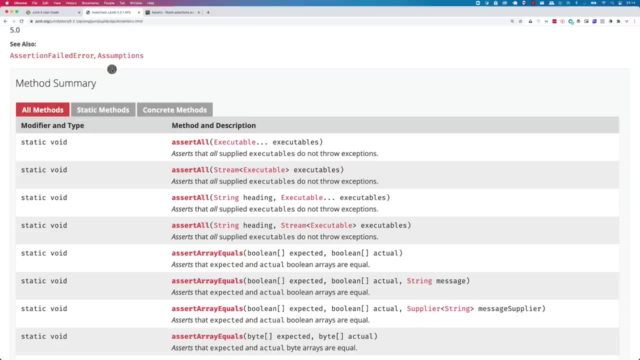 before we move on, is that you see that we say assert equals. So in here this is how you perform the assertions, If I click on this tab right here. So this is where I have the assertions And this is the class assertions for J, unit five. 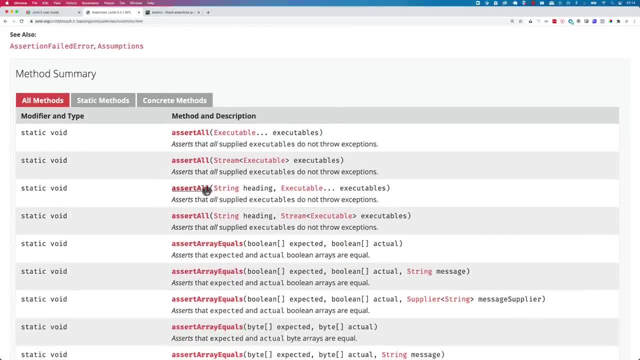 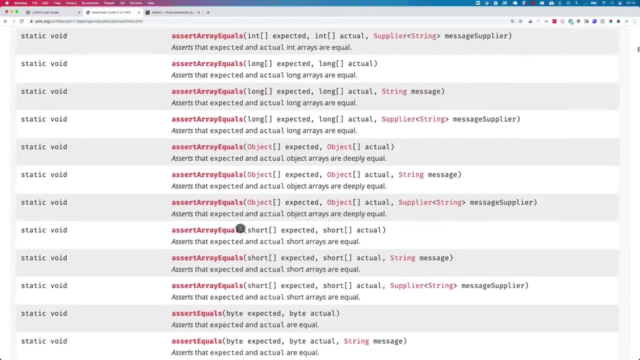 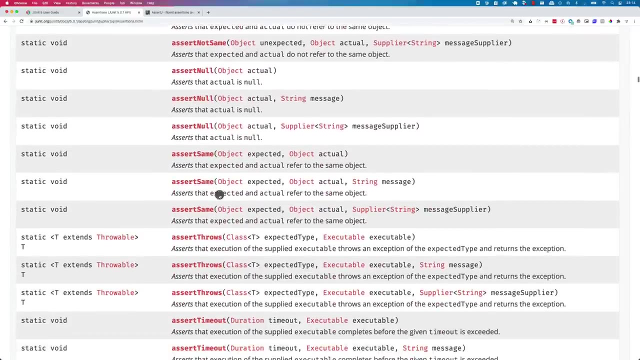 And basically you can see all of these methods. So assert all where you can pass a string, And then you can basically say assert, array equals. And if I scroll down you can see that a bunch of methods. So assert not equals, and then assert. 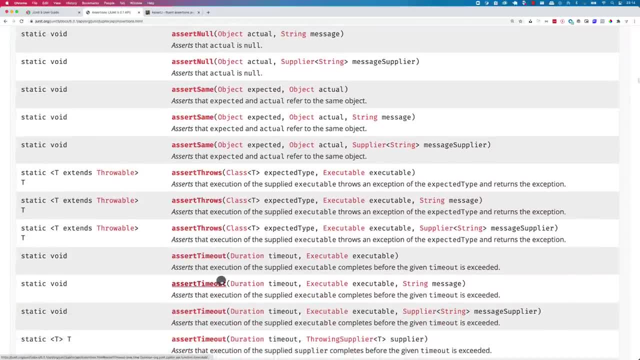 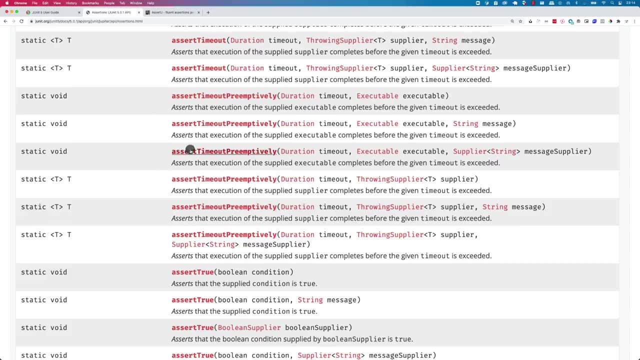 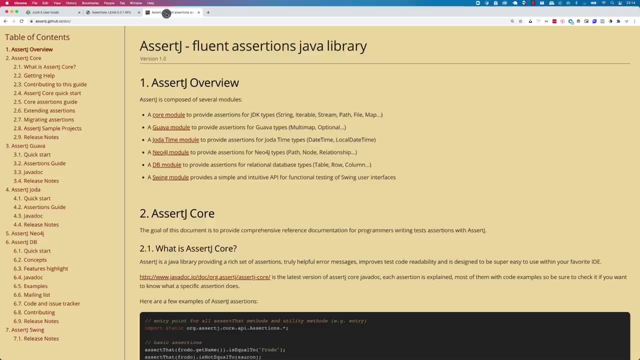 same assert throws for exceptions, time out, so on and so forth. So and also assert true for booleans. So in here, what I'm going to show you is there is a better assertion library that the one J unit five provides, and that is assert J. So assert J provides a rich 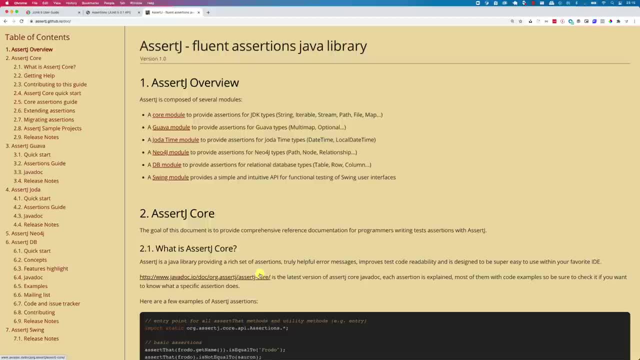 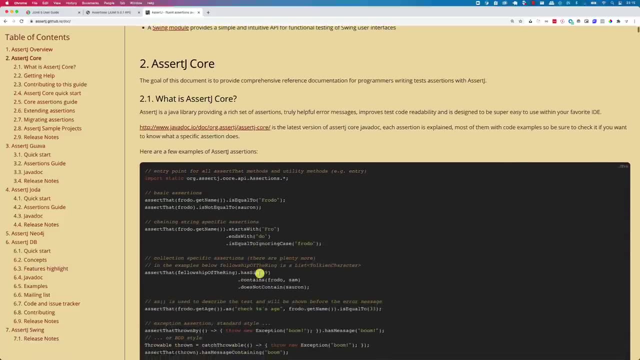 set of assertions that improves your test code readability and it's designed to be super easy to use within your favorite ID. So here you can see that, for example, this is how you use it. So if I zoom in a little bit, 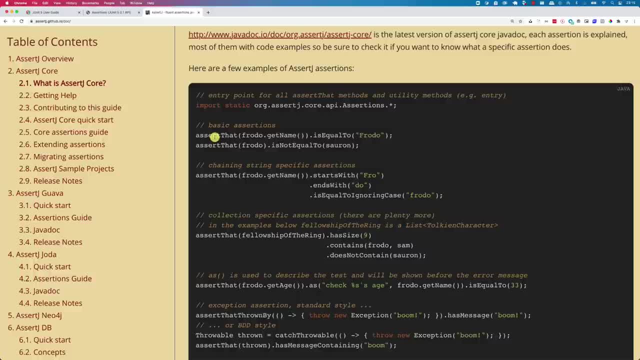 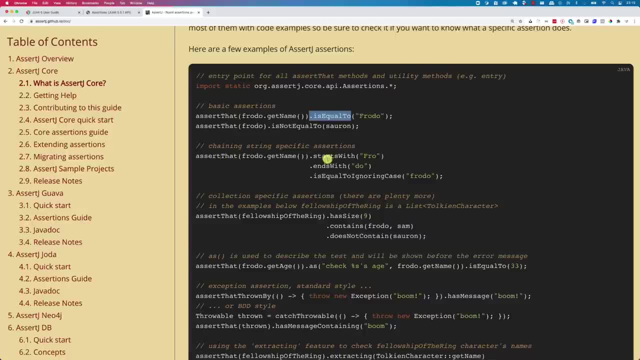 so you can see that you import a serve for J and then you can say: assert that, and then dot is equal to, And then you have methods such as: assert that, and then starts with ends with, And basically you can chain all of these Right. So the same with. 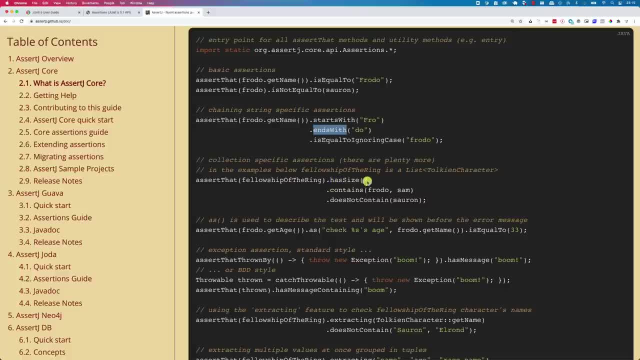 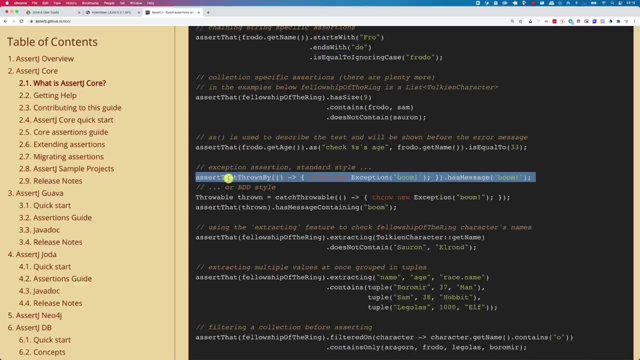 arrays or lists. you can say: has size, something, and then contains, does not contain, and also asserting, for example, exceptions. This is how you do it, So on and so forth. So I actually prefer assert J instead of the assertions provided by J unit. 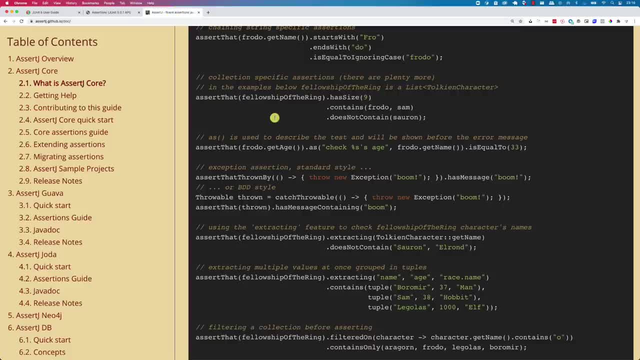 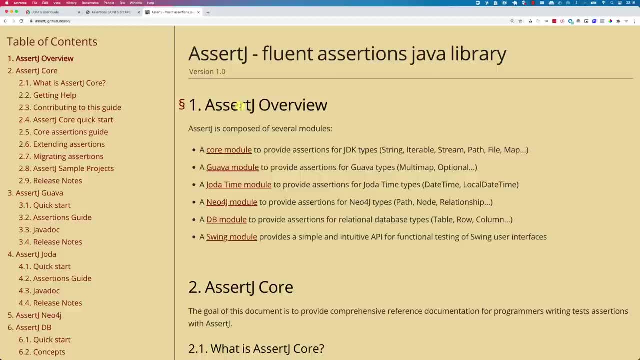 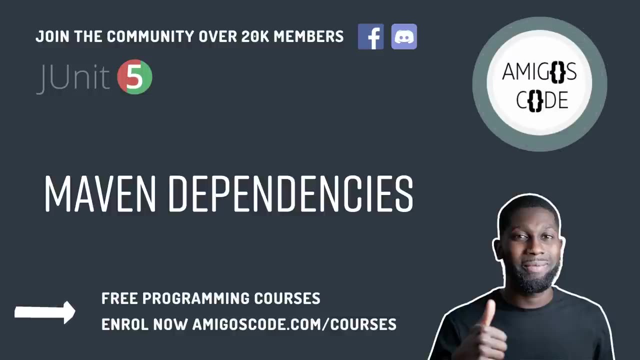 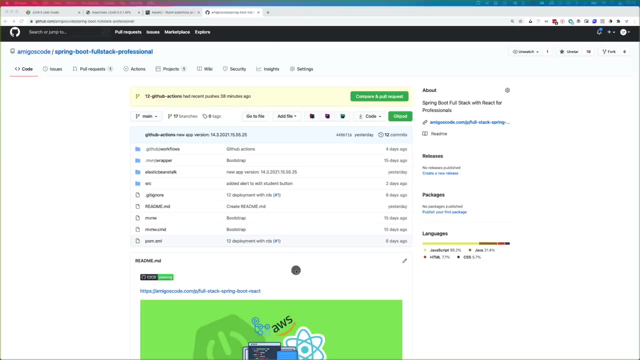 five, And this is what we're going to be using in this course. So now that you know about J, unit five and assertions, next let me go ahead and show you how to get your first test up and running, If you want to follow along and basically try for yourself. 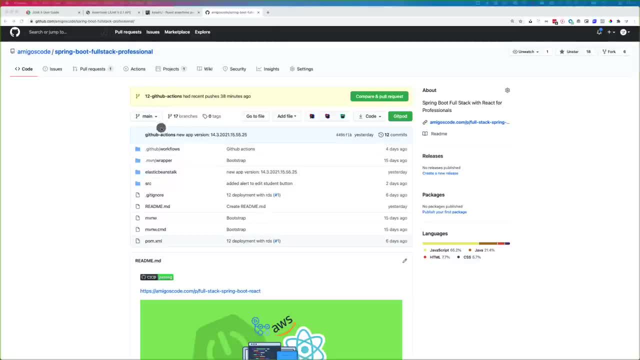 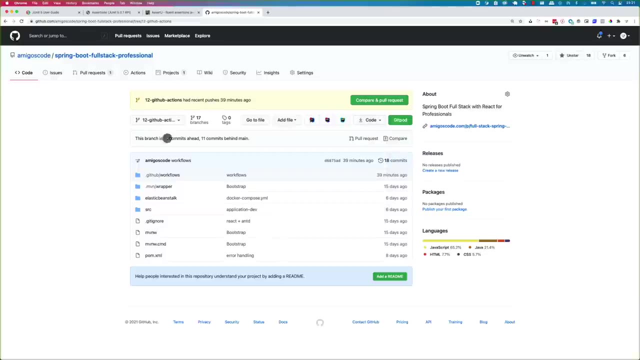 go ahead and basically clone this repo and check out the branch number twelve right here. So after get up actions, so you can basically clone this and then check out this branch right here, Or you can just basically just download the zip, But it's best if you use get. 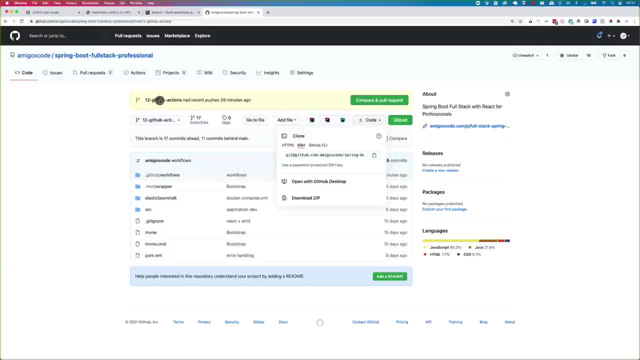 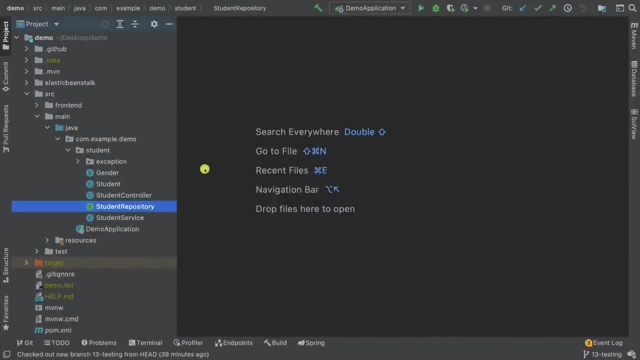 So I'm going to leave the link under the description of this video so you can just check this branch. Now let me go to IntelliJ, And in here remember I said that we have the student controller repository service And also we have a couple exception. 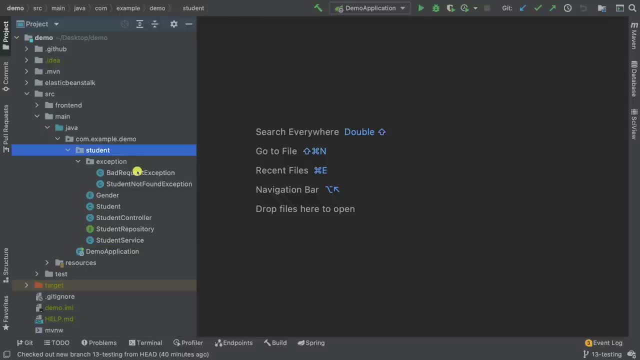 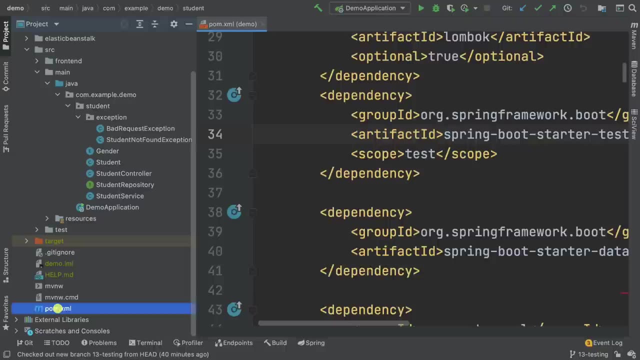 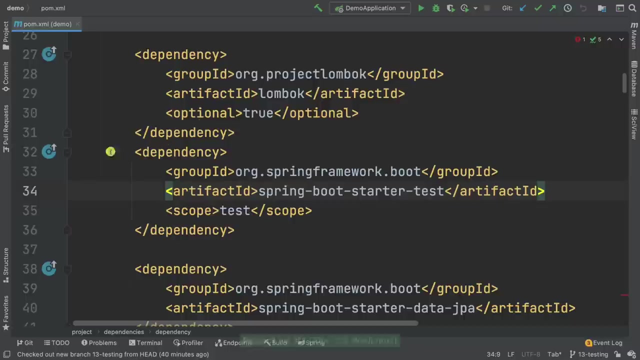 classes right here. So let me first show you that in order for us to get J, unit five, we don't have to do anything. So here, go ahead and open up the palm XML, And if I collapse, this for a second, and in here you see that we have this dependency. 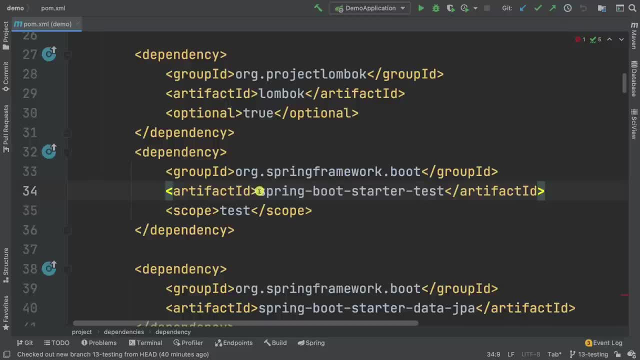 So org spring framework boot and then spring boot, start to test, And then the scope is test, which means we're just using this dependency for testing purposes. Now, if I click on this artifact right here, so I'm just going to press command and then basically click on it and you can see the keyboard. 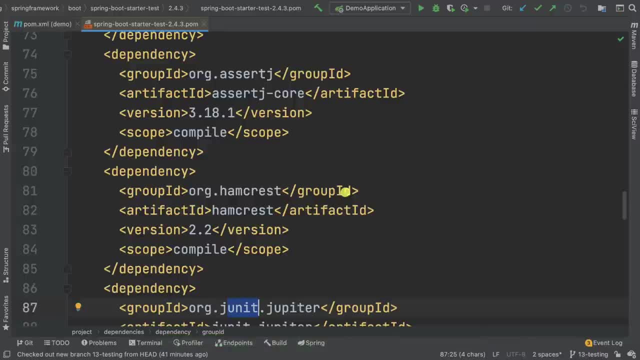 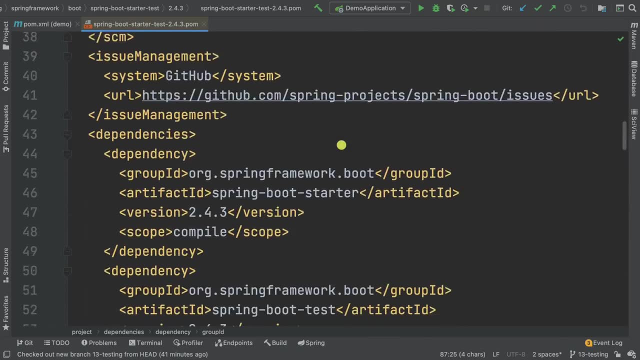 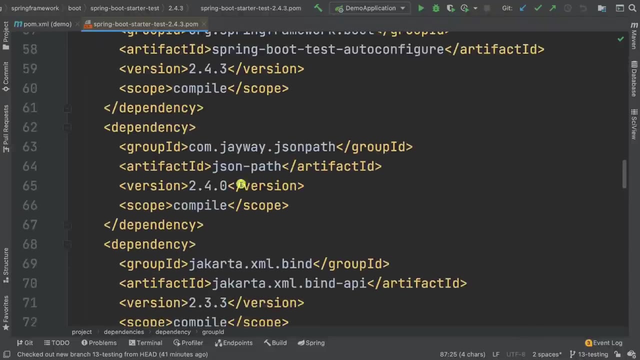 shortcut, command B or control B for Windows. Now in here. So basically we have a bunch of things, But if I quickly show you, So if I scroll down, you see we have dependencies And here we have some auto configuration JSON path. 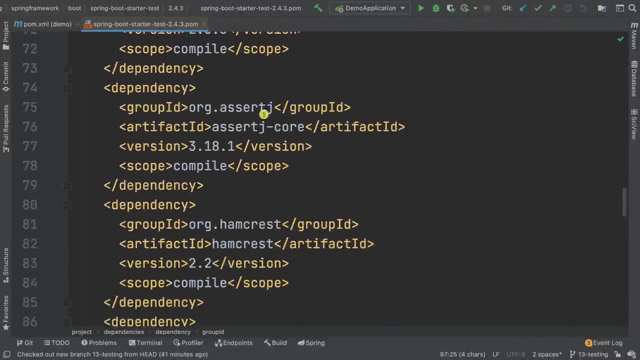 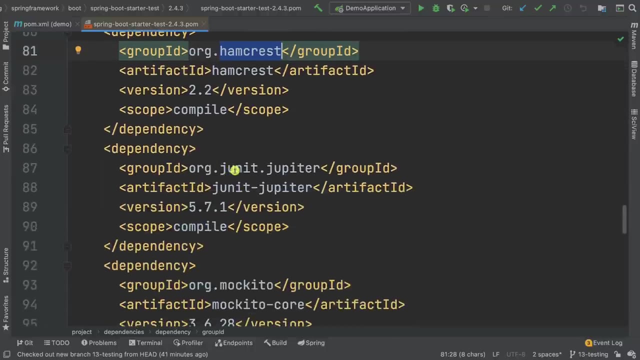 XML bind and have a look. assert J. So remember I told you about assert J, So this is already included for us, which is really nice. We also have Ham Crest, So this is another assertion library, And then we have J unit in here. Have a look. 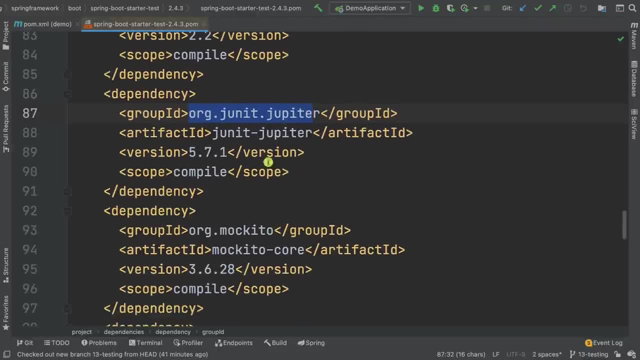 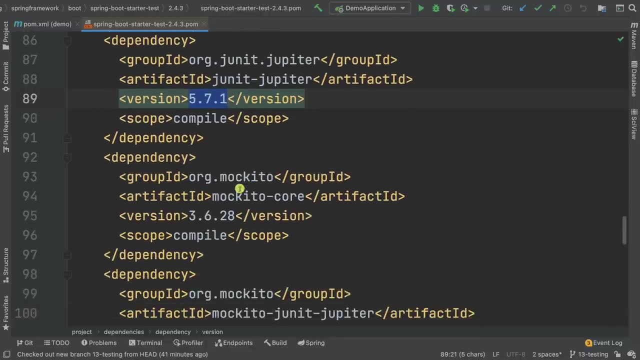 J, unit Jupiter, And the version is five point seven one. So this is the default that comes with the spring data test And we also have Mokito, So we're going to use Mokito later So we see how we do mock classes. 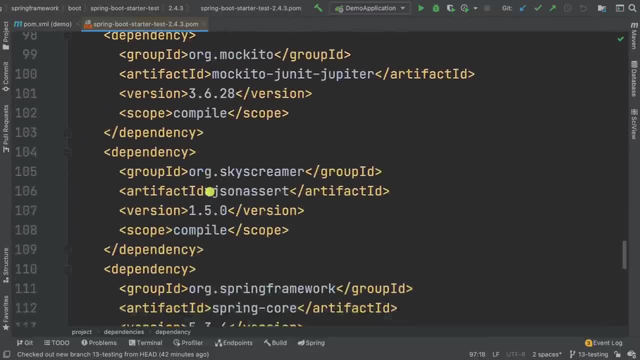 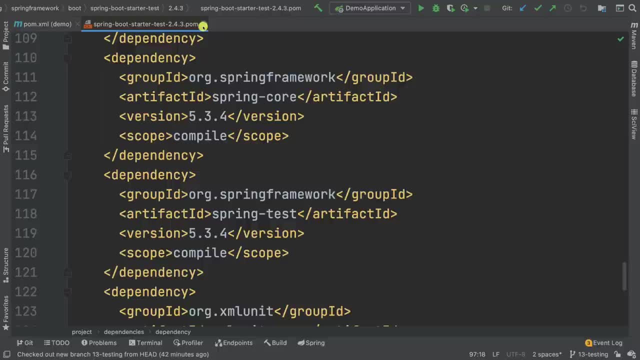 But this is pretty much everything that we need in order for us to start writing tests, So, which means that we don't have to go off and install anything, which is really nice. Let me close this And next let's go ahead and write. 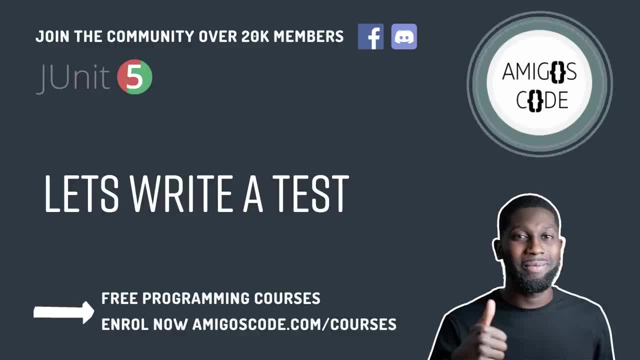 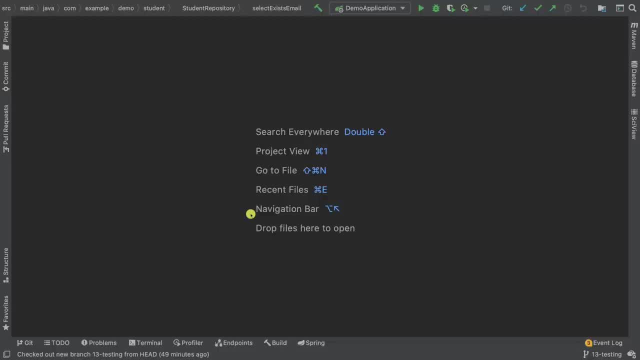 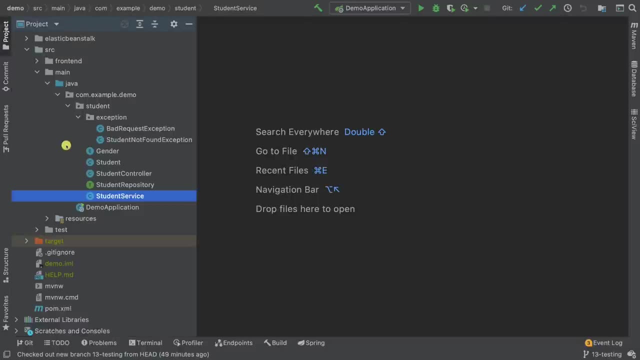 our very first test In order for you to write tests for your application in here. if I expand the project tab and you see that the Maven folder structure is so SRC, and then we have main, So this is where the main code lives, Right. So all of this you've seen. And then, if 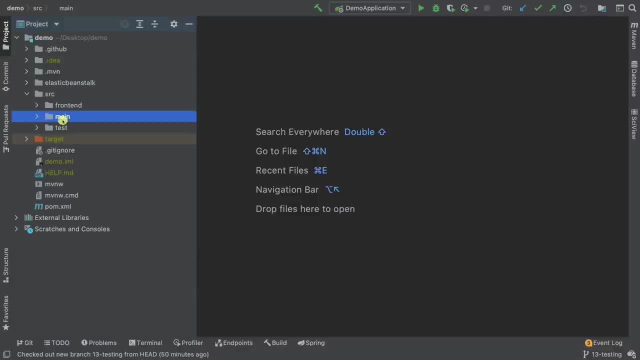 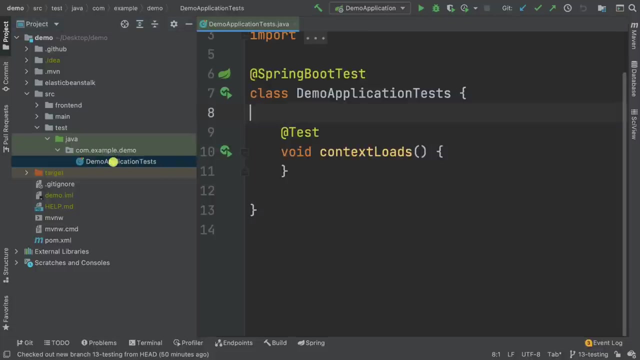 I put this back. you can see that. So we have main And then we have test. So in here test, So if I click on test and right here you can see that we have one default test. So if I click on it and have 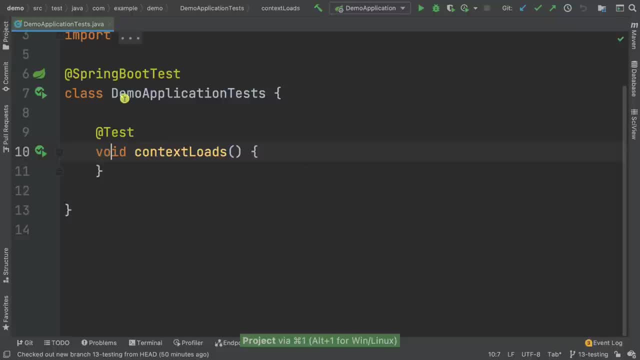 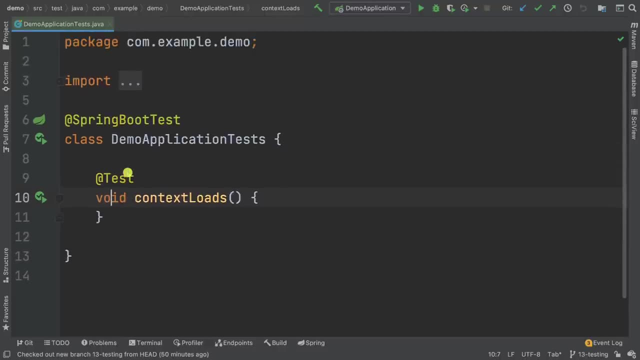 a look. So we have this class called demo application tests And then we have one single test, So this test doesn't do anything in here. We have this annotation at Spring Boot test, And I'm going to show you this in a second, But for now let's. 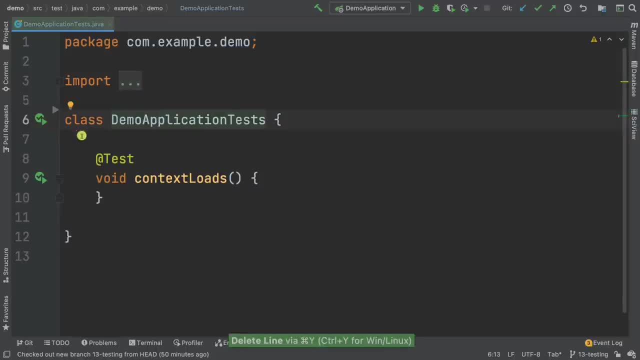 just delete this, And what we're going to do is let's just, basically, you can see that we have this play button in here or here, So basically, this will run all tests found within this class, or you can run a single test, So let's just 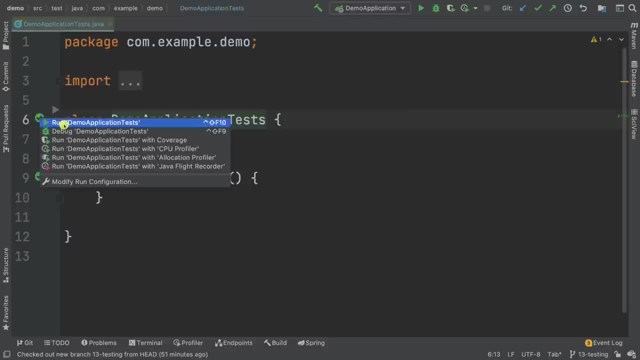 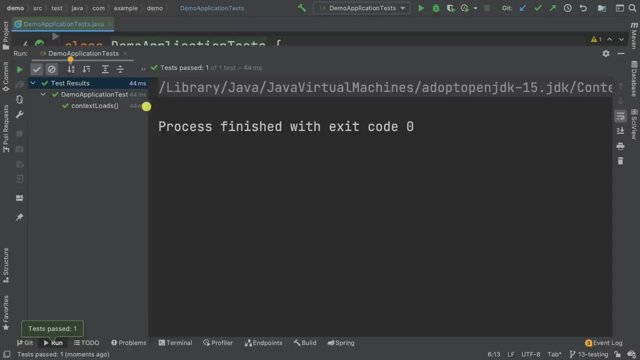 run all tests And you can see run demo application tests. And there we go. You see that the process has finished And here you can see that we have some test results. So this basically took 45 milliseconds. This was the class. 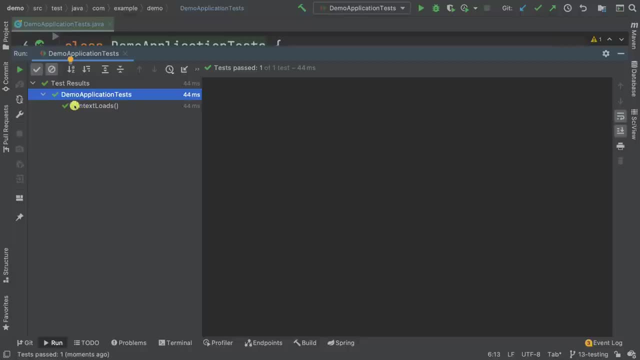 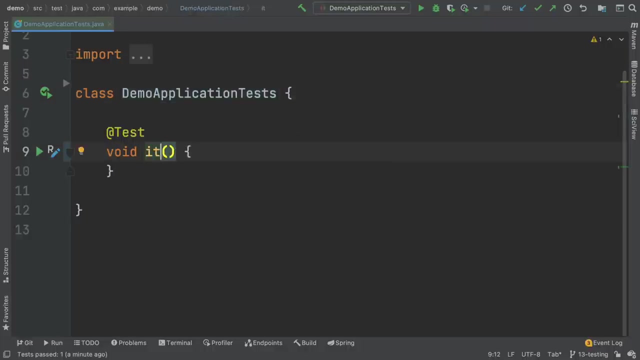 And within that class we had one test called context loads and it passed. So this test is pointless. So let's actually go and collapse this And let's change this to it, and then should, and then add, and then numbers. So here let me just create a class within this demo class. 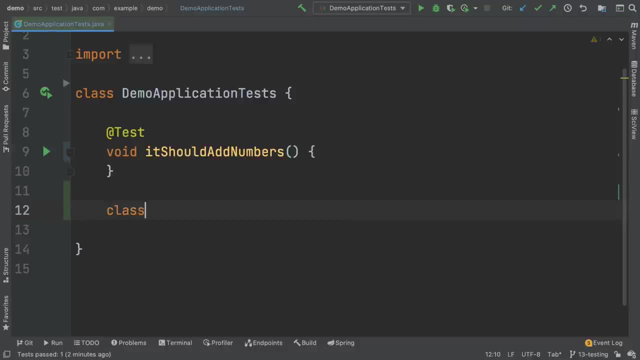 So here I'm going to say class, and then I want to say calculator, And then inside I'm going to have: so I'm going to say int and then I'm going to say add. This will take two integers, So int a and then int and then B And it's. 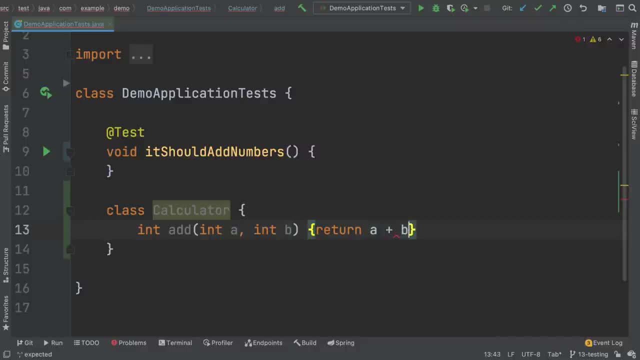 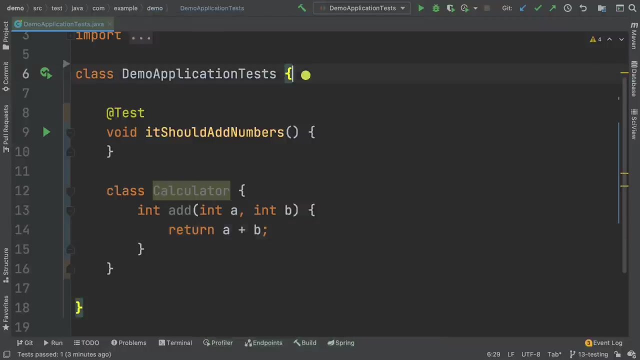 going to return a and then plus B. So this is the example that you saw before And here, if I basically in this with semi column there and in format things, and we have our calculator. Now let's create an instance of this class right here. So here we're going to say calculator. 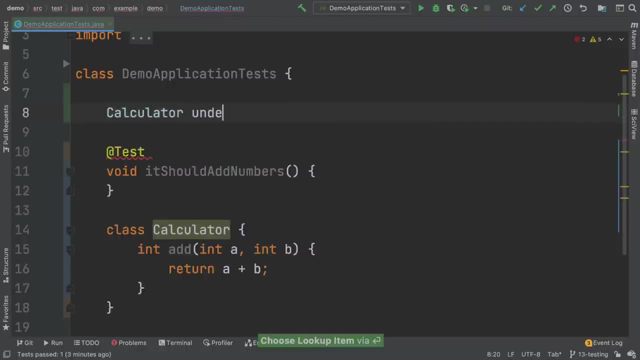 And I like to name these are under. and then test, because it's the class and the test equals to new. and then calculator. Now in here, what I like to do with my tests is to have comments to lay out the foundation. So here I'm going to say: forward. 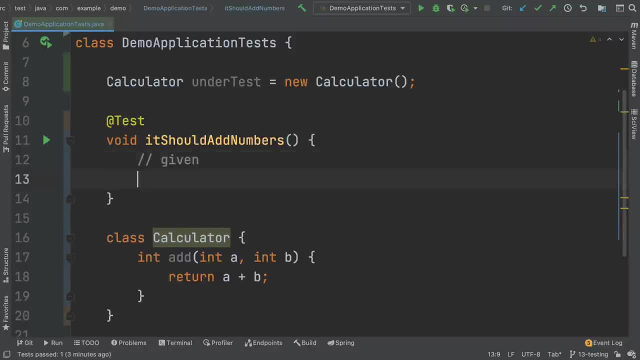 slash, forward slash, and then given, And then I'm going to say int, and then number one equals to ten, for example, or 20, and then int number, and then two equals two, And then let's say 30. And here I'm going to 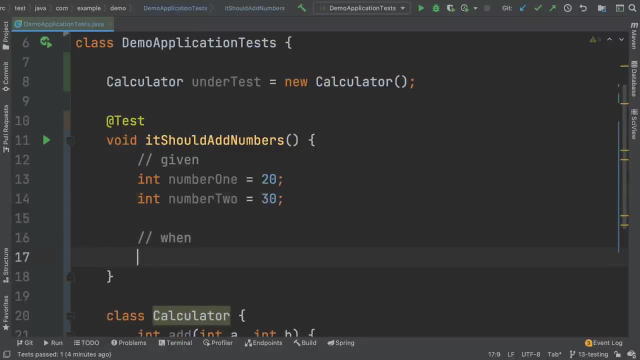 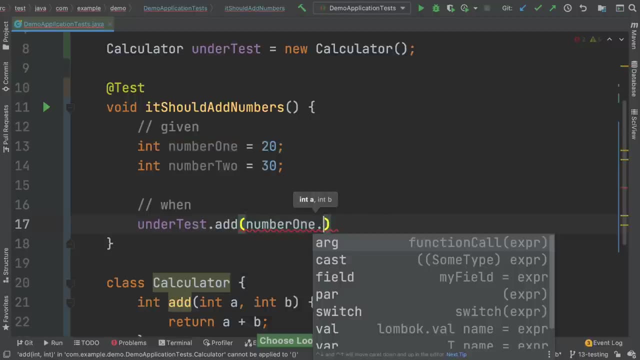 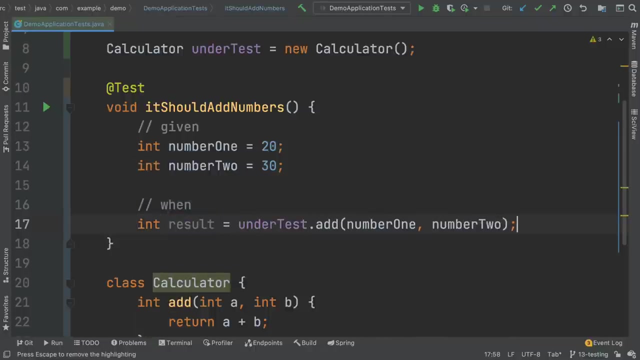 say when, and then when we say under test dot, add past the number one and number two, So this will give us an integer. So if I extract this to a variable and I'm going to name this as result, And then finally I'm going to have then and 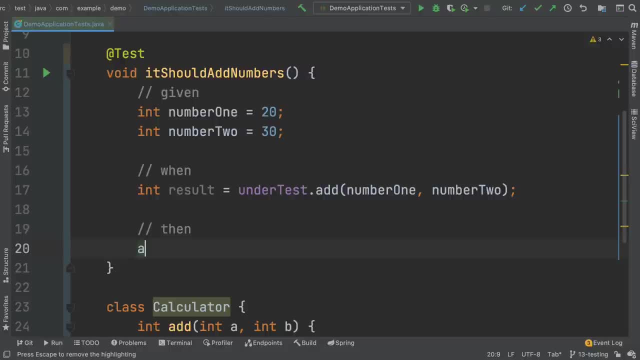 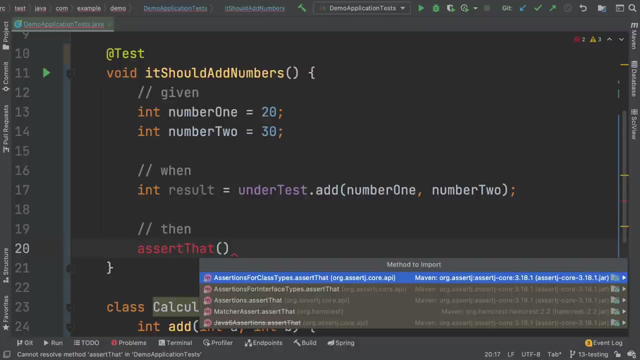 then here I could perform the assertion. So here I'm going to say assert and in that and here I'm going to basically import. So here import, static method, and then check this out. So we have a couple of imports, So you can see that we have org dot assert. 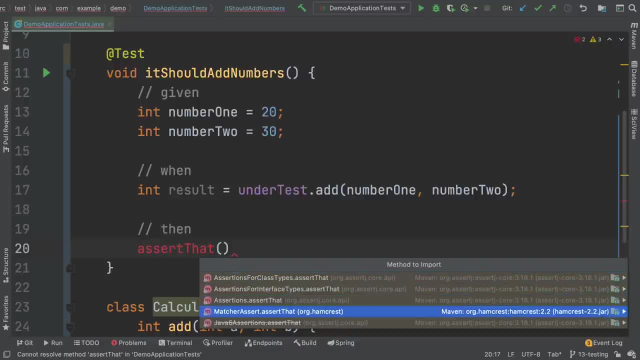 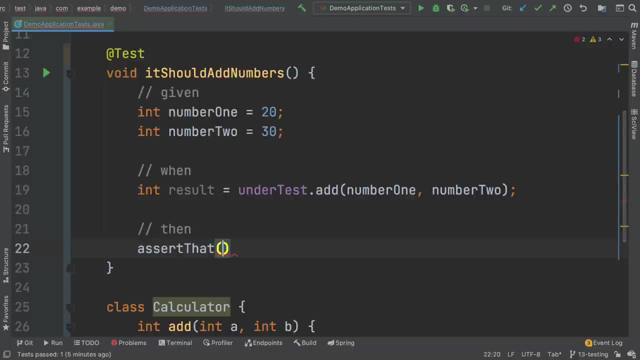 J core API. We also have Hamcrest and we also have this one, which is there Deprecated. So let's select the first one And then I'm going to say So here. basically, it takes D. You can see the actual. So assert that. 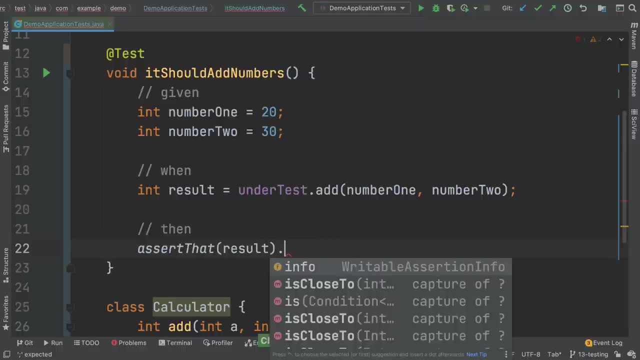 and then result dot and then is, and then equal to. if I press- or basically I don't have to press- command P, You can see that we have the expected value. So what I can do is say: right, So the expected value for me is actually 50,. right, Because 20 plus. 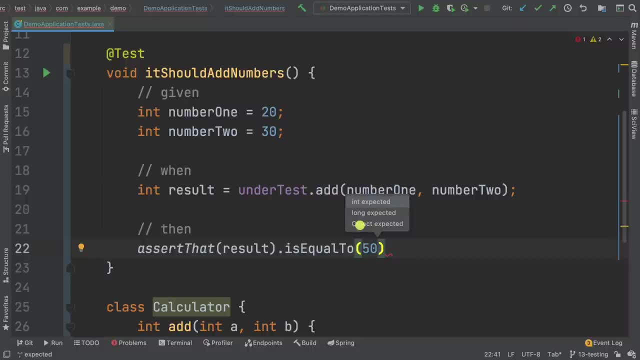 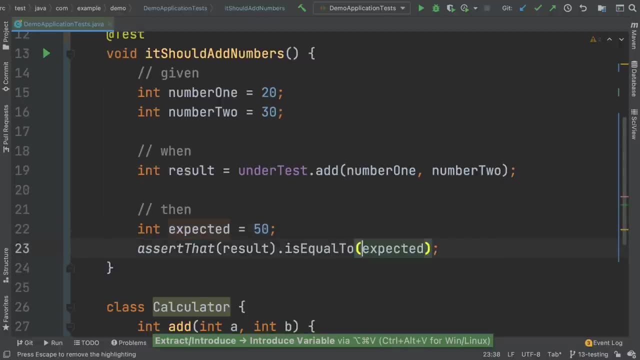 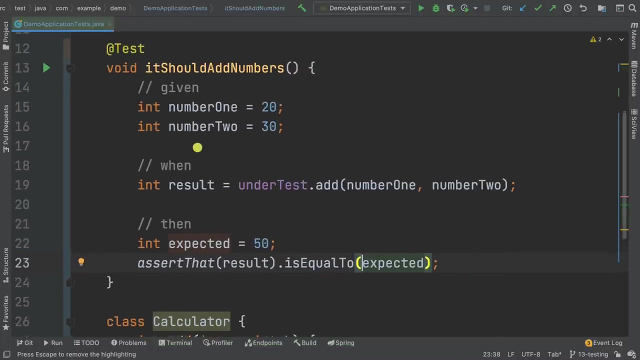 30 is 50, right? So here I can just end semi column and we can also take this to a variable and we can say expected. So it's really up to you whether you want to name things. And now this is our very simple test. 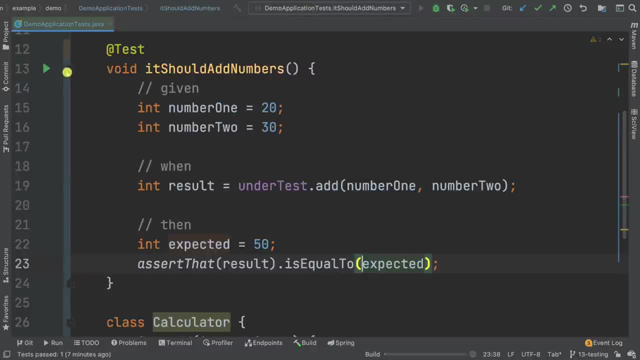 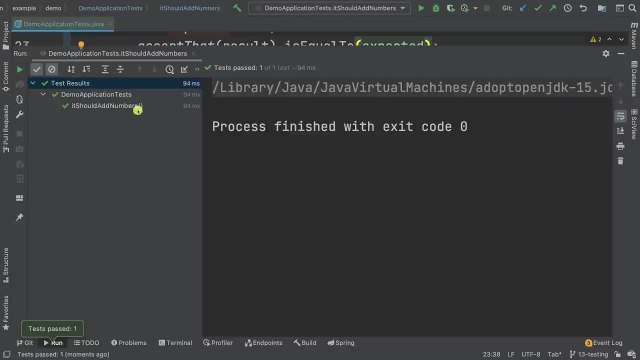 So let's just quickly run it And check this out So you see that the test passed. So here we have. it should add numbers, And maybe we should say it should add two numbers, Right? So let's just change it quickly. It should add: 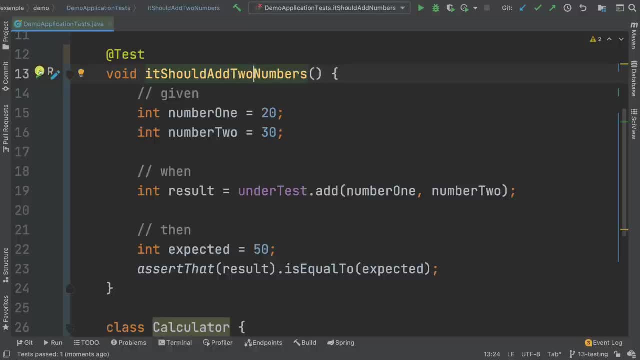 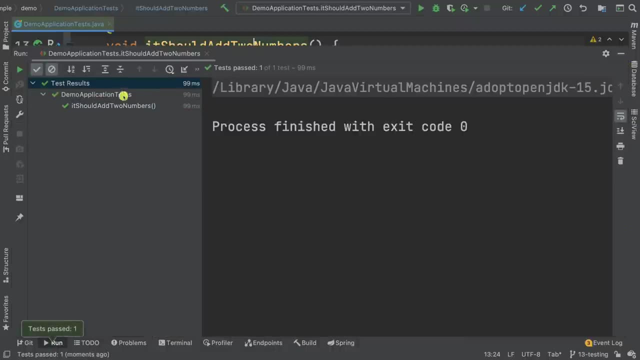 and then two numbers. Let's run it again And there we go. So this test passed Right, And this time it took a little bit longer, So 99 milliseconds, because we had some extra steps in it. Basically, this is a basic unit test using. 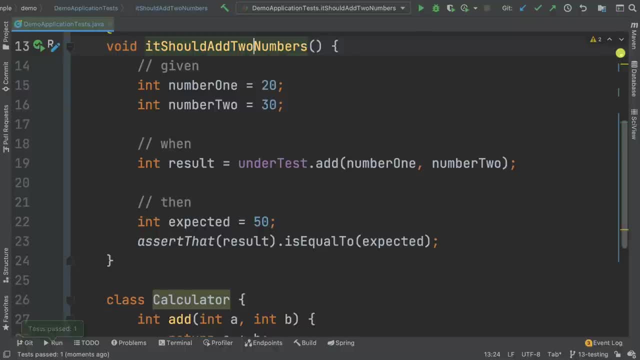 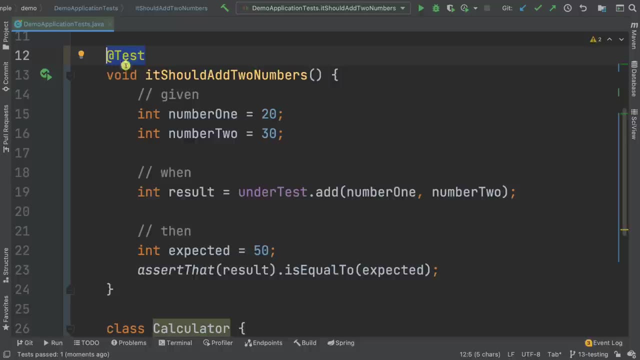 J unit and assert J. So let me just recap once more. So this annotation right here at test, this is J unit, right? So this tells that this method is a test method. And then we have basically in here I'm actually using BDD test style. So given 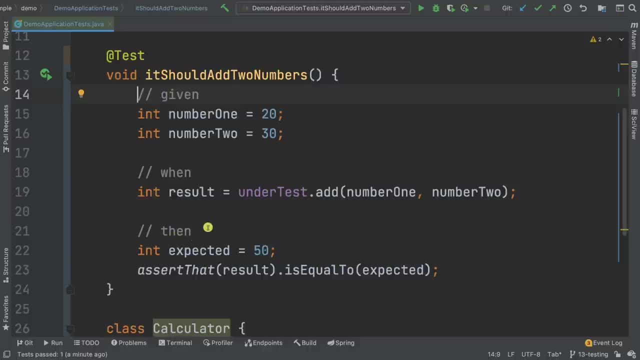 when and then then. So this makes it super easy for someone looking at the test and understand exactly what's going on. So, given So these are the inputs, And then when and the test with the method that you are trying to test is invoked- In our case, add when. 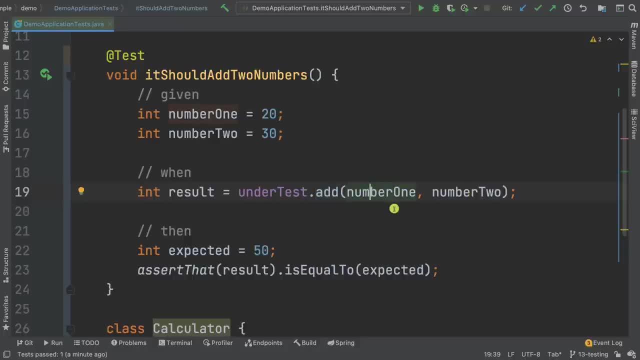 we pass the inputs number one and number two. we then say then, and then the expected, So we expect 50, and then we perform the assertion, So assert that the result is equal to expected. Now, if I also change this to 51,, for example: 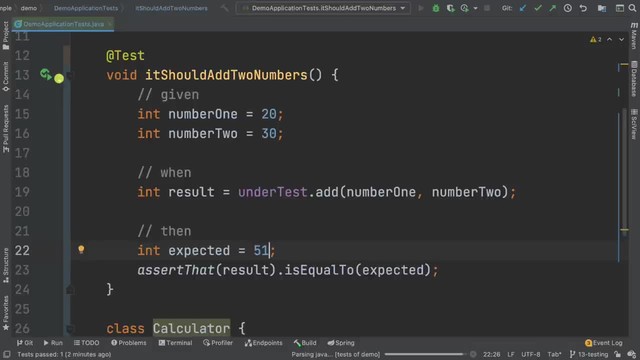 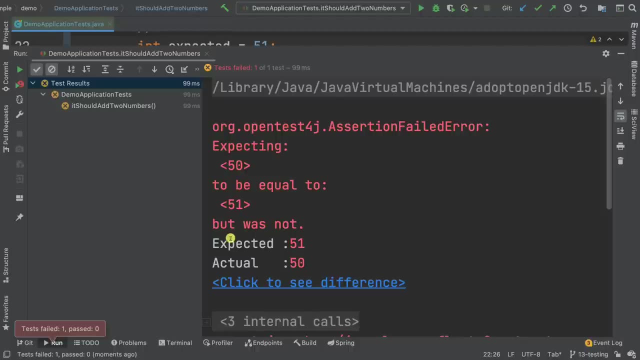 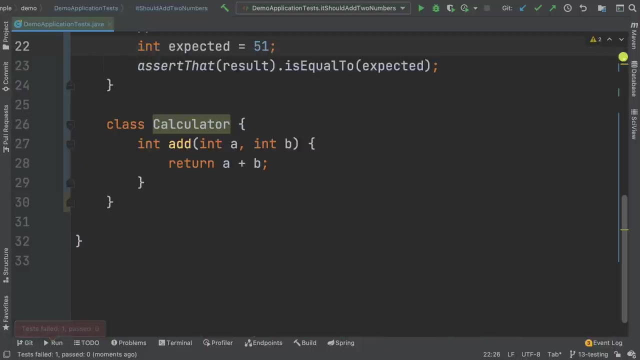 let's just run it again. There we go. You see that this failed and it says expected was 51. But the actual was 50. Right, So here, expecting 50 to be equal to, and then 51. So there we have it. Let me just collapse this. 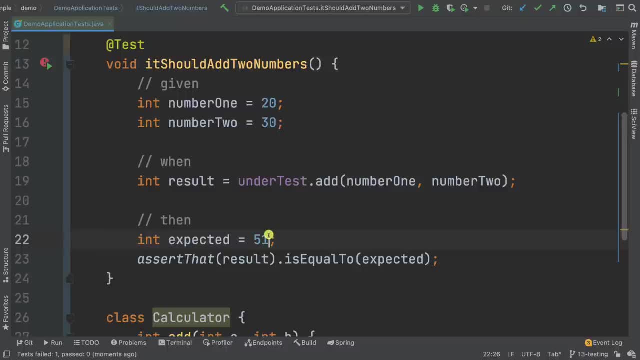 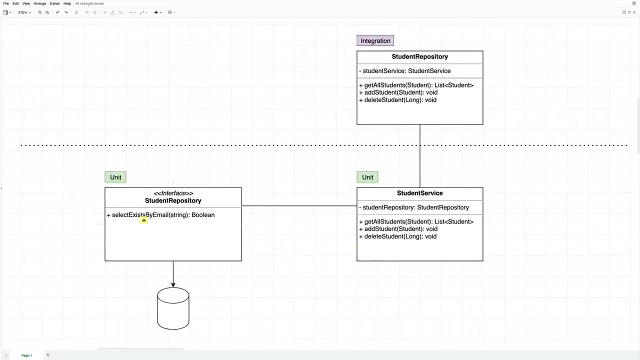 And you can see that this went red. And let me put this back to 50.. And there we go. So this is your very first J unit test, with one assertion. Next, let's go ahead and test this student repository interface right here, which is a little. 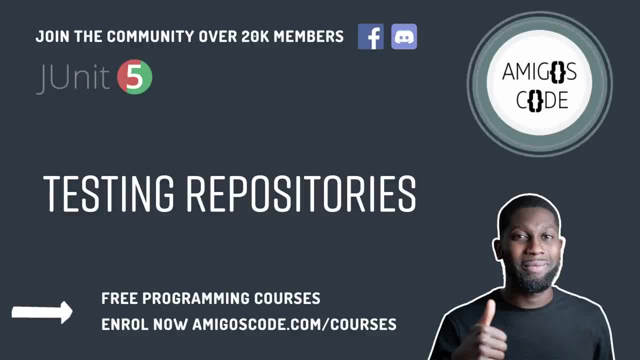 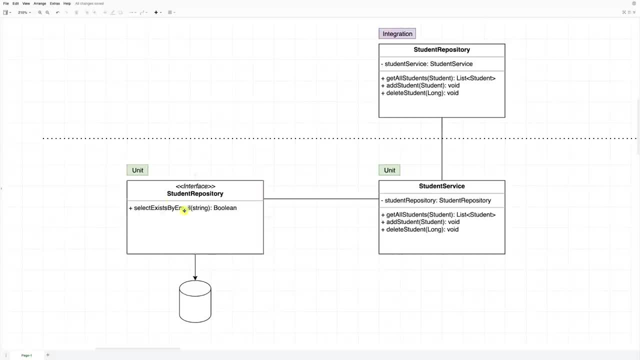 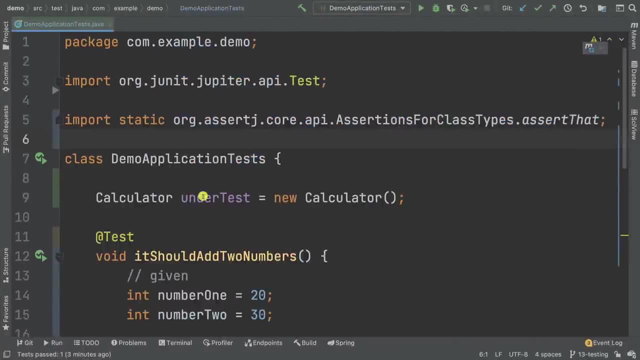 bit more interesting. Right, Let's go ahead and test this method right here: Select, buy and then email. So let's go back to IntelliJ, And in here I'm going to open up the project tab and then I'm going to navigate to Java. 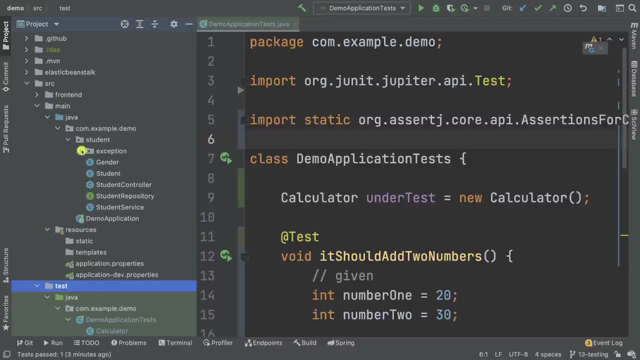 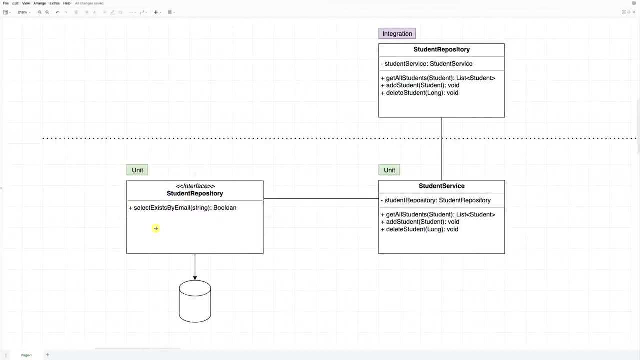 So main Java, And then inside of student, we have the student repository. And this repository, you can see it's an interface and is this interface that we want to test. So again, this talks to this database right here. So in our example. so you saw that we 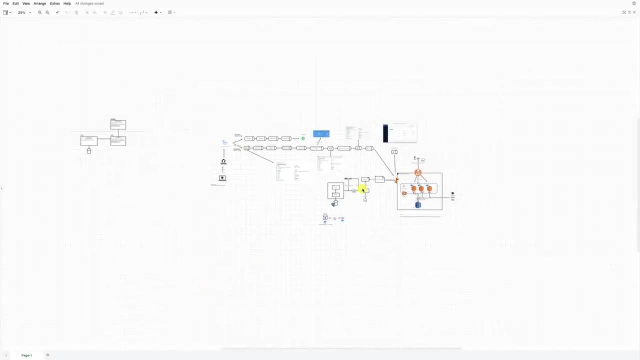 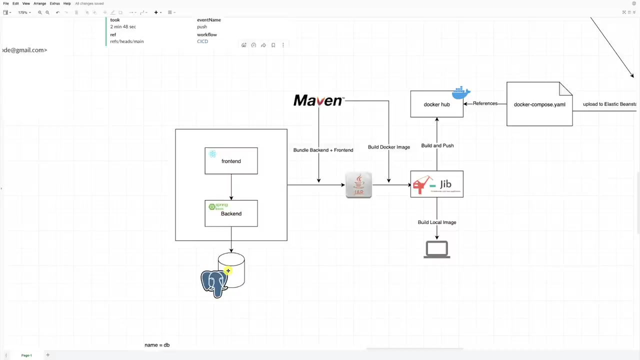 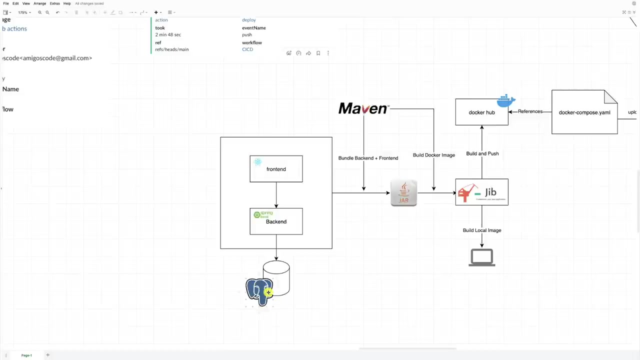 have. So if I just zoom out a little bit and then just zoom in here, you saw that we have a Postgres database running Right. So for testing purposes we're not going to use the Postgres instance that we have locally, And I'm going to show you a better way. 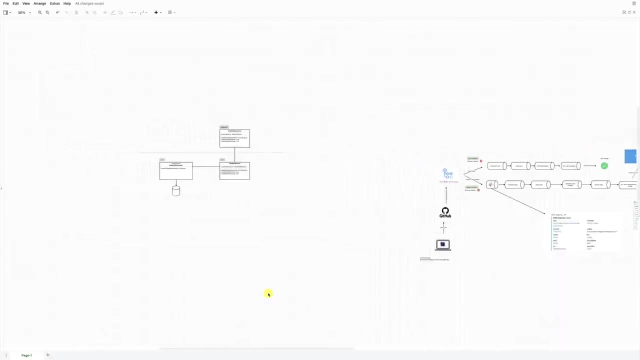 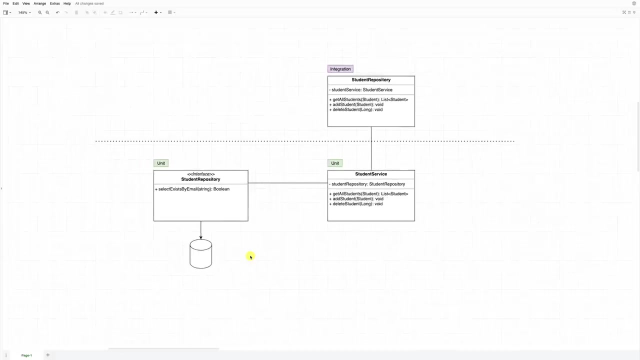 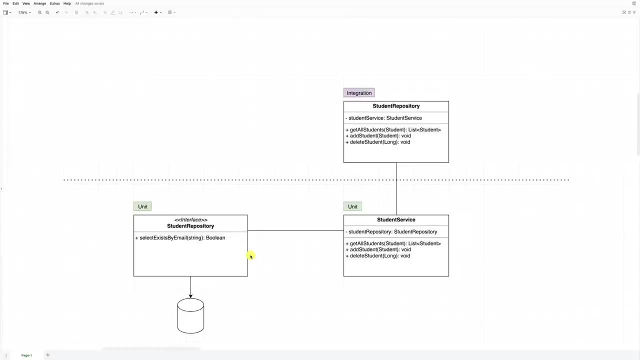 that we can do this. So let's just quickly go back to IntelliJ. And if I put this back just like that, it's kind of hard to zoom with the trackpad. There we go, So I think this is good for you. There we go. So in here, the way that we're going to create tests. 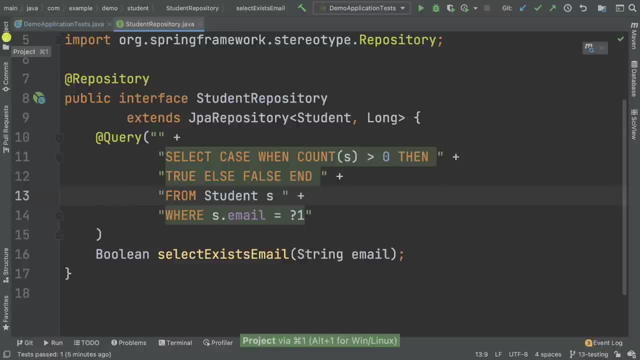 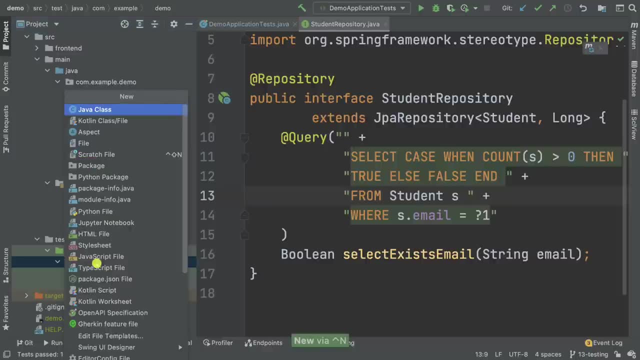 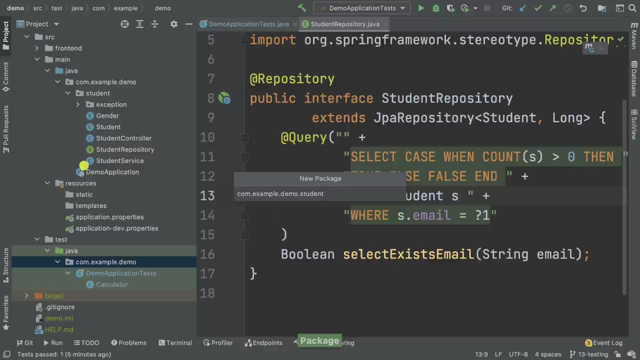 for this is: you saw that if I open a project, you saw that we can basically in here we can say right, So we can write, Oh, actually, we can right click, and then we can create a new package. We can say student, And then inside of student, 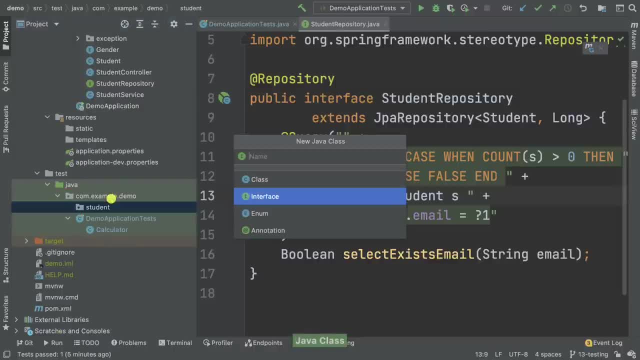 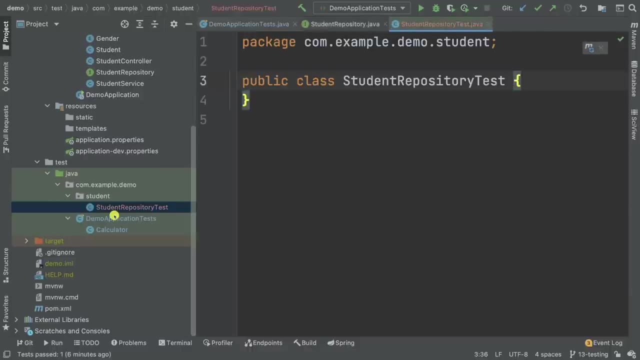 then we can say student and then have a new interface And this will be actually a new class, And then this will be a student, And then repository and then test, just like that: Enter, And then we can go and basically write a test, Right? So you saw that this was a bit manual. 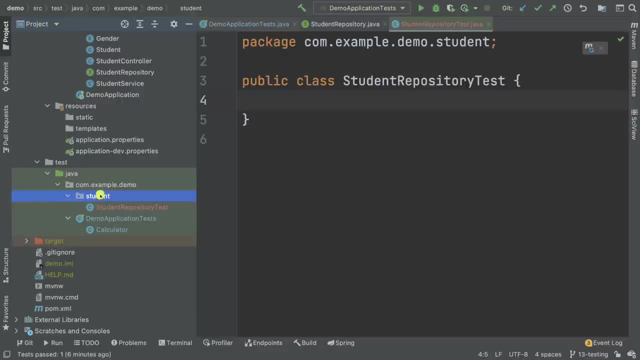 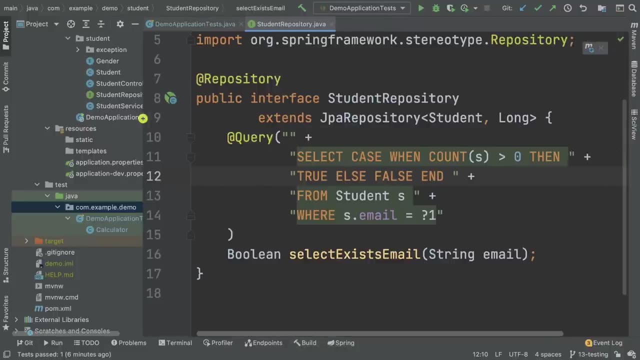 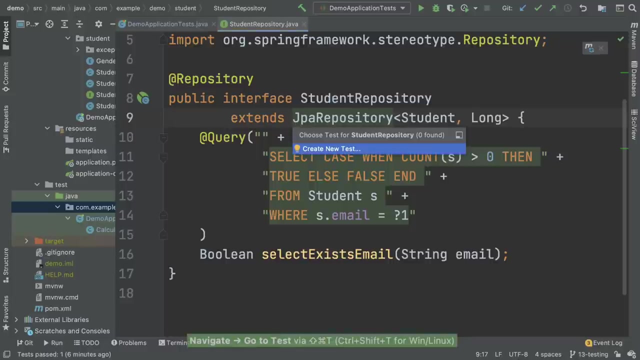 So let me actually delete this package inside of the test folder, And I'm going to show you a better way of doing this. So in here, inside of this interface, go ahead and press shift command and T, or shift control and then T. if you are on Windows And right here you can see that. 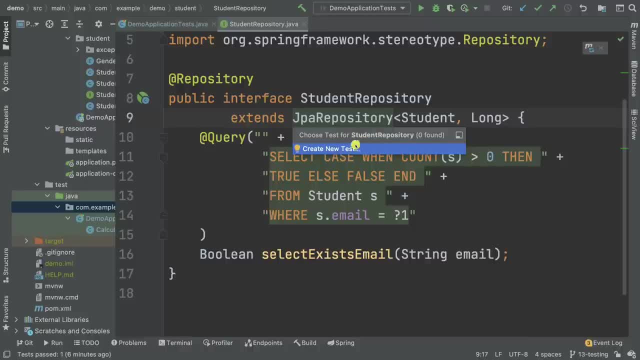 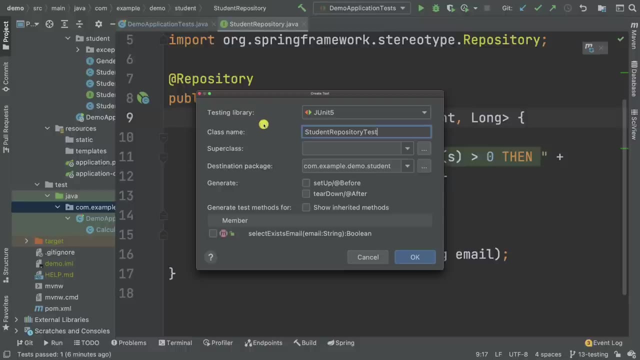 we have choose new test for repository. So zero found. And that means if you have a test it will just navigate into the test class. But here what we want to do is create a new test. So create test And then you can see that this is prepopulated. So testing library. 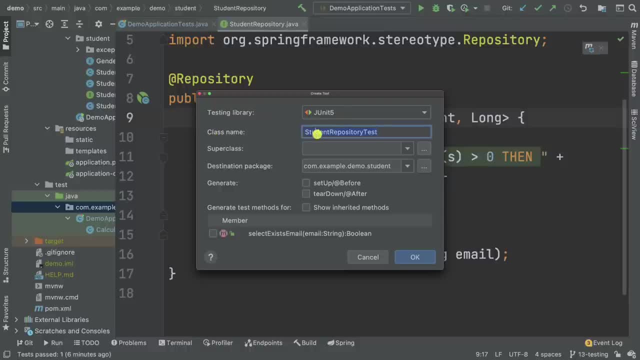 J unit class name. So basically this is the same class that we had just a minute ago, And then for the subclass, we're just going to leave it as is. And then destination package: You can see that this follows the same package as the one. 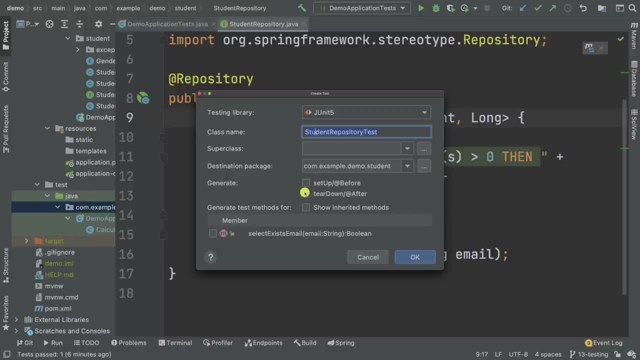 you have in main Right And then we can set up the. basically we can have the set up method and tear down so on and so forth, And right here you can see that generate test for methods and then member So select and then exists email. So let's just take this. 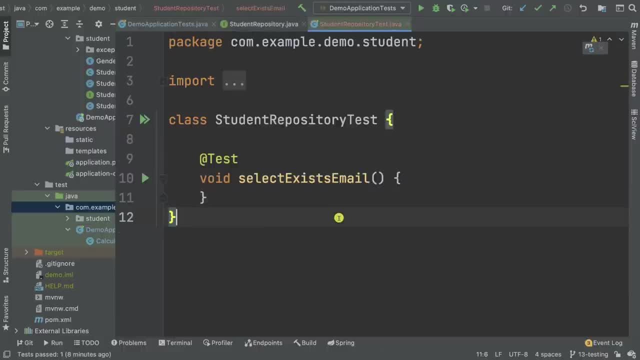 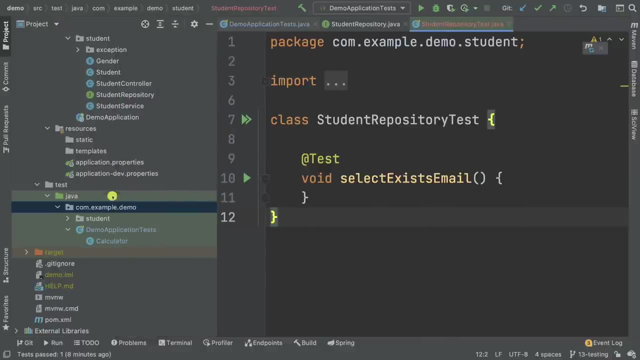 and okay, There we go. So you see that we have a test class. So this was some auto generating for us And you can see that basically we have the exact same thing here. Expand, You can see that we have repository, and then test. 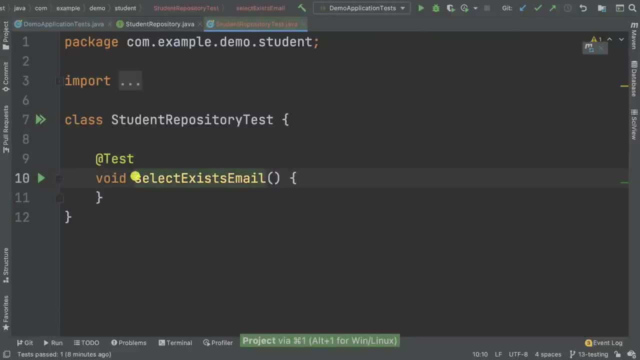 So now we can write our test. So here let me just say it, and then should, and then select, and then exists by email, And I think we should have a better name here. So it should select, it should check if, and then student, and then exists by email And basically the name here doesn't really. 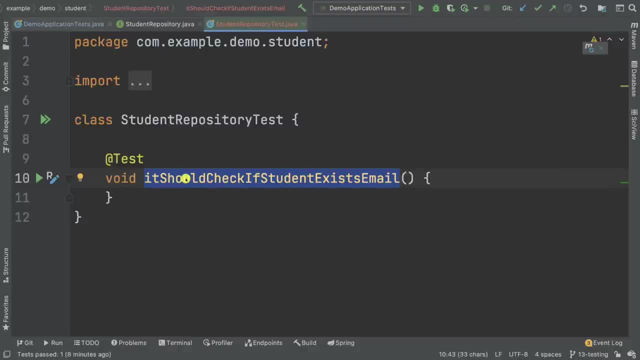 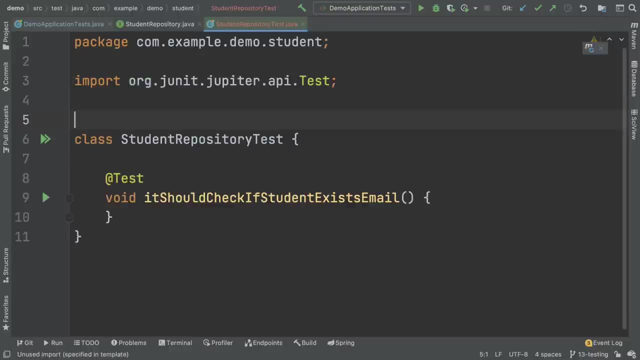 matter. You can go as long as you want, but as long as it makes sense, that's what matters. So in here now, what we're going to do is: so let me just remove this import, because we're not using assertions from the unit, And here let's just say that we want. 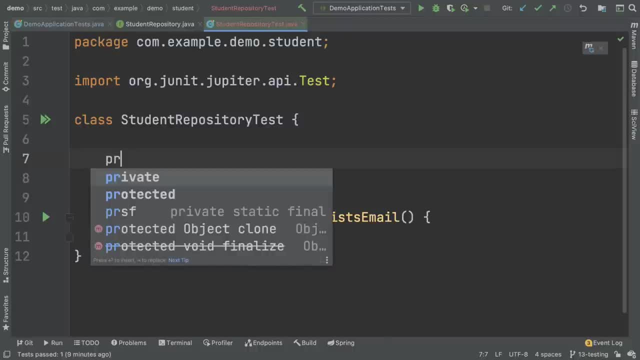 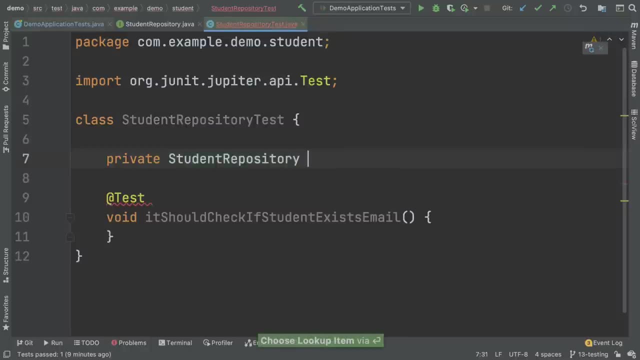 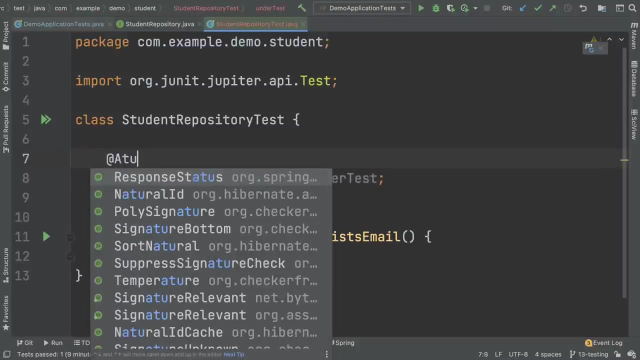 to. basically we want to auto wire So private, and then say student, and then repository, And here I'm going to say: and the test, and then end this with semicolon, And in here I'm going to auto wire, So here I'm going to say at, and then auto. 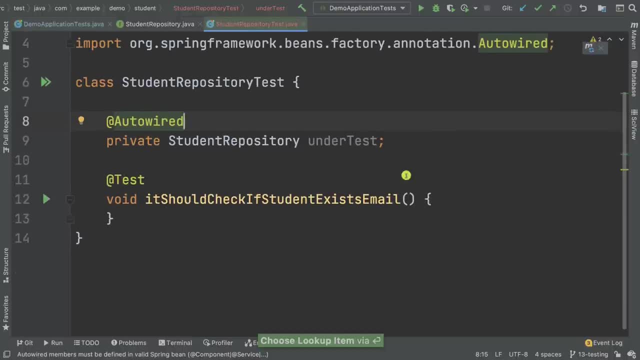 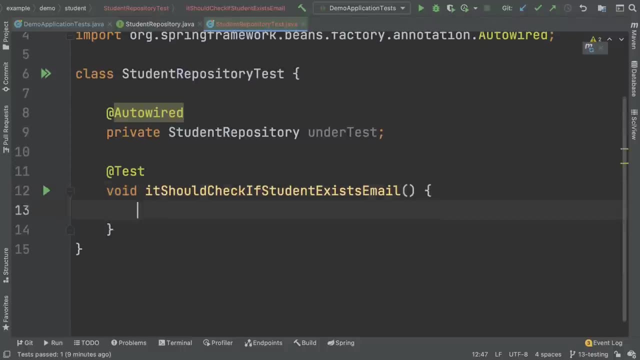 wired, And you'll see this in a second. And now what we can do is basically set up the given wire When and then then. So here let's go ahead and say that given and then when, and then then- and I'm missing an N in there. 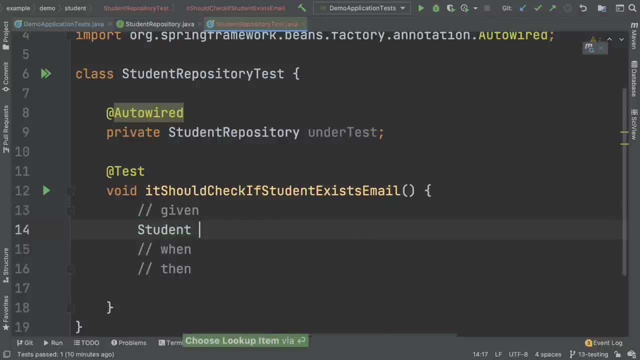 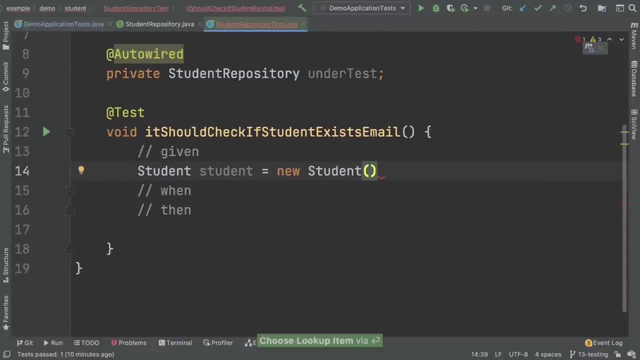 So given a student, So let's say student and then equals to new, and then student, And then inside I want to have. So basically let's just have name. So I'm going to say Jamila and then email will be Jamila at Gmail. 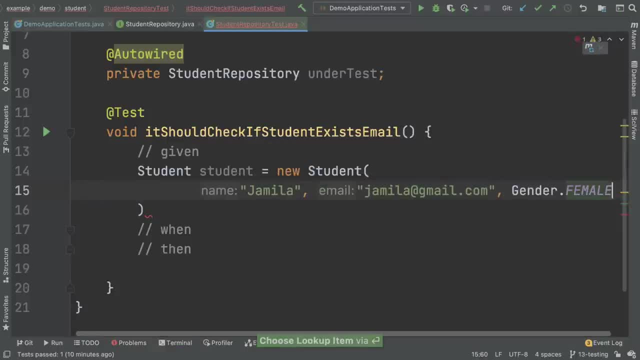 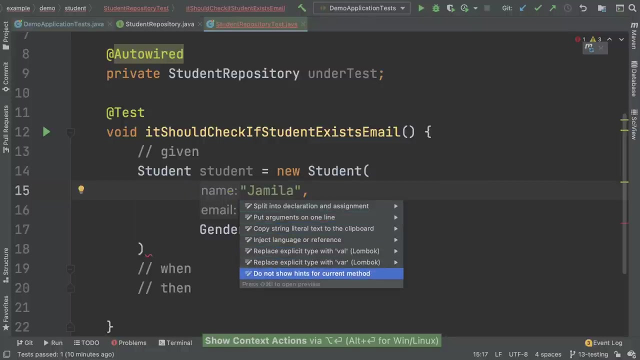 dot com and then gender. And let me put this on a new line. There we go Just like that, And, by the way, do not type name and then column, and then email and then column. So this is intelligent. given me hints. So here, if I say, do not, 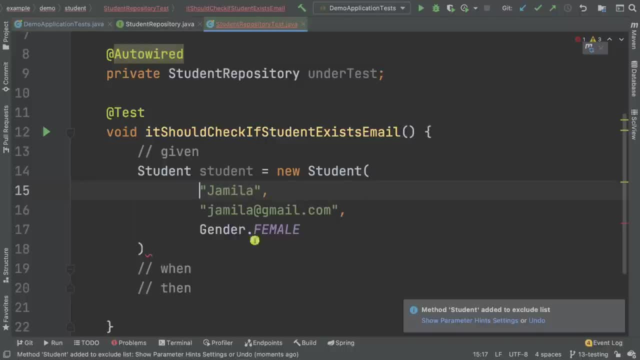 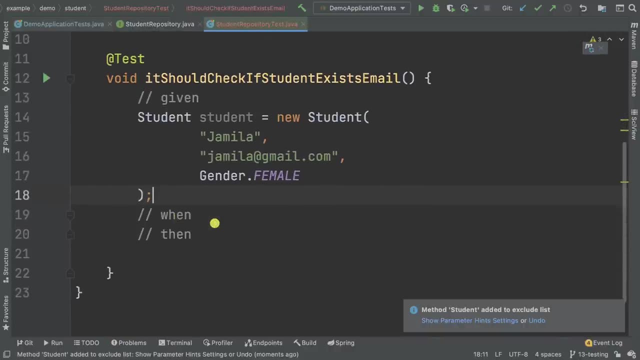 show and then hints for current method, You can see that that goes away Right. So here, if I press semicolon there, So we have a student And what I want to do is so given. So here I want to say: under test, dot and then save. 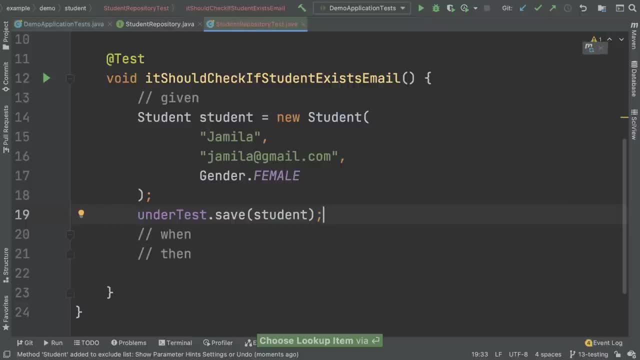 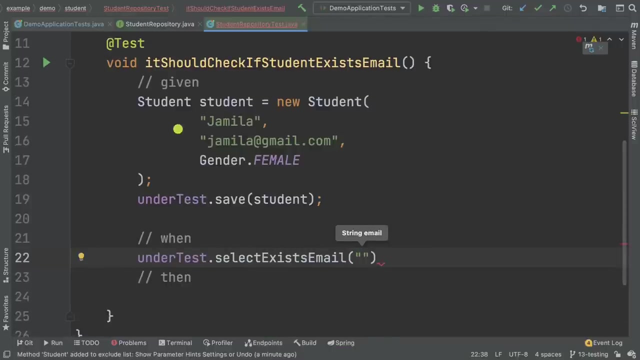 the student. And then I want to say when. and then under test dot and then select, exists email. In here let's just pass an email. So here I'm going to say, let's just extract this to a variable as well. So email. 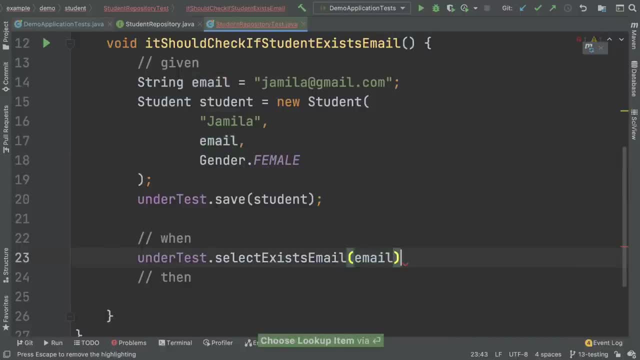 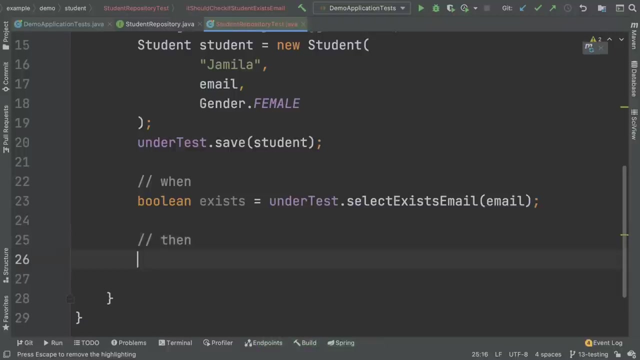 And then here I'm going to say email, And then this returns a Boolean Right, So exists. There we go, And this can be lowercase Boolean, And then so in here, then I want to say assert, And then that, And if I press option and then enter, or you can click. 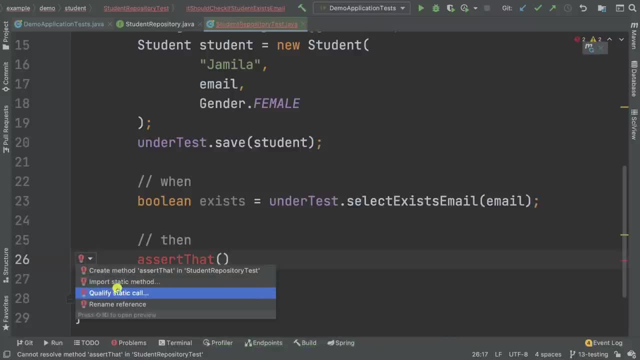 on this bulb right here and then import static method and make sure it is the one from Sir J Core, API, And then I'm going to say exists, And then dot is, and then true, just like that. And you can name this too, Expected, for example. So if you want, so expected. 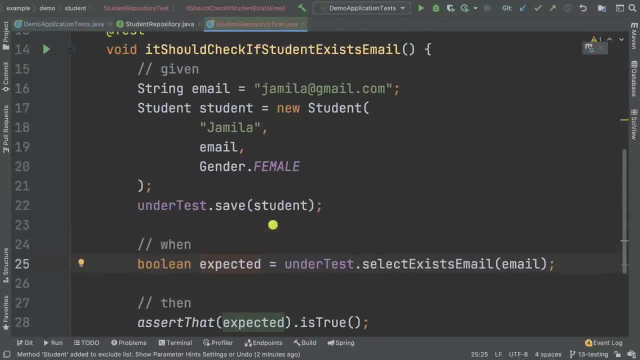 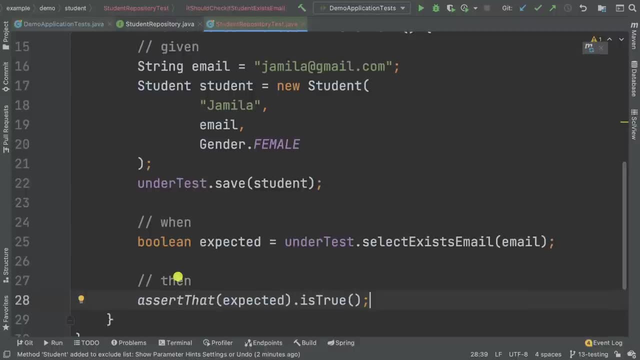 there we go And this is our test. So you can see that it's really straightforward, Right? So, as you have the given when and then, then it's very easy for you to set up your tests. So, given a student Right. 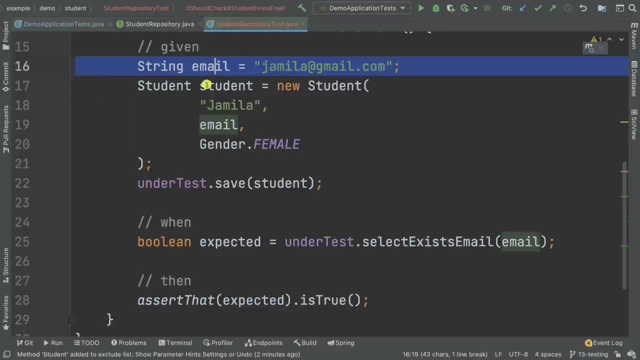 So here we're doing all the prep work, So we have an email, the student- we save the students. So all of this is part of the given. And then, when we invoke the under test- and this is the method that we are testing- then 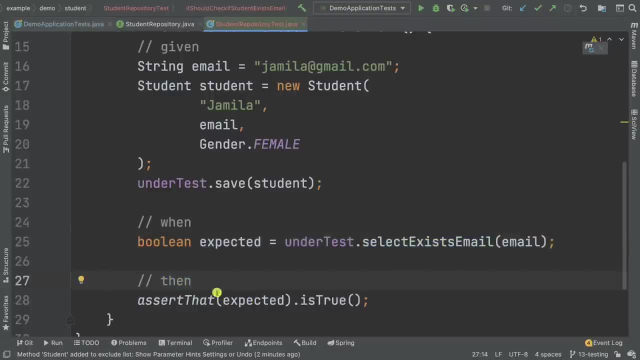 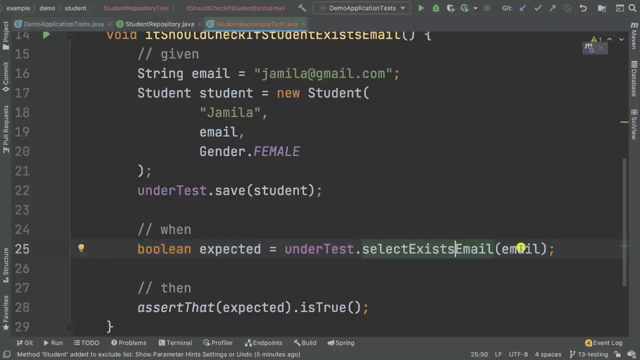 the assertion is. so we say: assert that expected is true. Right, Because we know that this method should return. true, because this email is already owned by Jamila. So before we actually run this test, there is something that we should configure, because we don't. 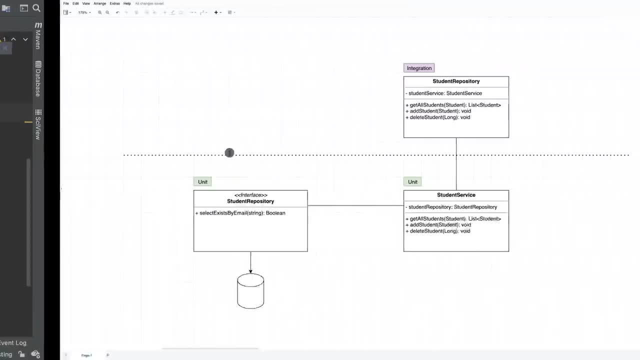 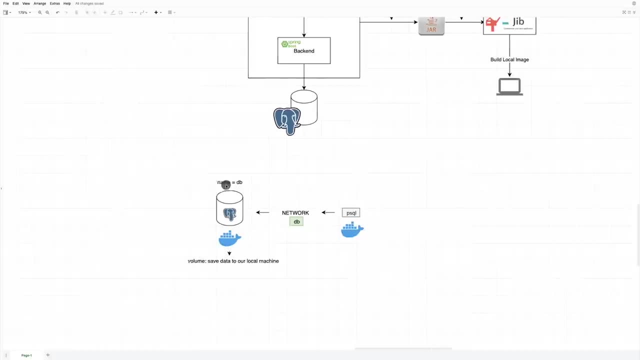 want this test to run against our database, right here. So remember I said so in here we have. So where is it So in here, Right? So we don't want the unit test to run against our Postgres instance, but instead we want this. 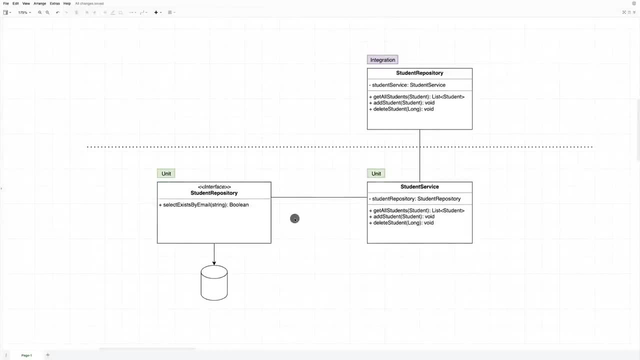 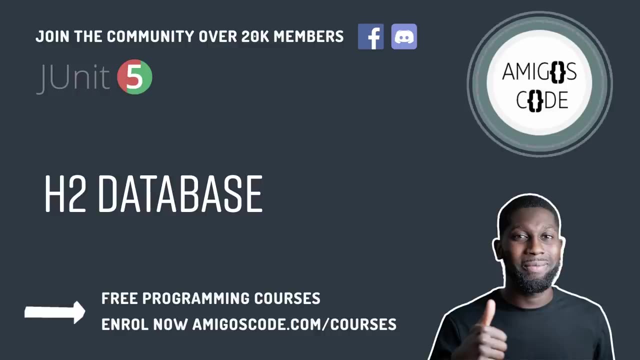 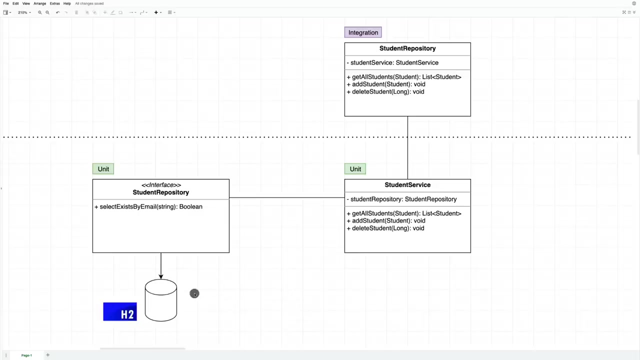 to run against an H two database, which is an in memory database. Next, let's go ahead and configure this in memory database, Right? So, as I said, we want to run our unit tests for this student repository against an in memory database. We don't want to run the. 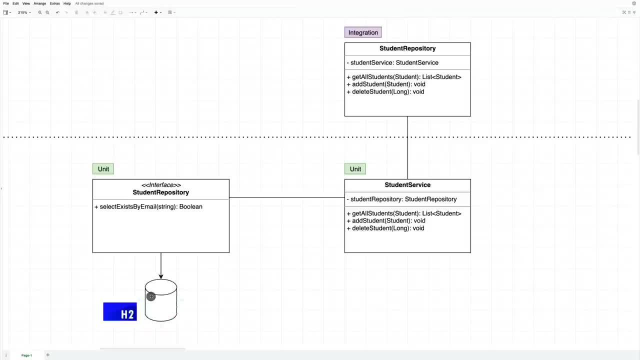 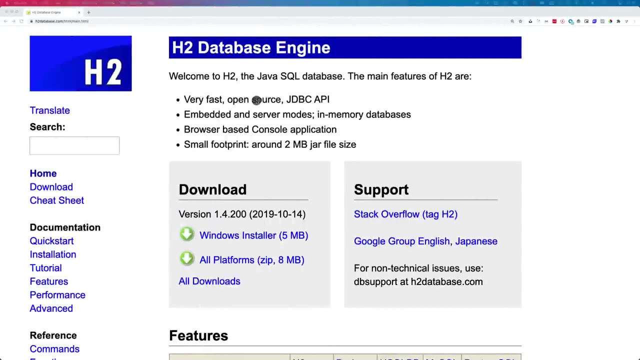 tests against our local database, because the data produced by these unit tests we don't want to keep them in our database And luckily for us we have this database called H two, And H two is an open source SQL database and you can use it as. 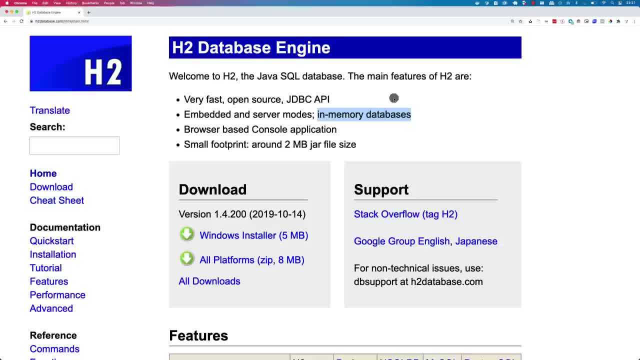 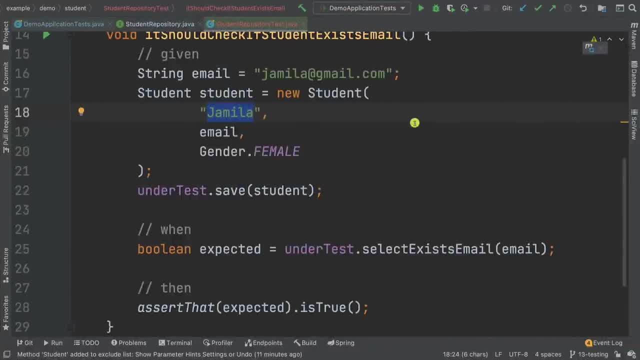 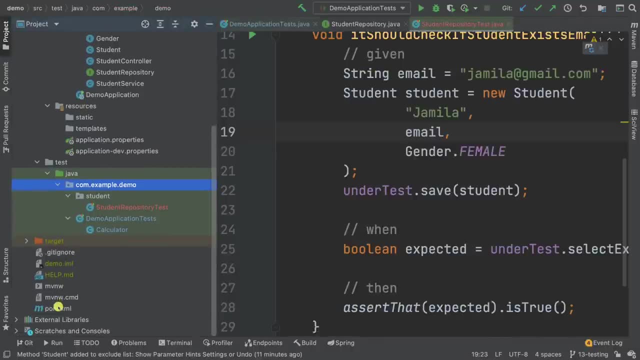 an in memory database. So to set up this in our application, to use it for testing, it's really straightforward. So if I open up IntelliJ and in here open a project and then go to Palm dot XML And what we're going to do is the following: 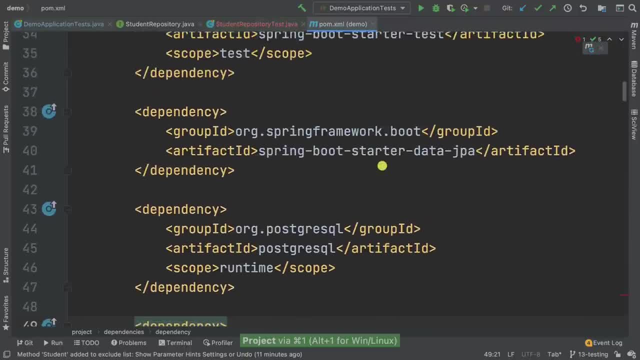 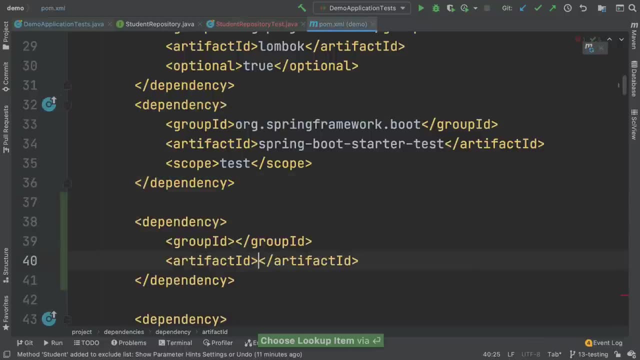 In here. it doesn't really matter where we add this, but let's just see, right after the spring boot starter test, let's add a new dependency. So dependency: this will be H two and then the group ID will be calm dot and an H two. 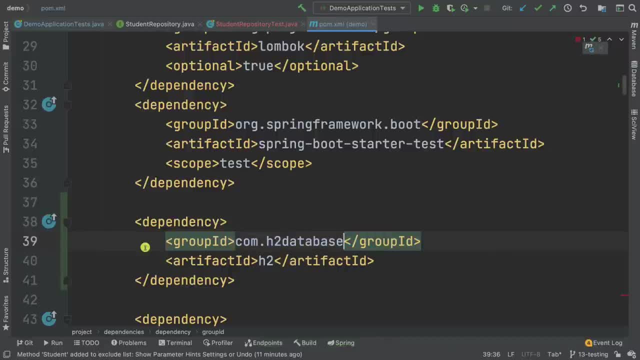 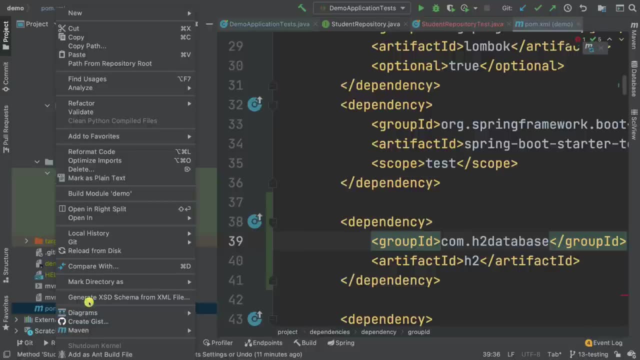 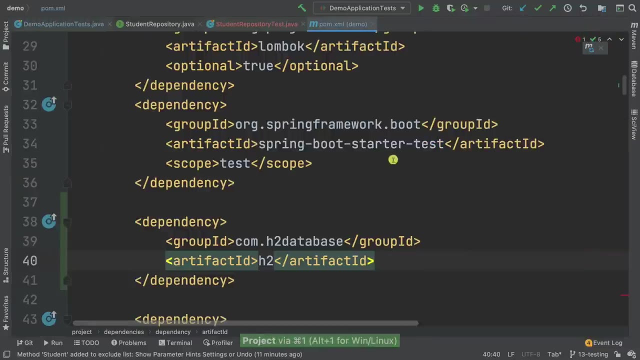 database. Now, if this is right for you, what I want you to do is just go to project and then open up Palm dot XML right click and then, actually, before we do that, let's also set the scope for this, as they have done in here. 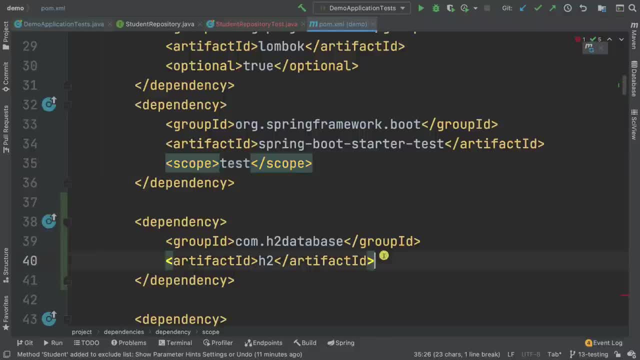 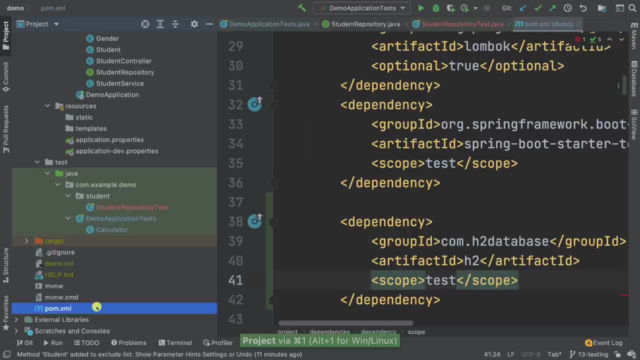 So the scope for this right here is test. Let's also do the same here. So scope and then test. Now open up the Palm dot XML, right click and then go to Maven and then reload project, And that should sort this dependency out. So now that we have this dependency, 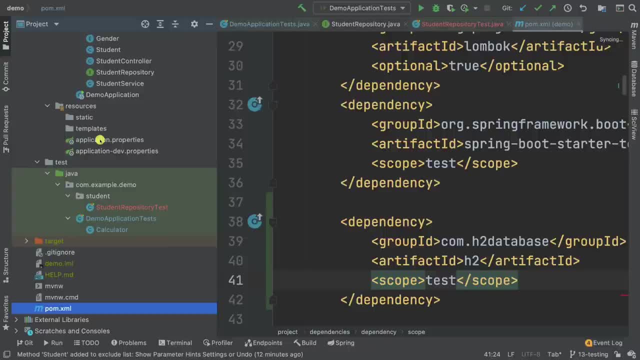 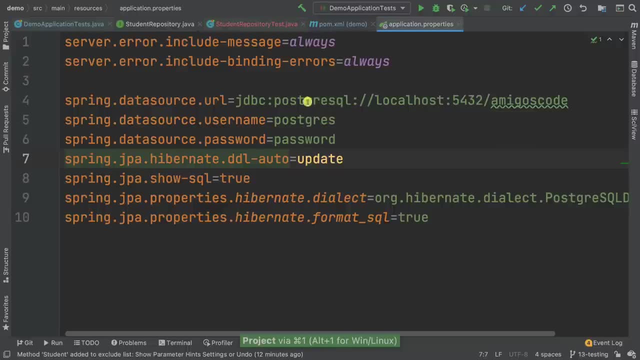 what we need to do is to remember, in here we have application dot properties, So application dot properties, And this in here connects to our local database, right? So our Postgres instance. So what we're going to do is the following: We're going to, so we're going to create: 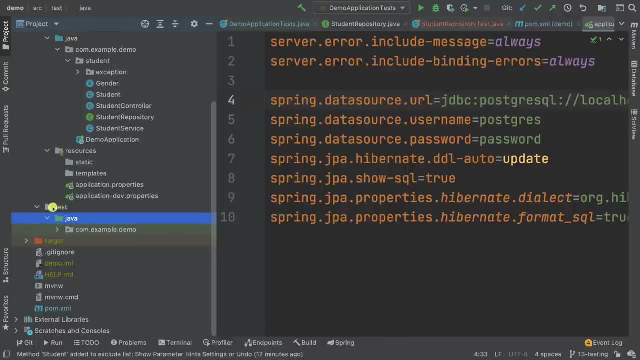 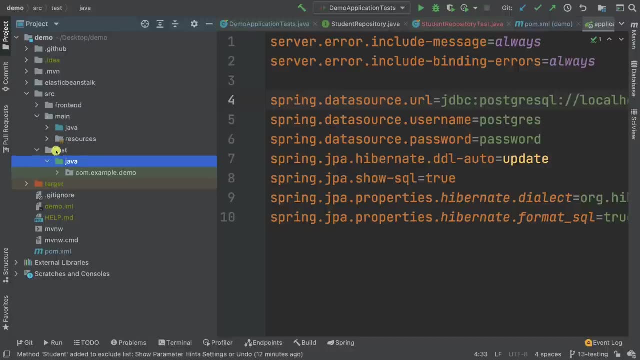 a new folder under Java, So test, and then Java, And we want the exact same thing right in here. So main Java resources, test Java, And we also want resources. So I'm going to right click And then in here, if I say new and then directory, I can pick. 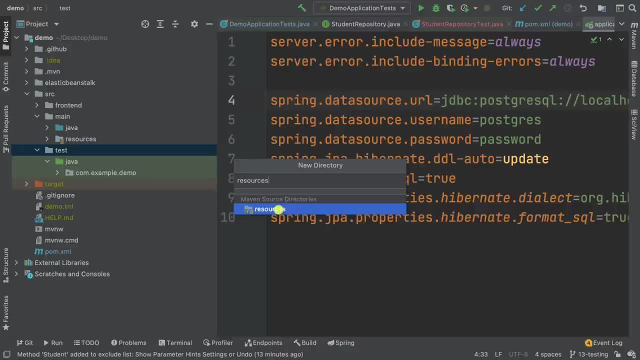 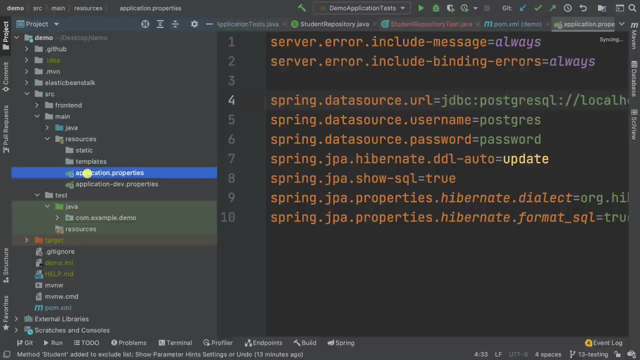 this Maven source directories. So pick that And there you go. Now take this application dot properties in here, Command C, and then put it inside and then okay, Now this application dot properties is used for testing, And what we can do now is basically in here. we can 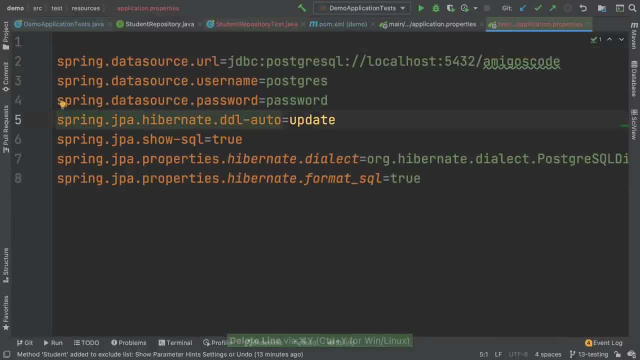 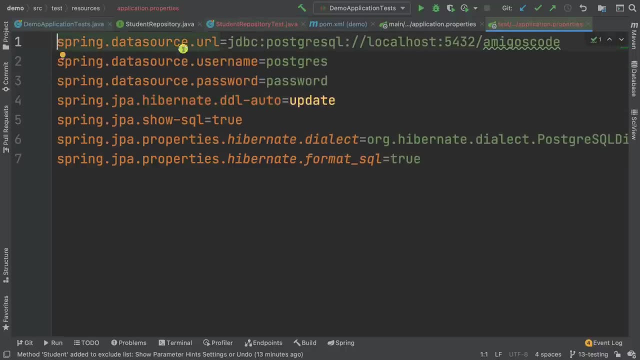 remove all of this. So let's remove that. Basically, we can actually keep all of these, But one thing that I want to change is so in here the data source URL as well as the username and password. So the URL instead of Postgres. this will be. 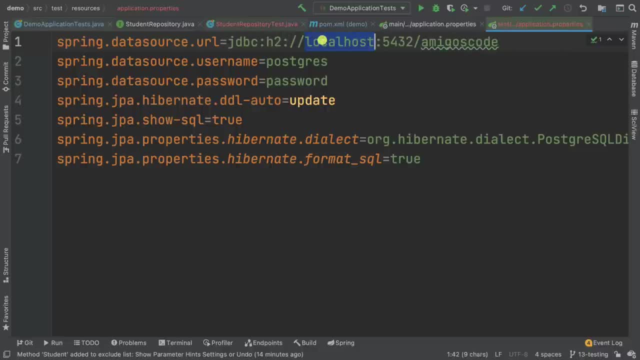 H two. And then here we want an in memory database. So say Mem and then DB and then and then semicolon and then DB and then underscore and then close, and the score delay equals two and then minus one. So this is some configuration that we can add for our in memory database. 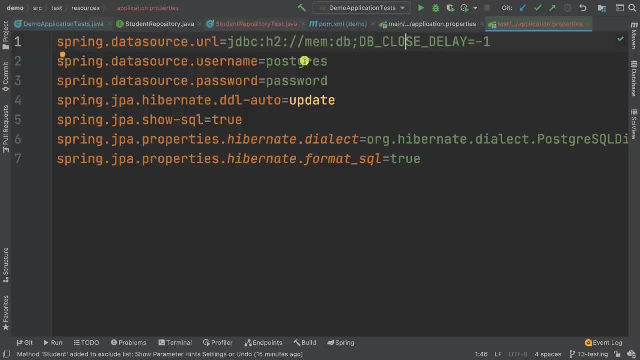 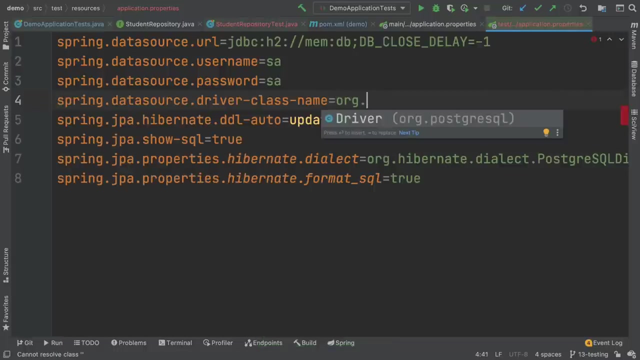 And this should be close just like that. Then, for the username, we want this to be SA and then password as well as a, And also, what I want to set is the driver and then class name, And this will be org dot and then H, two dot and then a driver. 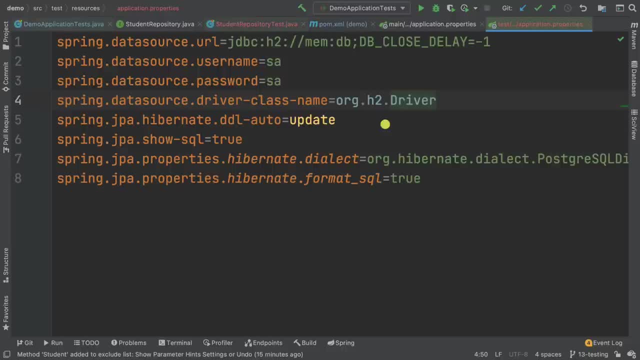 just like that, And this is pretty much everything that we want. And in here, instead of say update, let's say create, drop. So basically, we want to have a fresh database every time we run the tests. Now let's go back to our student repository test. 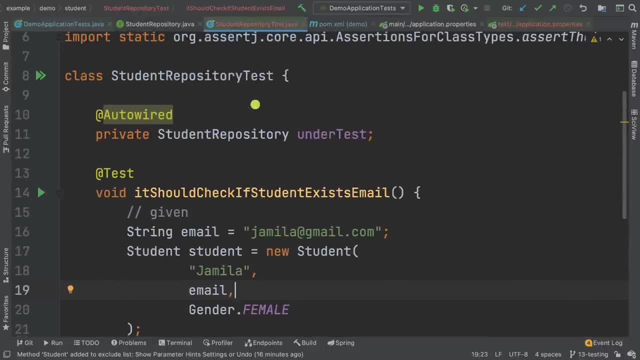 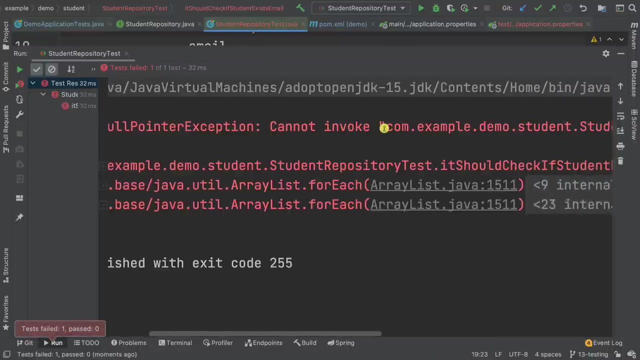 and let's actually just try and run to see if things will work. But I can tell you that it's not going to work, And this is because we need a special annotation. So here let's just try and run the test class And there we go. So you see that we have a no pointer exception. 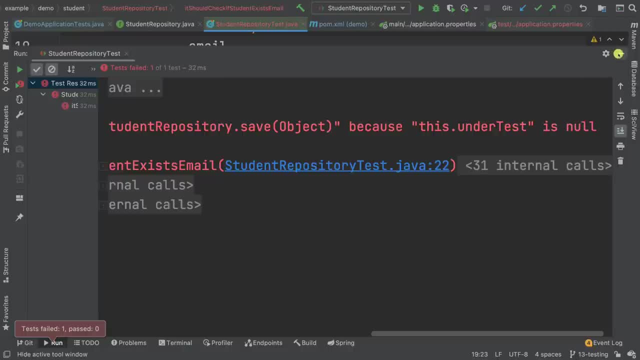 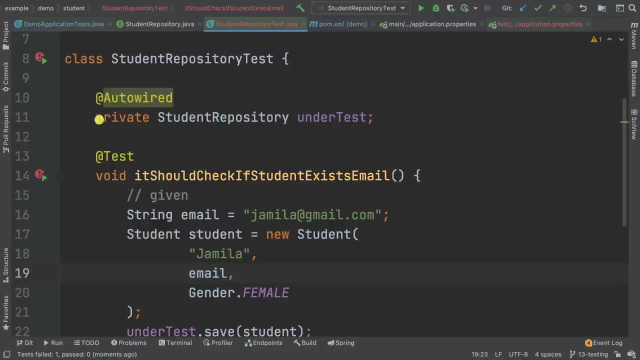 And it says that under test is no. So this is correct And that is because we are missing an annotation that will basically wire up everything. So, basically, it will start the application, It will connect, It will get a data source from the configuration that we have. 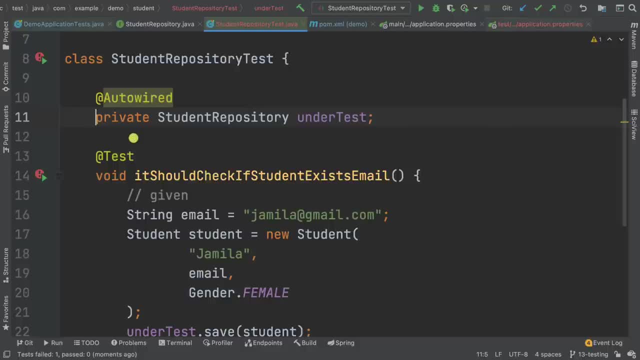 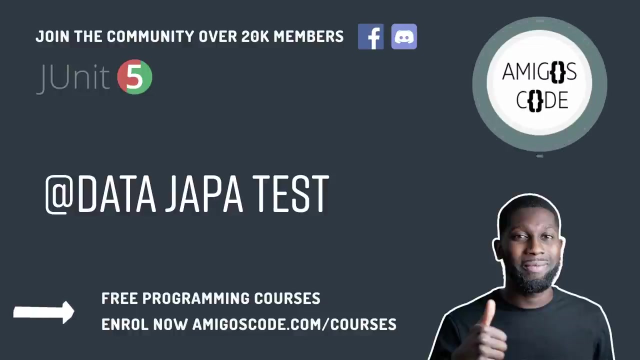 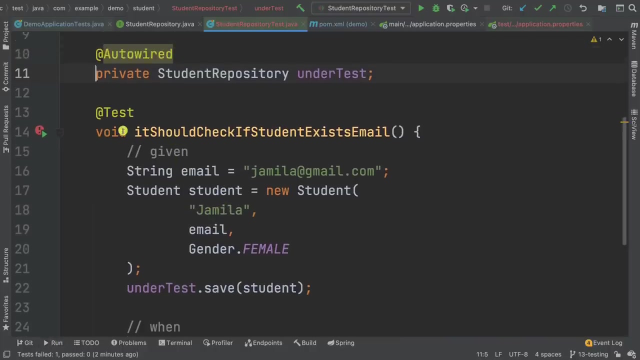 And then we're going to auto wire things. So there we go, Now that we have H two configured. next let's go ahead and get this test class running and then also add a second test Right? You saw that this test, when we tried to run it, it did fail. 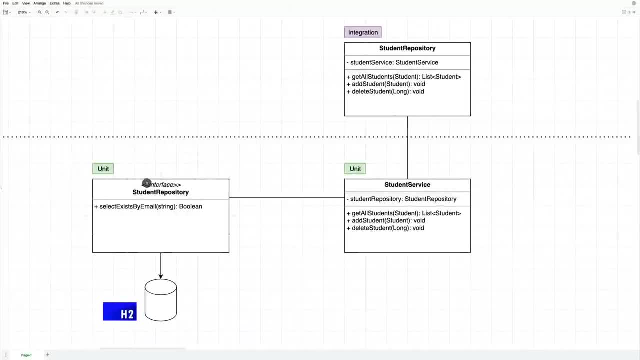 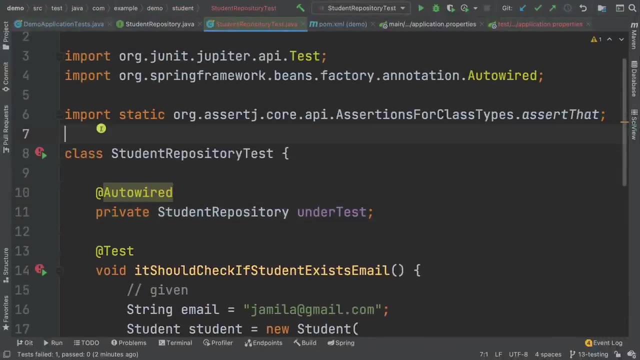 And that's because in here this test- So we have a test for this interface- needs to connect to the H two database. Now, anytime that you are unit testing your repositories, you need to use this annotation right here. So I'm going to say: 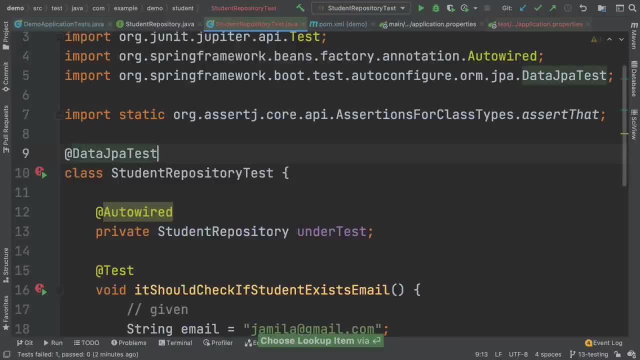 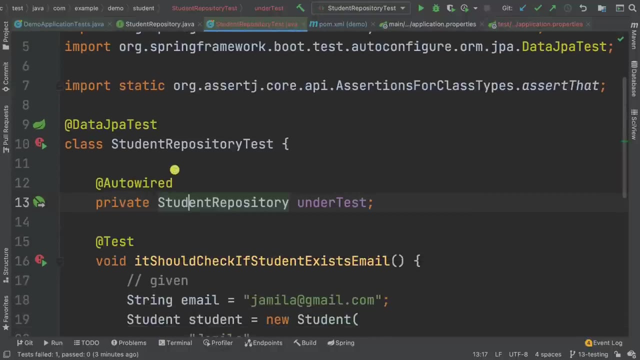 add and then data JPA test, And this is the magic that will glue up everything, including auto wire, the student repository And you can see that the error went away, and also spin up the database for us. So let's actually just for a second. let me just put a break point in here and 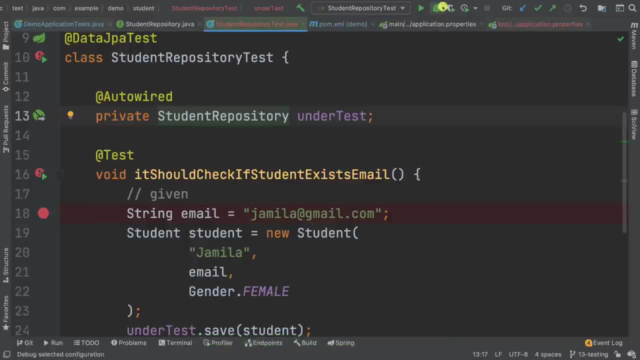 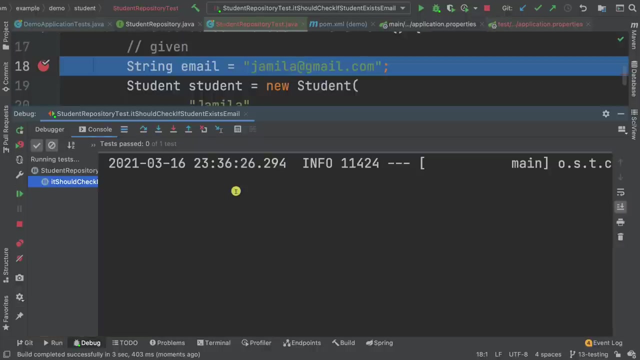 I'm going to debug this so we can debug, or I can just right click on the method and then debug And now check this out. This is familiar, right? So you can see that if I go to log again. so I just want. 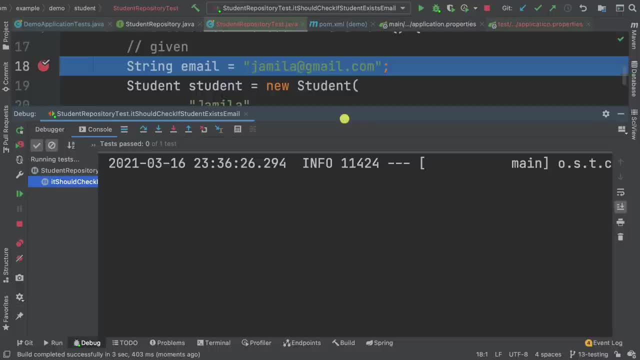 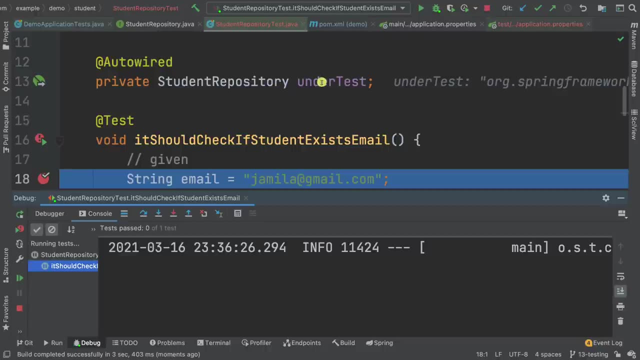 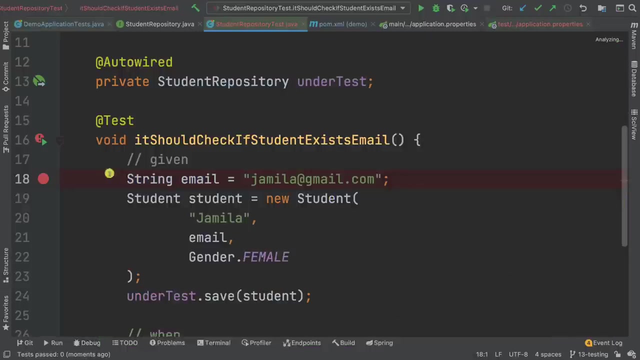 to see that it actually connected to the database, And in here this is actually paused. But if I inspect the under test right here, you can see that this is a JDK dynamic proxy and we can use it. So let me just stop this for a second. And then here let me collapse this. 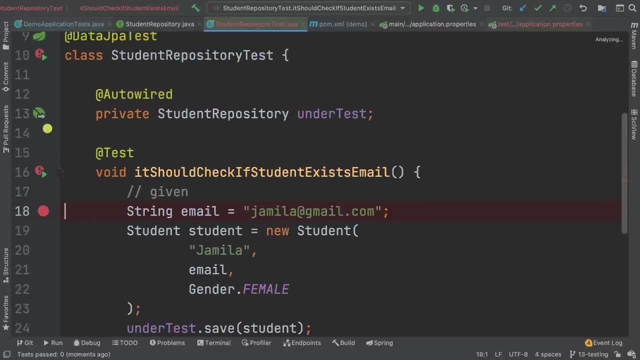 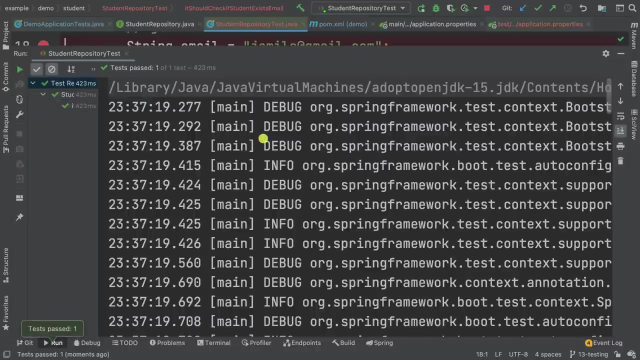 Now remember before this failed. So let's run the test Again. So I'm going to click on the class and then run student repository test And you can see that we have the familiar logging and check this out. So let's have a look at the logs So you can see that we 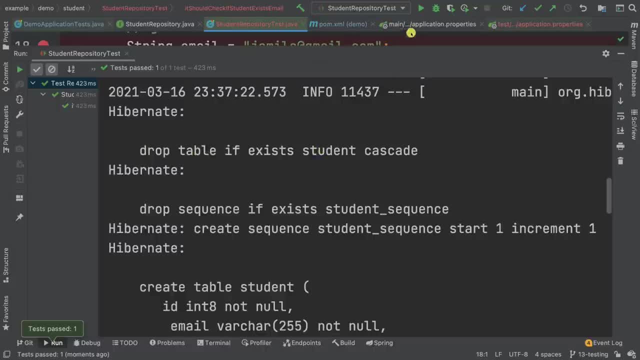 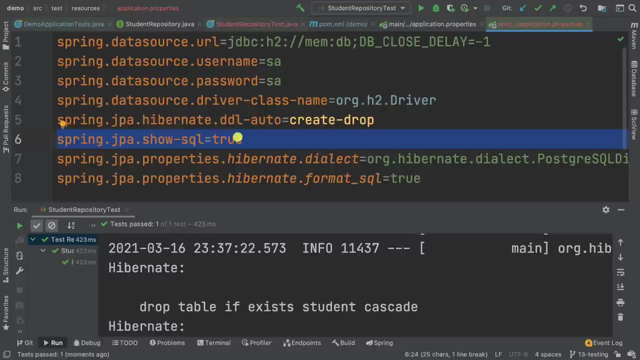 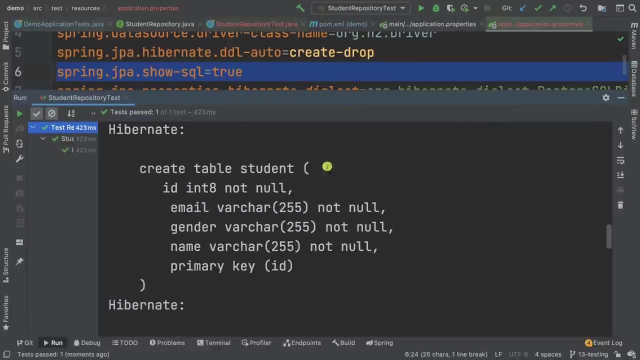 have some logging, create table, if exists. So this is because of this logging right here. This one show SQL And, to be honest, if you want you can get rid of those because it's just noise on the console, But for testing it's absolutely fine And you can see that we. 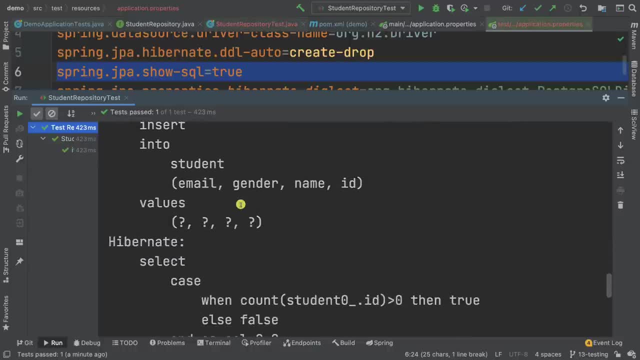 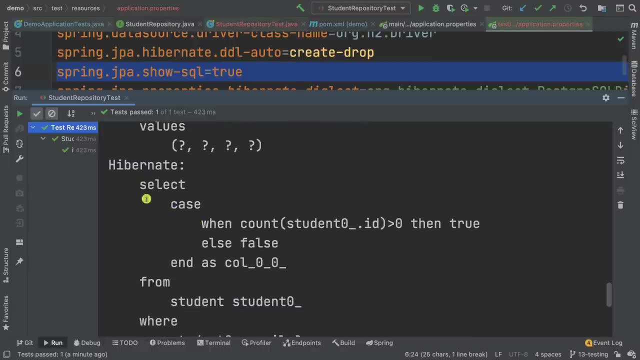 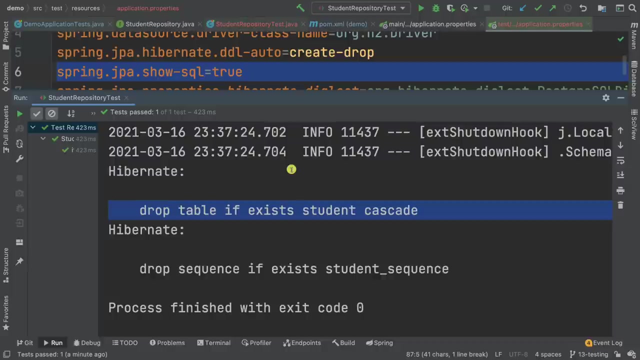 have great table And then we have some shenanigans about the insert, And then this is our select exists method. So this is when it was invoked And this is when the test ended. So it drop if exists, And you can see that our 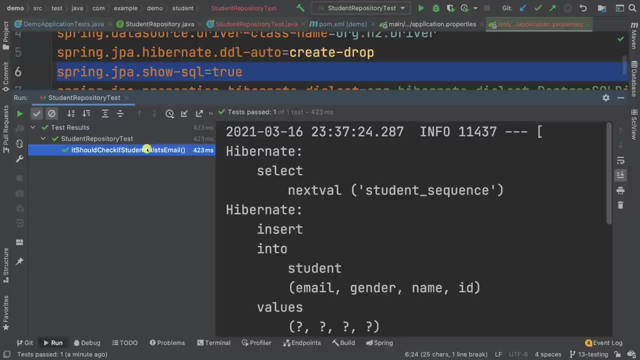 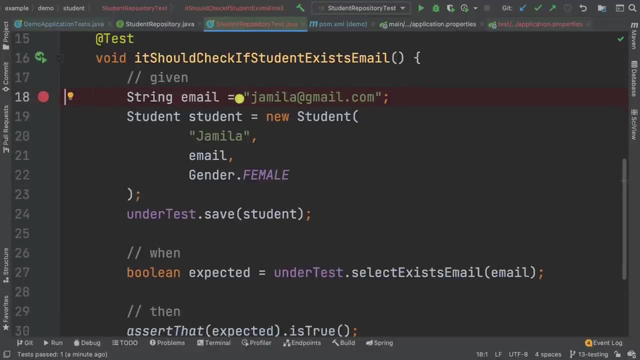 test did pass, So, which is really cool, Right? So let's now focus on testing. So, now that we have things up and running and working, you can see that this test did pass. Now let's have a second test. Let's just. 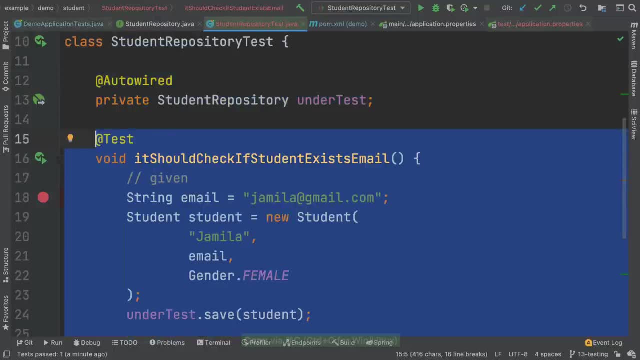 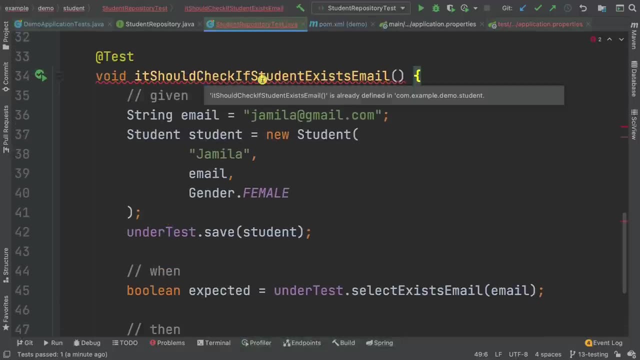 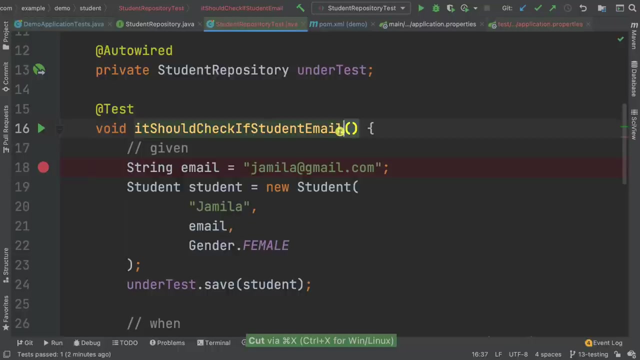 duplicate all of this in here, Command C, And then I'm going to paste that And in here it should check if student and this name should actually be if student email and then exists. So that was a mistake there. And here it should check if student email. 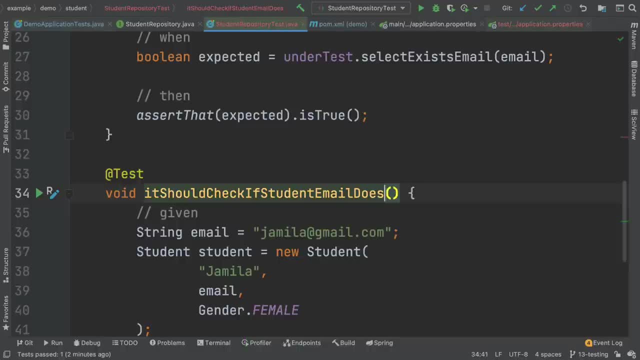 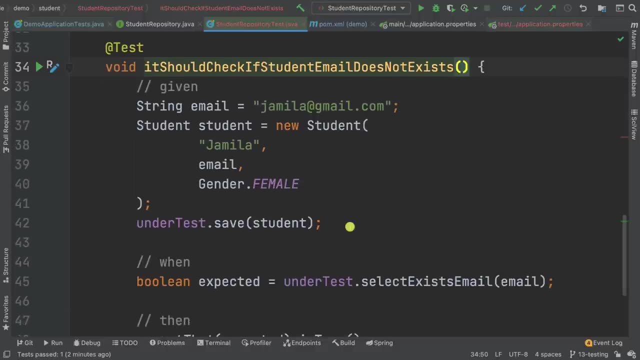 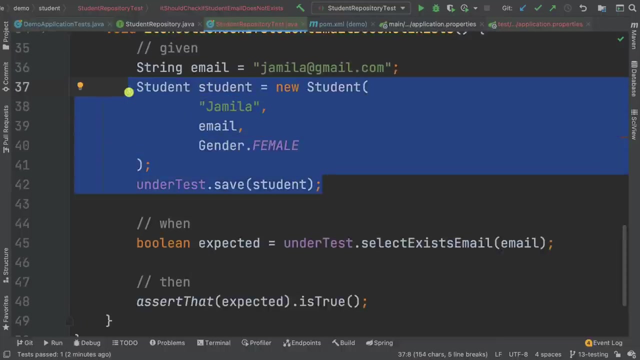 and then does not, And then exists. You can basically improve on the name of these methods And this method right here. what it should do is: So let's just remove this save, Right? So we're going to move that save because 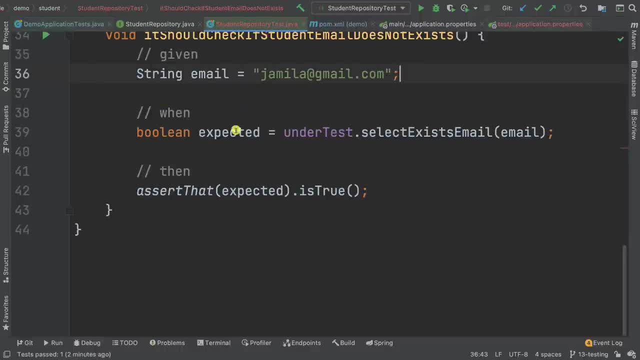 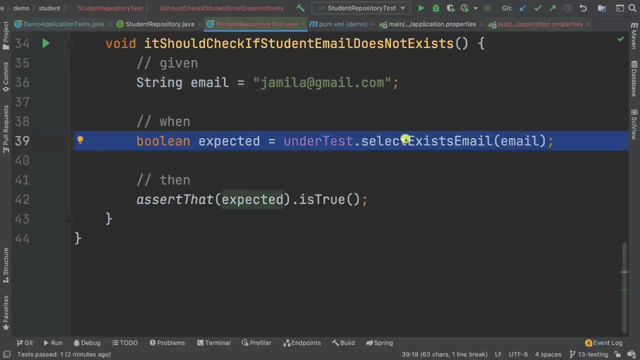 we don't want to save anyone into the database And here the expected is: given this email And then, when select exists email, this should be false. So is false because there is no one with that email. There we go, So you can see that. 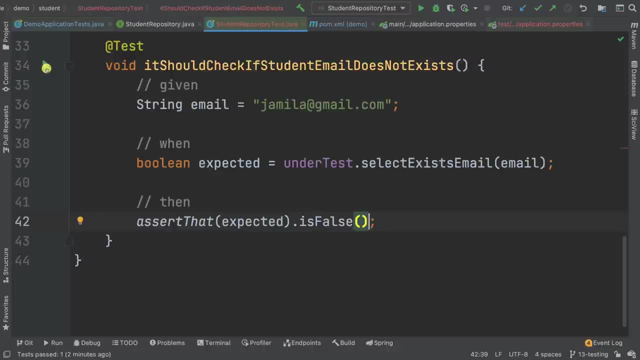 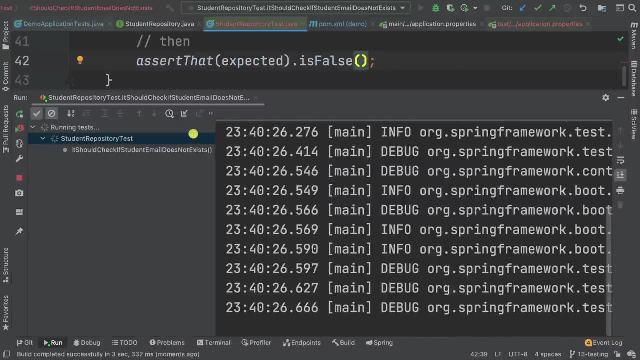 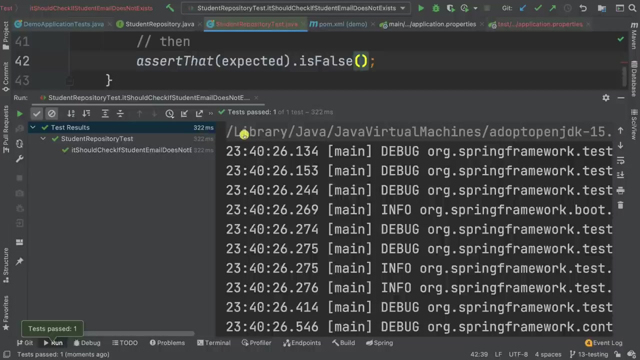 how easy it was for us to write a second test. So let's just run this one test And you can see that this test did pass. Now, one thing that I want to do here is: I want to have- So I'm going to press- control and 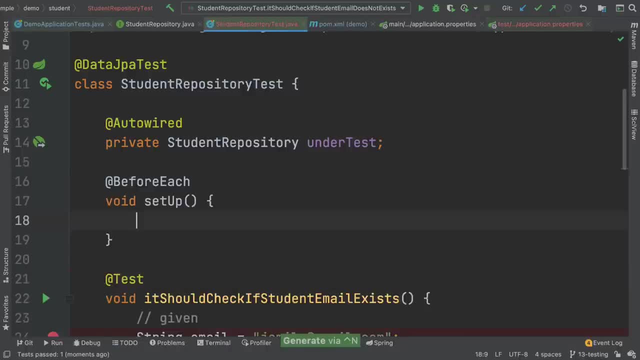 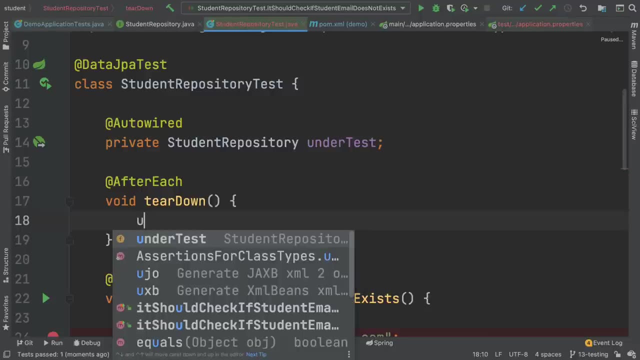 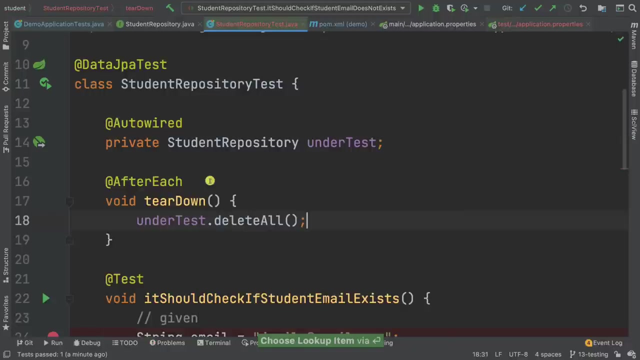 then enter, And here I'm going to say set up, And then here I want to say tear down, And then after each test I'm going to say under test, dot, and then delete all. So I want to delete everyone. So after each test I want to. 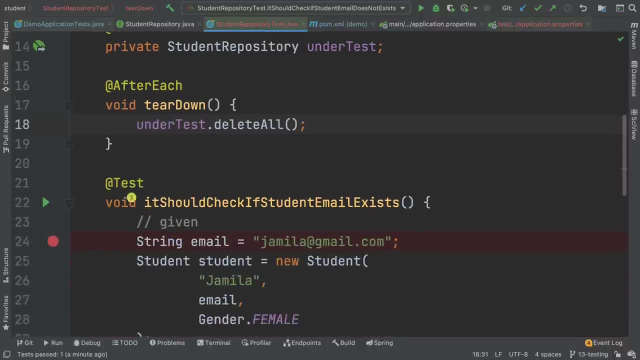 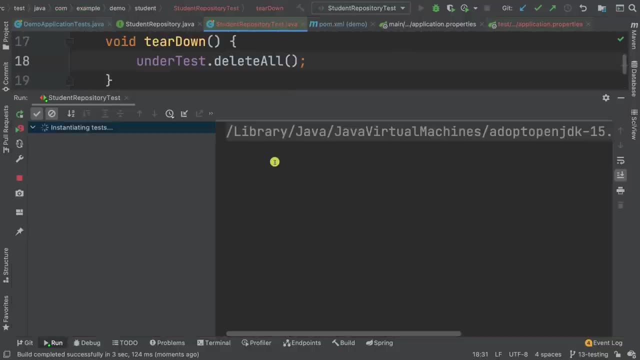 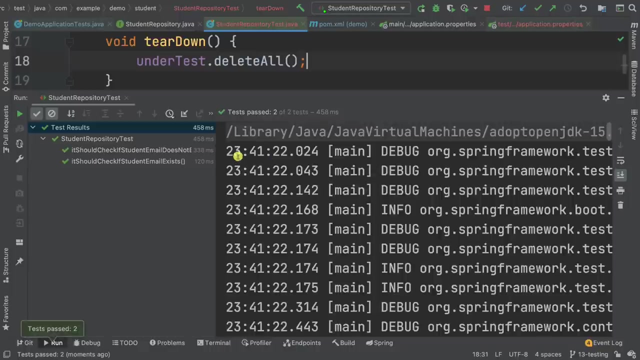 delete everyone, Which means that for each test, we'll have a clean state. Now let's run all the tests in this class And you can find all of this code and the decision of this video. And there we go. You can see that we have two tests and 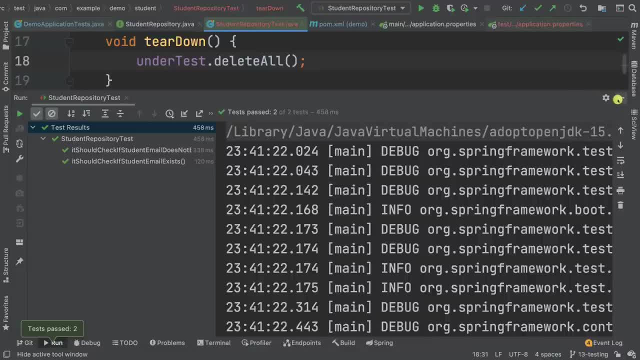 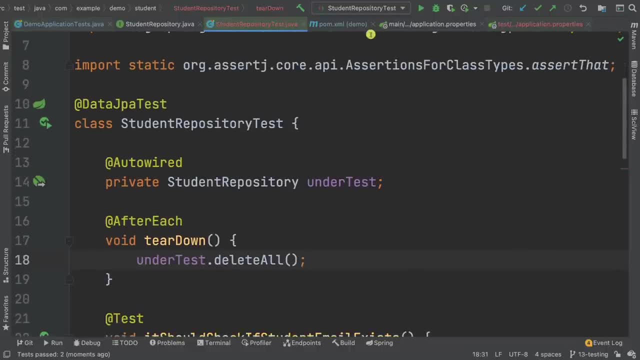 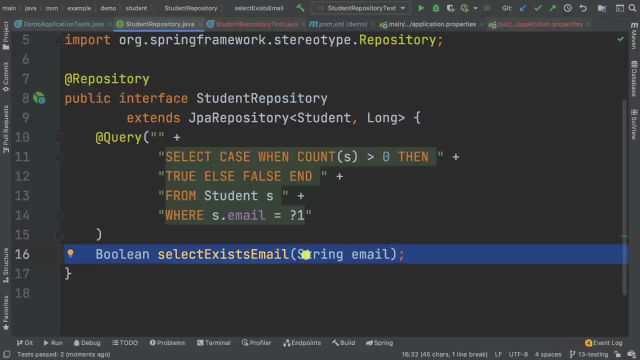 they did pass, So they are doing what it's supposed to do, So this is really cool. Now, one thing that I want to mention is that the only reason why we are testing this student repository is because we have this method, and this is our own custom method. 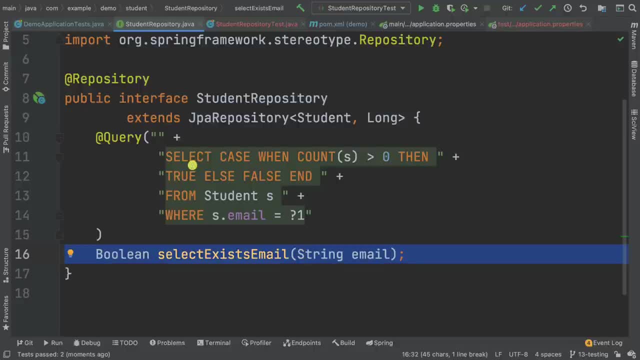 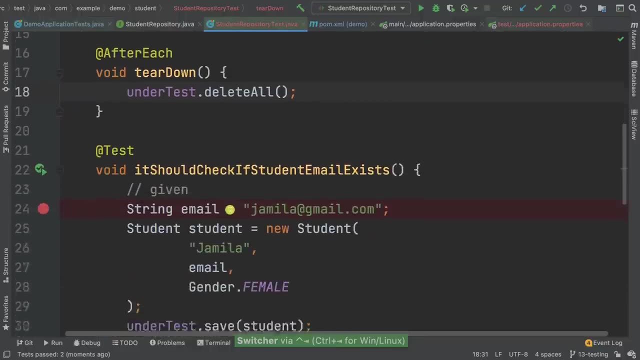 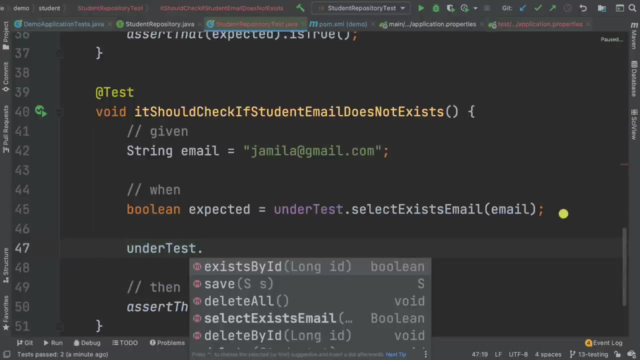 So we wrote this SQL query and it's important for us to test that our queries indeed work. But you see that, So if I go back in here, if I basically put my mouse anywhere, so here I can say under test dot, and then this: 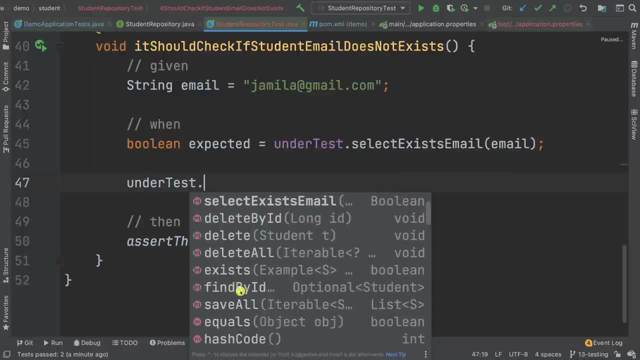 has a bunch of other methods, right? So delete all exists, find my ID, save, so on and so forth, Right? All of these are the methods. we don't have to test them because we didn't write any of that And it's provided by Spring Data, JPA and 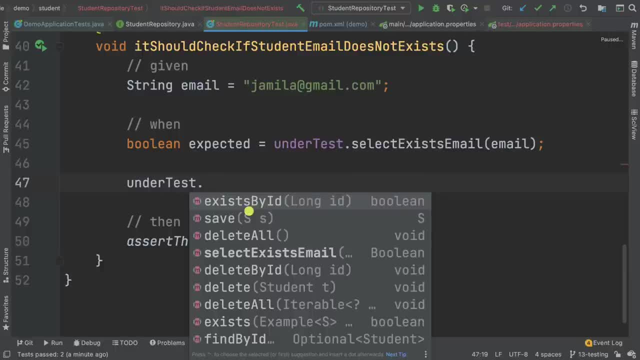 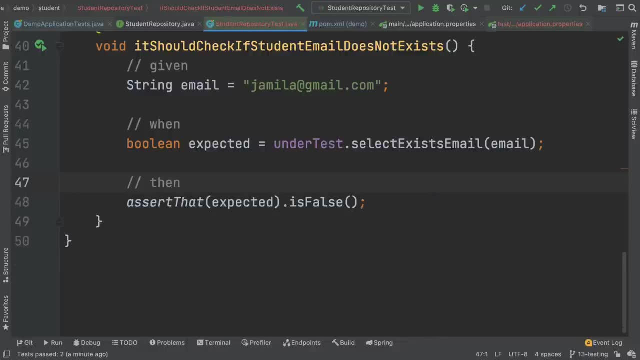 it's already been tested. That's why they provide it to us as an API that we can use. So for those methods, there is no need for us to test them, because it's given to us for free. The only methods that we have to test are the. 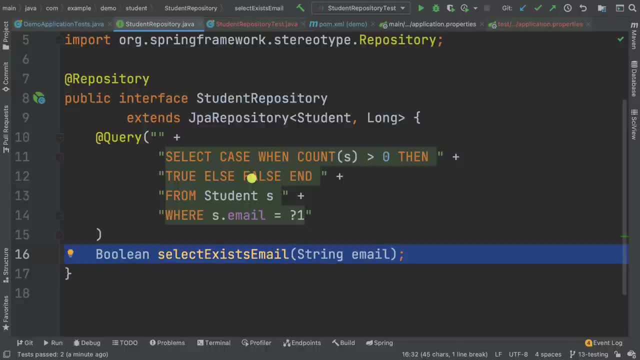 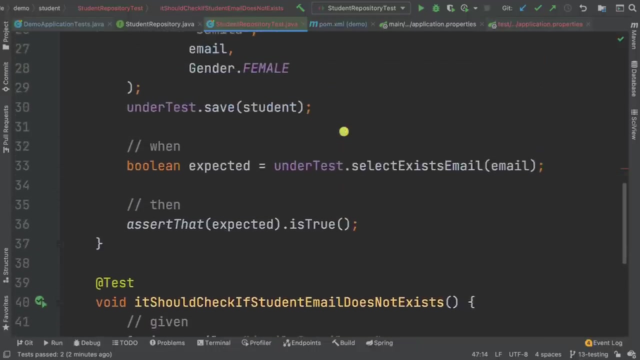 ones that we add in our interface. In our case, we tested that when we call this method right here, we tested both scenarios: where the email exists and when the email does not exist. So it should check if student email does not exist, and then it should check if student. Oh, actually, let's. 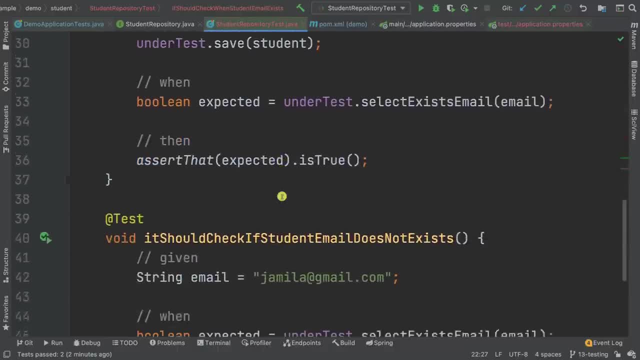 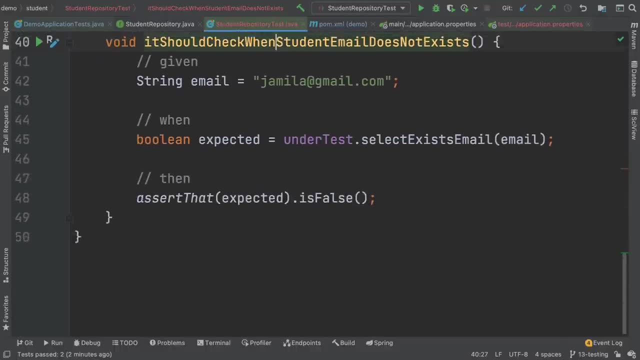 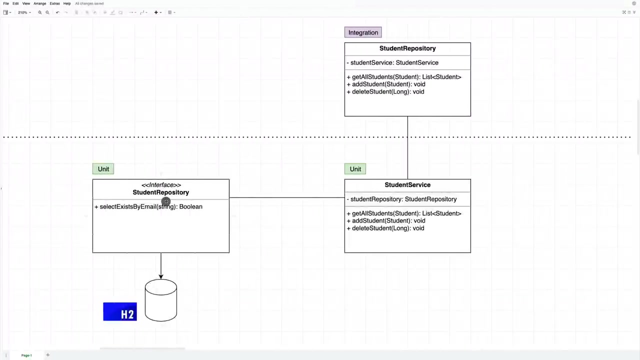 just say when. So naming things can be really difficult sometimes, but if or when it's the same thing. So there you have it. Hopefully you now know how to test your JPA repositories. So it's really simple. And if you break down things with given when, 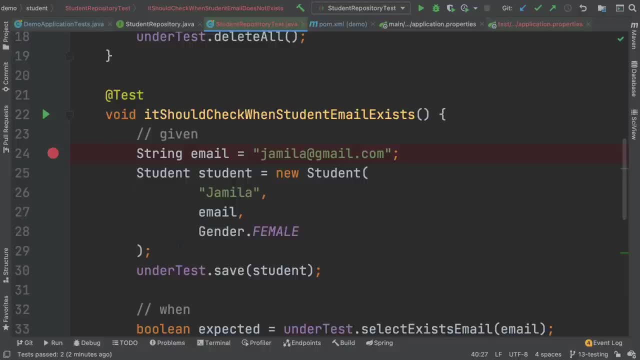 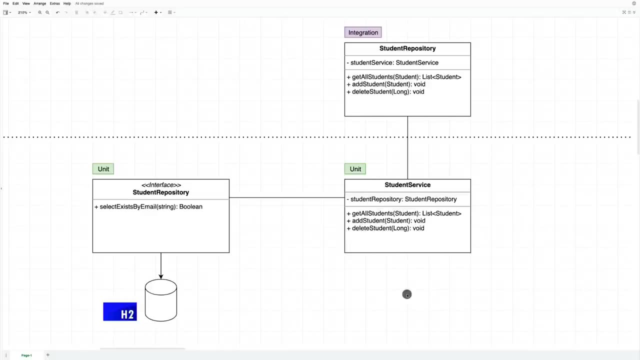 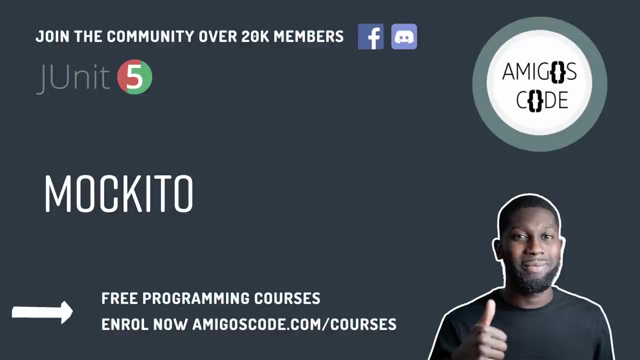 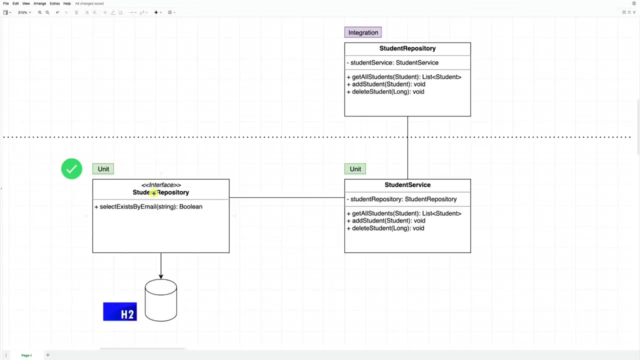 and then it's a piece of cake: testing your repositories. Next, let's go ahead and learn how to test the student service, And if you have any questions, please do let me know. Right, So we have tested this student repository. Now let's focus on student service. 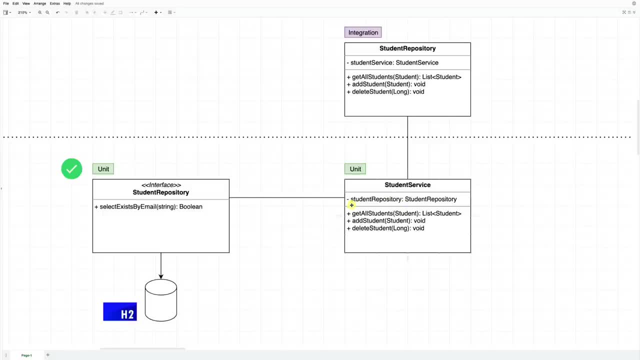 First I want to show you how you might want to test this, which will be the wrong way of doing things, And then I'm going to show you how to use mocking. So in here, let's go ahead and open up IntelliJ, and let's open the. 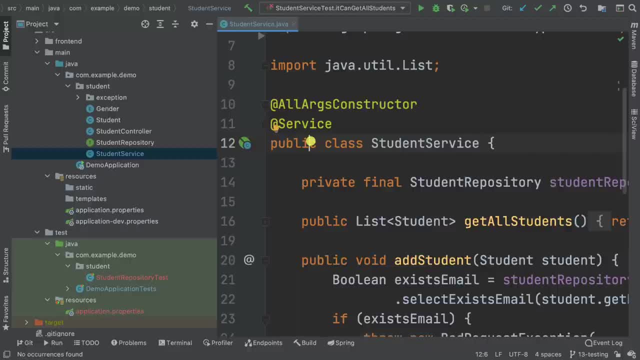 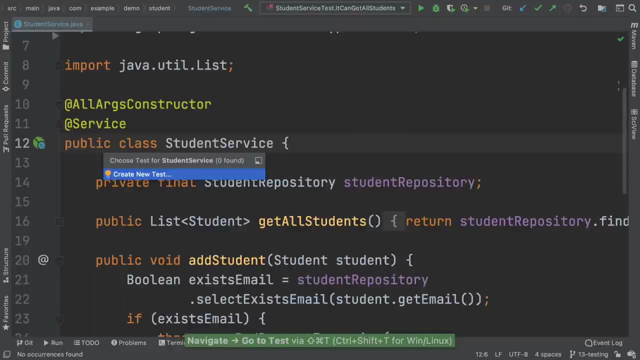 student service class. And what I'm going to do is I'm going to press shift command T, So I'm going to create a test And you can see that we have the dialog create test. And there we go. So J unit five. 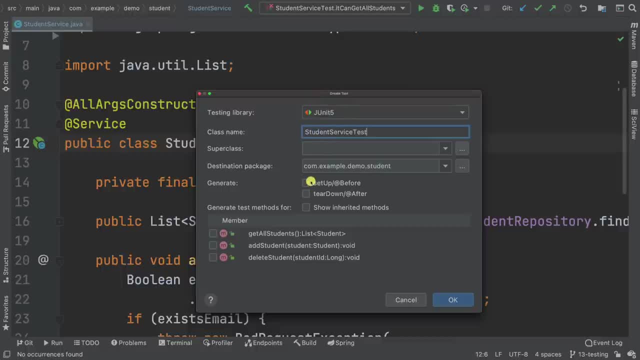 Then we have the class name and we can have the set up. So here, set up before, tear down, and then get all students, add students, so on and so forth. Let's just click on these three members And, by the way, we're going to. 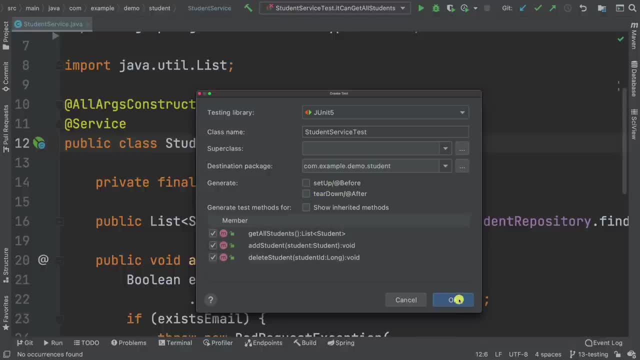 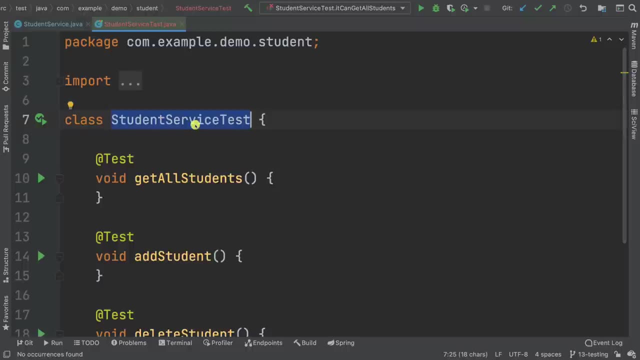 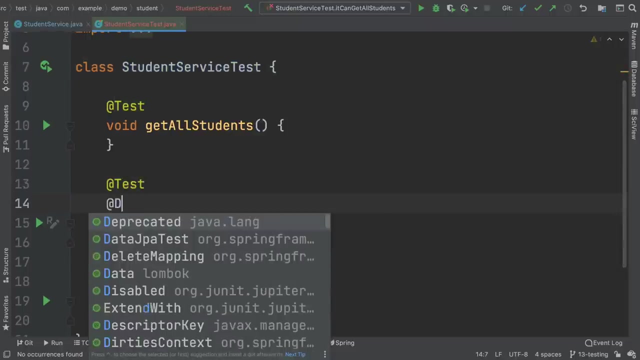 learn about set up and tear down in a second. So we're going to use them and just say, okay, so now in here. so we have the student service test right here and we have three methods right. So currently I can just even say add and disable. 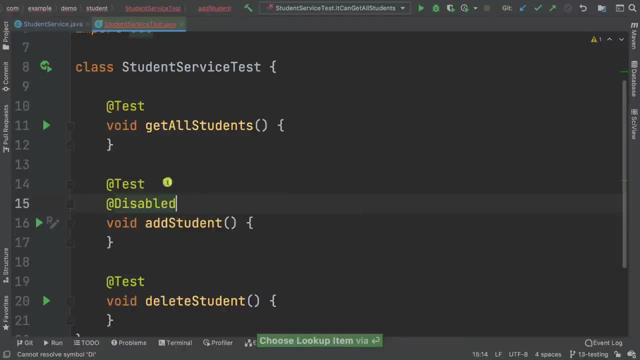 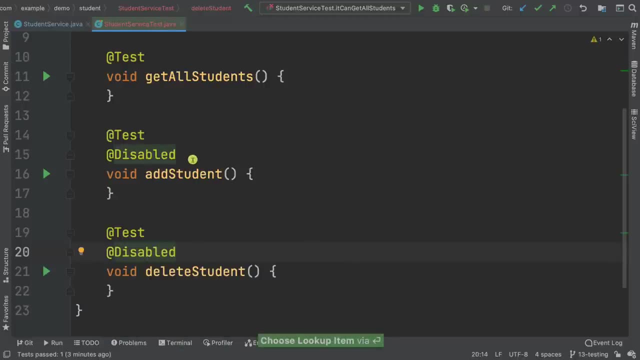 So this is you learning a new annotation and this will disable these tests, which means that they won't run. So I disabled and they won't run. Now in here I can go ahead and let's test that we can get all students. 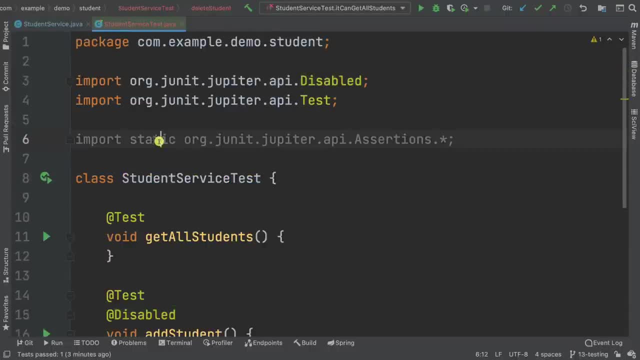 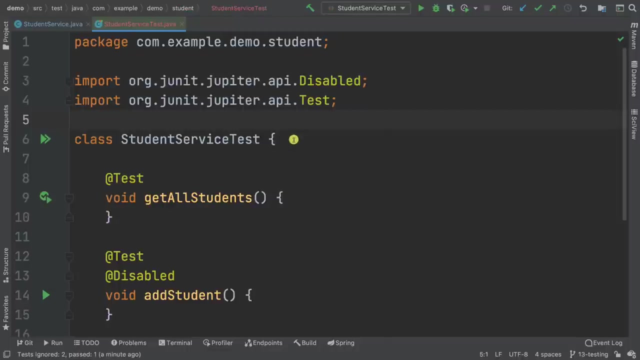 So you might even think that the best way for you to test this- And, by the way, let me just remove the Jupiter API assertions because we are using assert J, So in here you might think right. So in order for me to test, get all students, we first need to have the test. 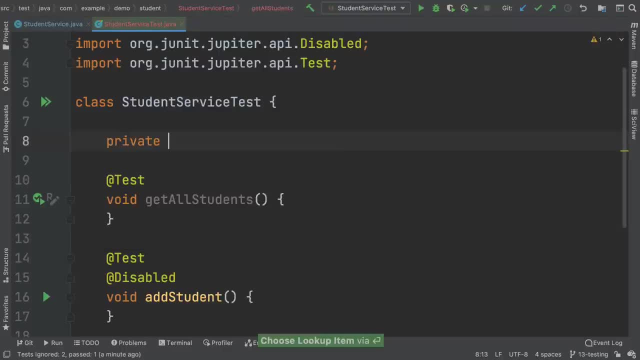 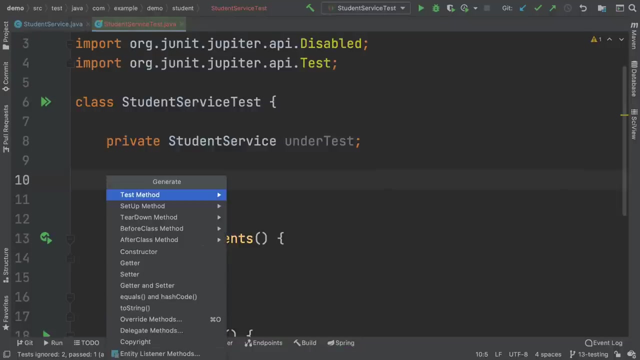 So here let's say private, And then I'm going to say student, and then service under and then test. And here let me just press control and then enter And you can see the keyboard shortcut And I'm going to generate the setup. So in here. 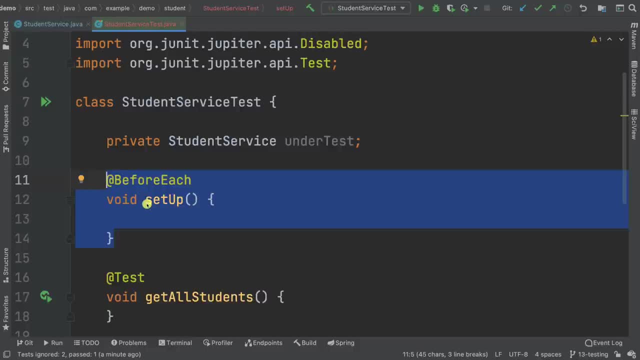 we could actually have selected this method from the previous dialog, But in this setup, So this will run before each test, I'm going to say under test equals to new, and then student service. Now, inside we need to pass the student repository. Now, the way that we're going to do this is the following: 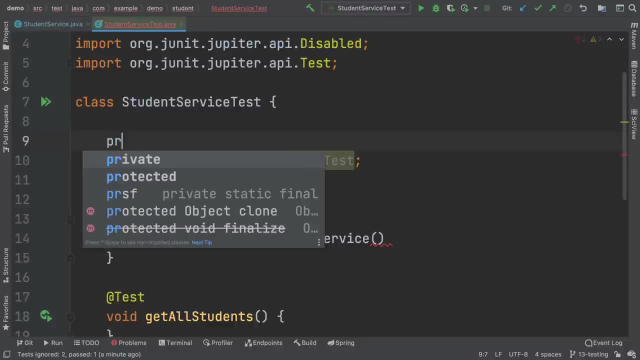 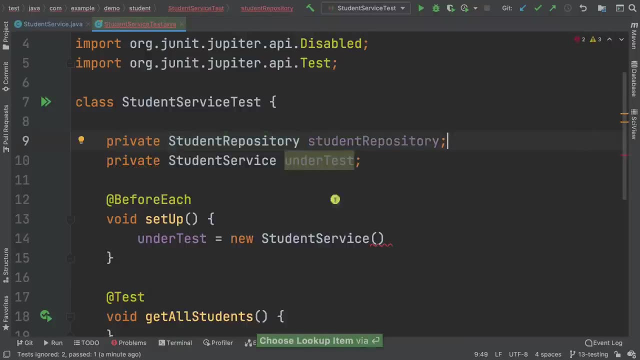 So in here I'm going to say private, and then student, and then repository, repository, and then pass student repository in here, just like that. And now before each test we're going to get a fresh instance for student service. Now in here let's just say that. 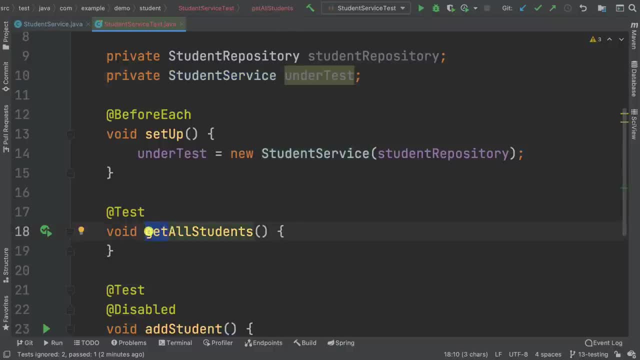 let's change this name here to can and then get all students, And what we're going to do is the following: So, basically, this test is super simple, And that's because, if I press shift command T and go back to student service, you can. 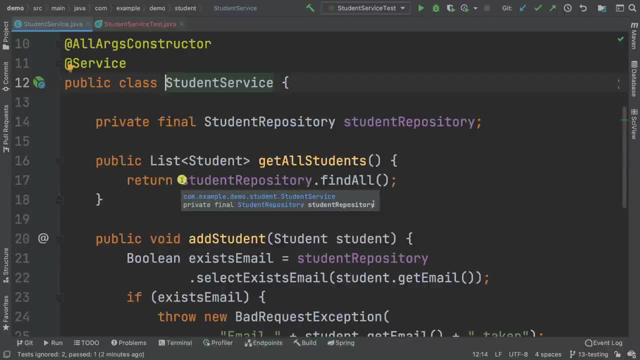 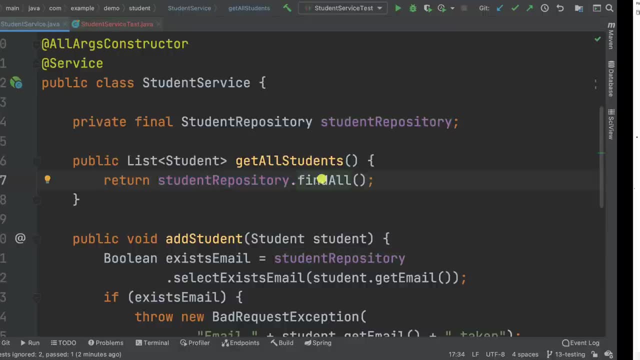 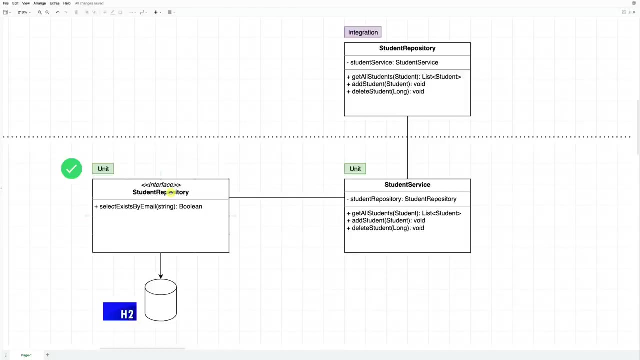 see that the only thing that it does it just calls student repository dot find all. Now, when it comes to unit testing, if I go back in here for a second, remember this student repository has been tested. We tested in isolation and we know. 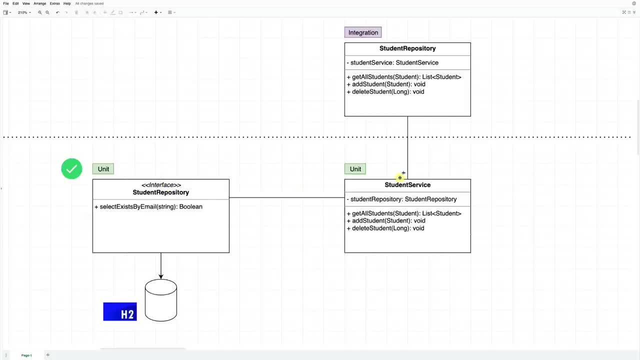 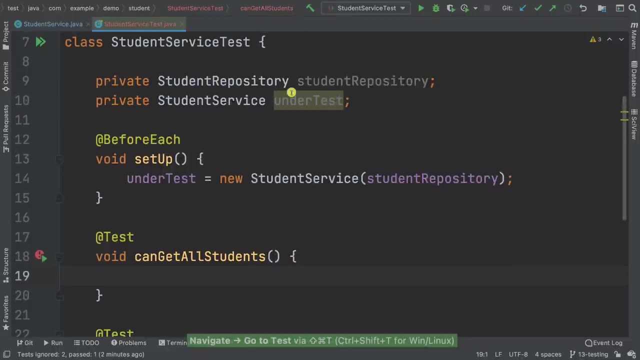 that it definitely works And inside of student service we have a reference or we have a field of type student repository. Now you might be thinking that perhaps we can go back to the test and then here: So this shouldn't repository, Maybe we can just say add and then auto. 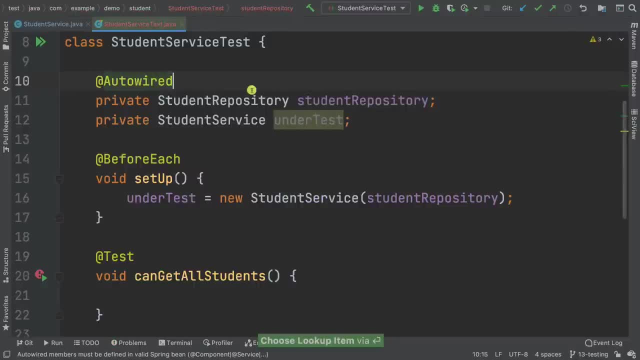 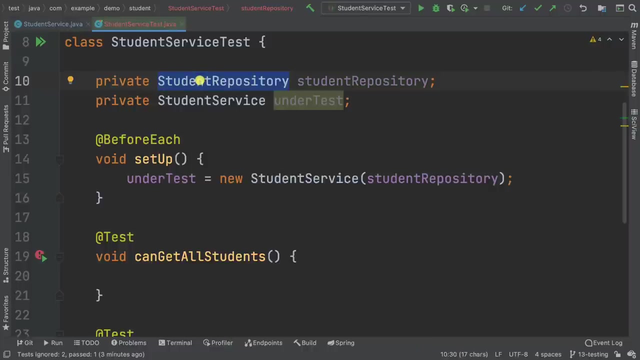 wire Right And then we get the real instance for student repository and then we can add new students, the leads on and so forth. But in reality we don't want to do this Right. We don't want to do this because this student repository- we know that for fact, indeed. 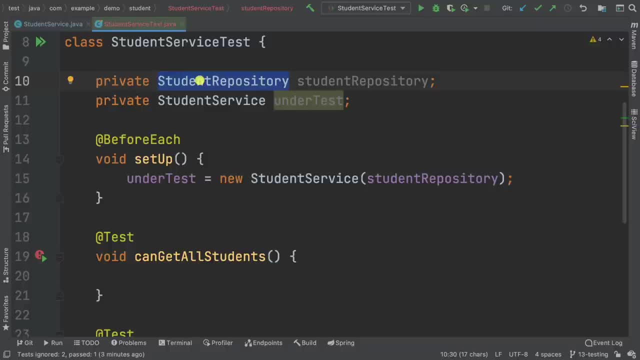 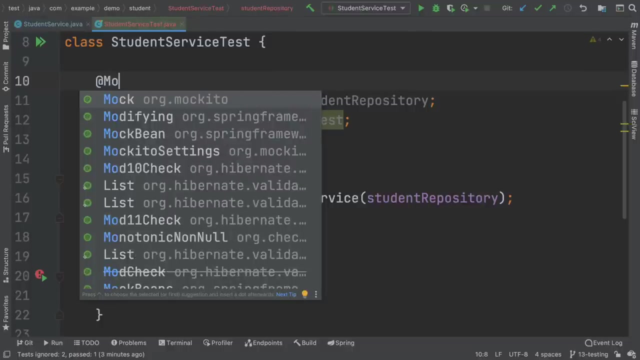 its implementation is good enough, Right? So every single method that we have in it does work. And this is when we mock this student repository. So we say, right, So here we want this to be a mock using Moquito. So this is org Moquito, just like that. 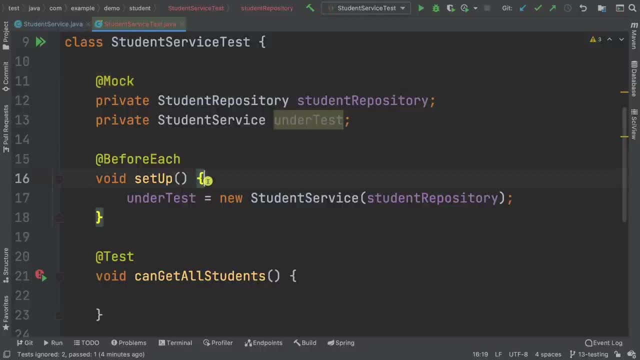 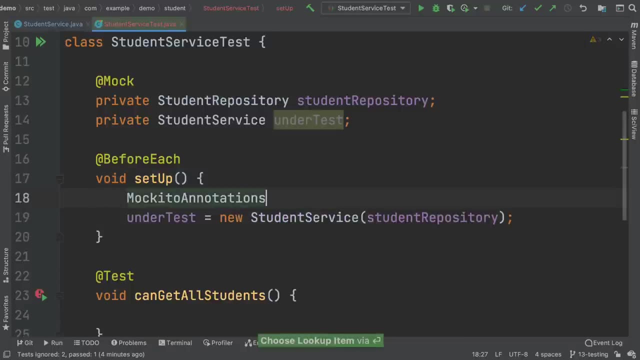 And now what we need to do is the following. So here, in order to initialize this mock, we need to say that Moquito annotations dot, and then open marks, And then inside let's just say this: So, basically, if we have more than one mock, 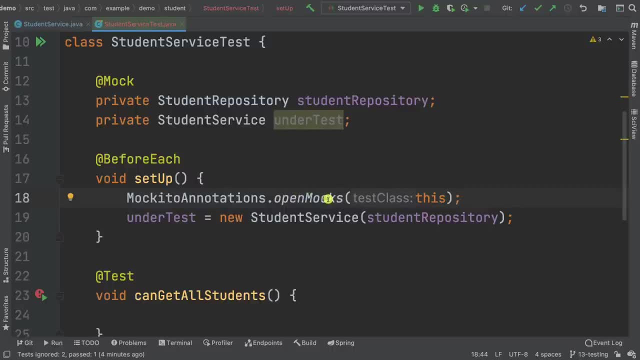 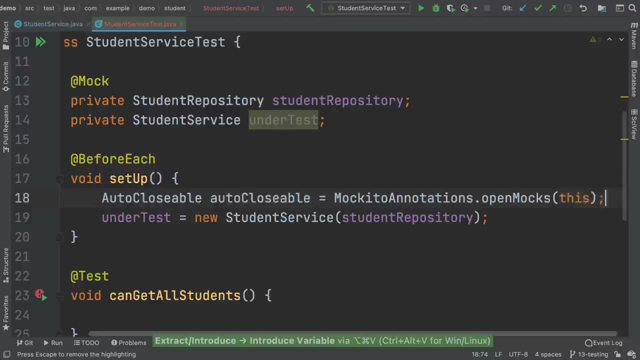 it will initialize all the marks in this test class and this. So this returns a closeable. You can see here closeable. And what we're going to do is the following: We're going to take this just like that. So I've just pressed shift command V to extract. 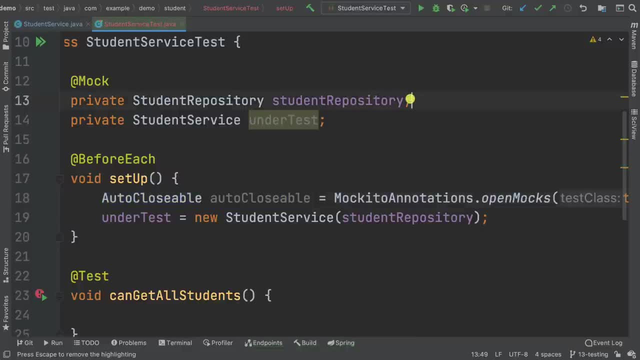 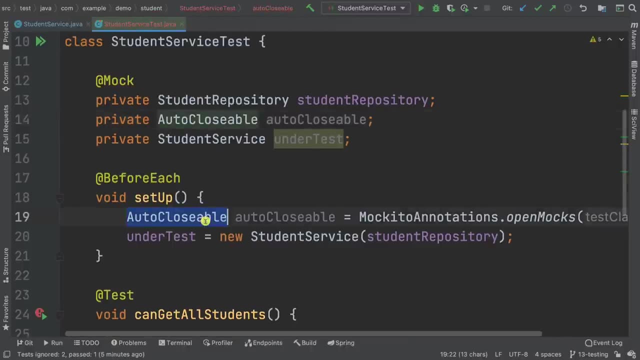 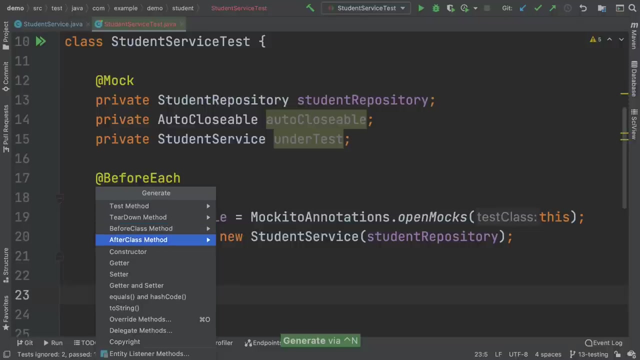 to a variable, And here I'm going to say this will be private, and then paste that, And here I'm going to say that this will be equal to that, And then after each test, So after actually tear down method, So here after each, we're going to say: 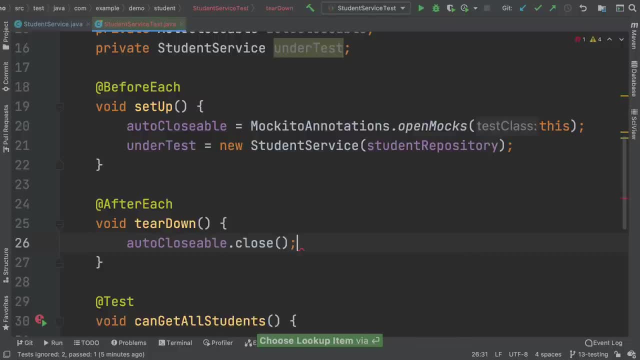 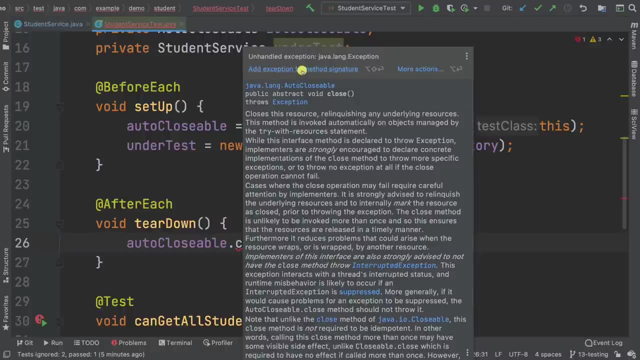 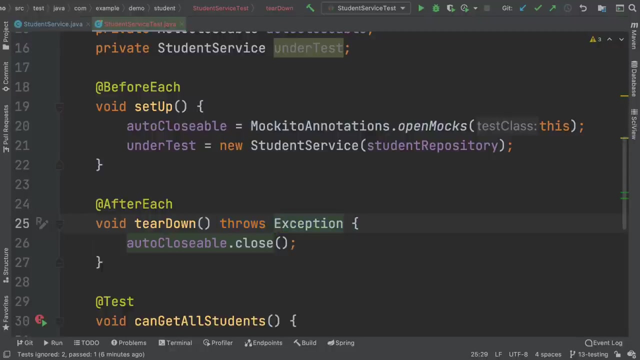 a auto closeable dot and then close. So this allows us to close and this actually throws an exception. So it's fine. Let's just say that we change this method to throw this exception. So this will allow us to close the resource after the test. 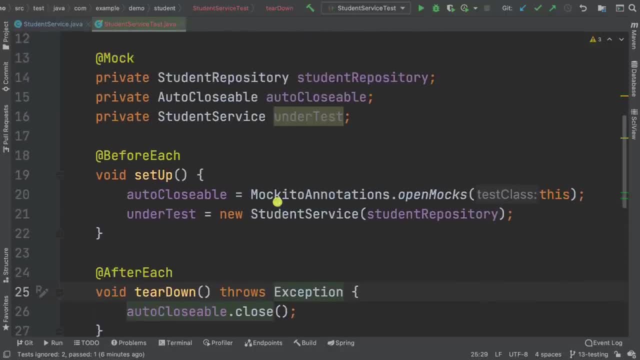 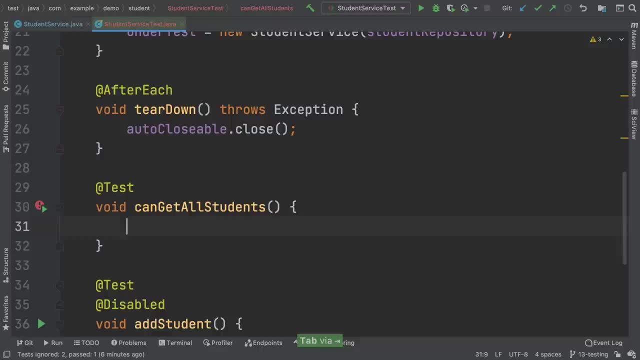 And now so we have things set up. So let's just in here. So now we can go back to testing our method. And the way we're going to test this is we're going to pretty much just say when and then under test dot get. 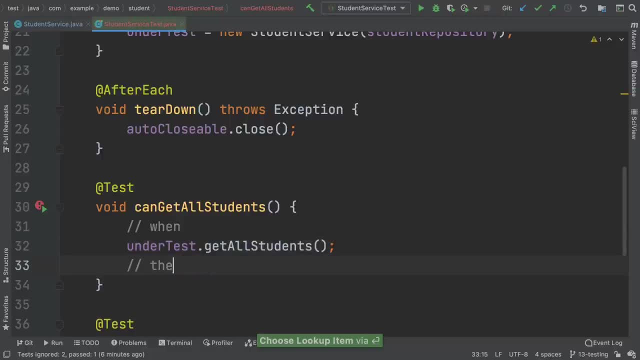 all students. Then in here we're going to say verify, And we need to import this from Okito. So here, import static method And this should come from Okito, So verify, And this will be our mark. So student repository. 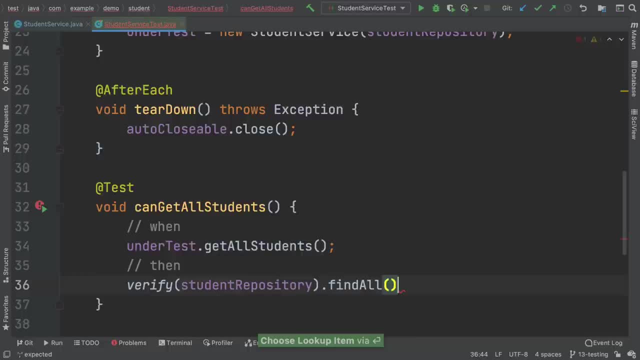 And then I can say dot and then find all. So we want to verify that this repository was invoked using the method find all. So you can see that this is a little bit strange, right, But what is happening is we basically don't want to test the real student repository. 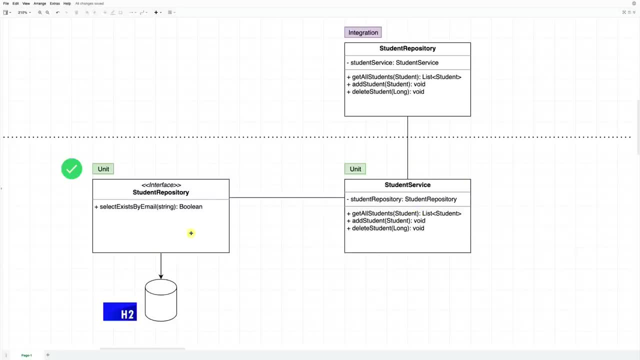 when we are testing the student service because student repository, we know that it works for fact and then we can just mark its implementation inside of the student service test And the benefit that we get with that is that our unit test is now fast, so we don't have to bring up the database. 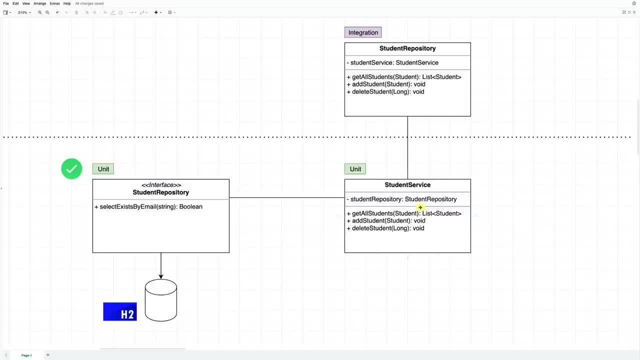 create the table, so on and so forth, Insert a new student and drop the database and all of that stuff that you've seen when we tested this repository. So we've done that work once. Therefore, anywhere that we use this repository, we just mock it as we've done it within. 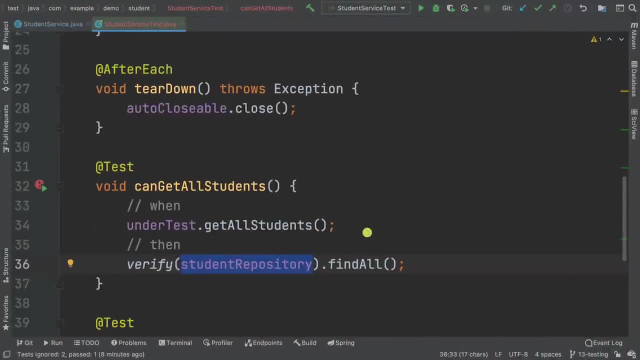 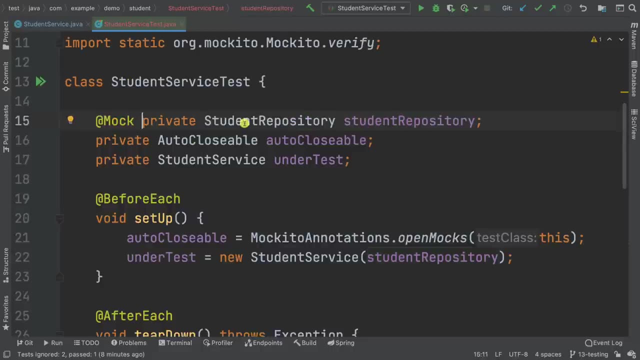 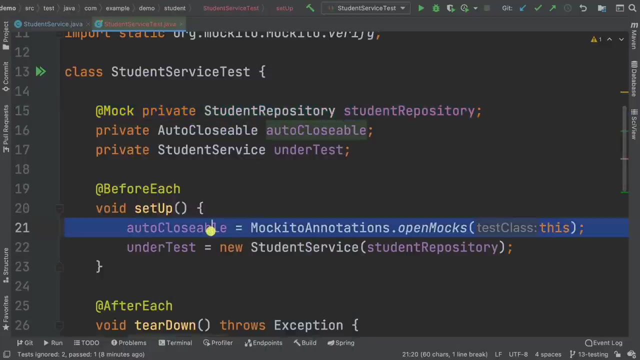 this student service. So in here, this is what we're doing. So basically, we have a mark, So let me just put like that. So we have a mark for the student repository and then auto closeable. And this is because of Mokito, And I'm going to show you a better. 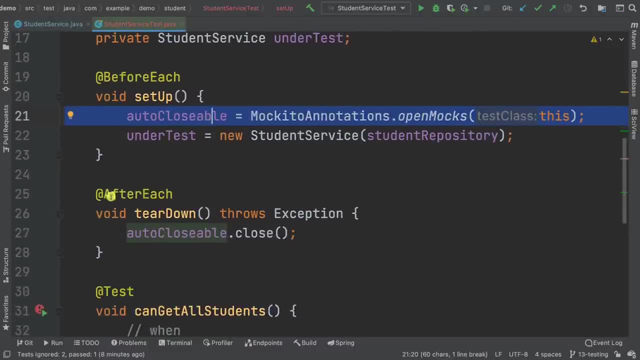 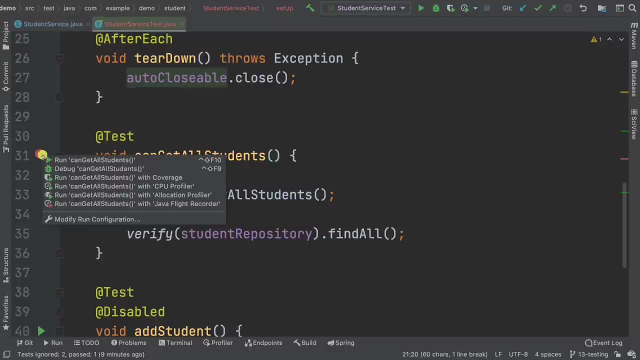 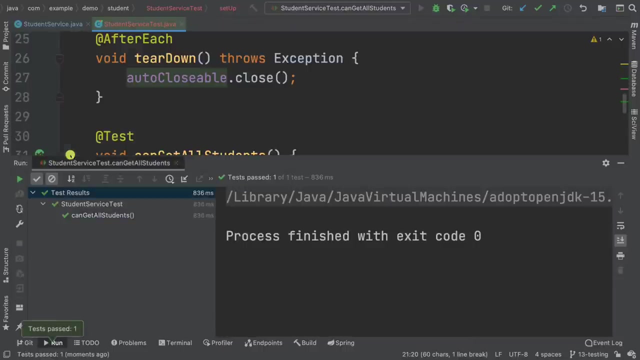 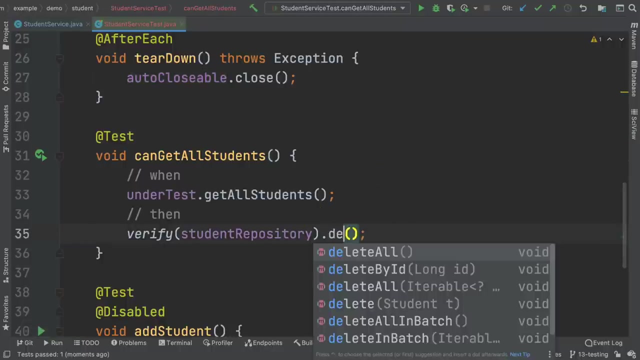 way of doing this in a second. And then we have the after each, which we didn't close the resource, And this is our test. So if I run this test, you can see that it works right. So here, if I say: verify that the method, delete all. 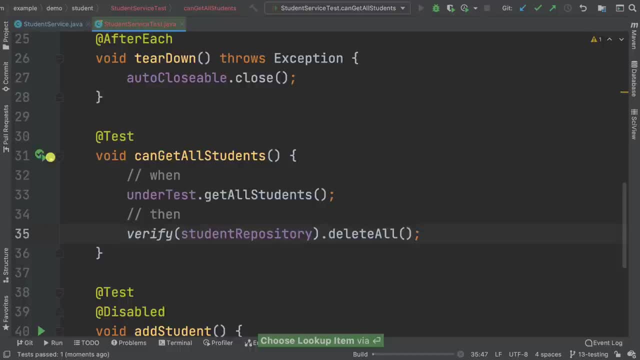 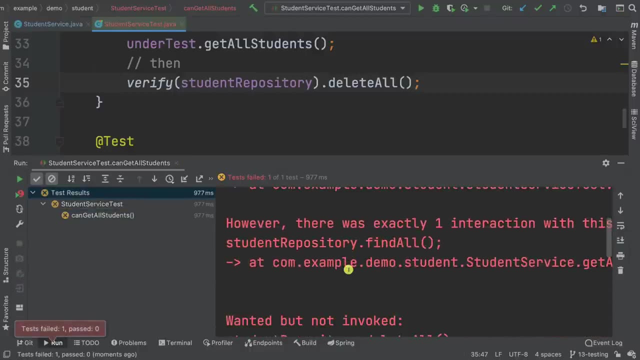 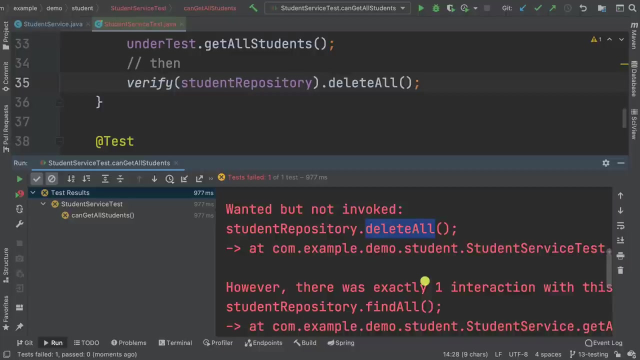 was invoked, So this should fail. There we go. So this fails, Right, And it failed because you can see that. wanted but invoked, delete, all Right, And you can see that. However, there was exactly one interaction with this mock and it was fine. 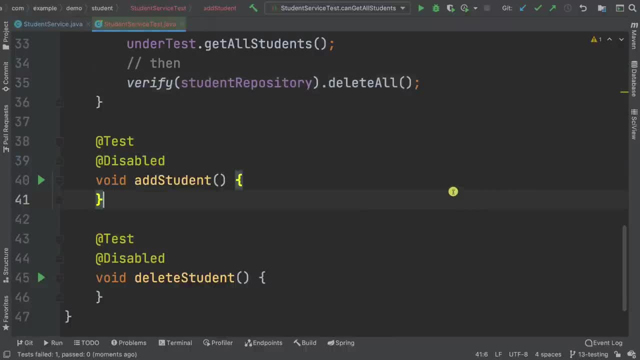 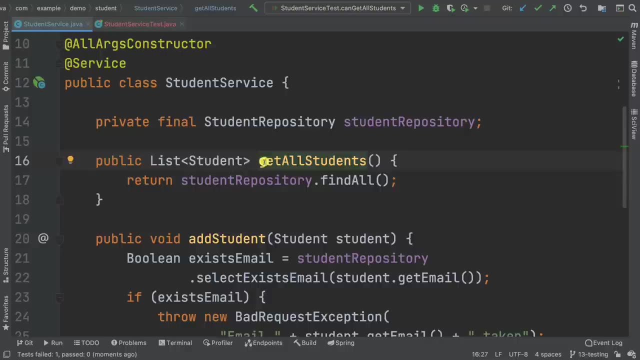 All. So if I go back to the student service, so shift command T here. So when the end the test was invoked, so get our students the mock was invoked with find all And again. we just have to verify that this is called because 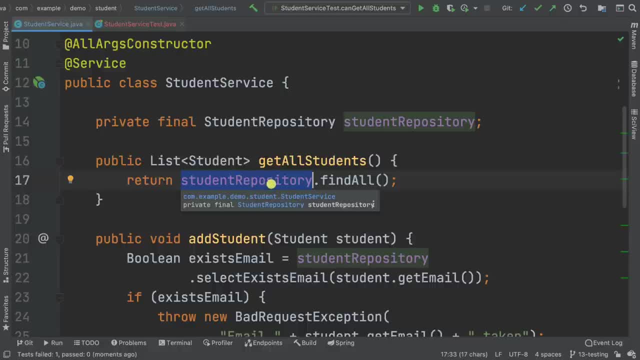 we know that whatever this returns indeed does work. And also, we didn't write this method find all. And this is a good way of actually mocking things right, Because this is given to us for free and we just rely on its implementation. 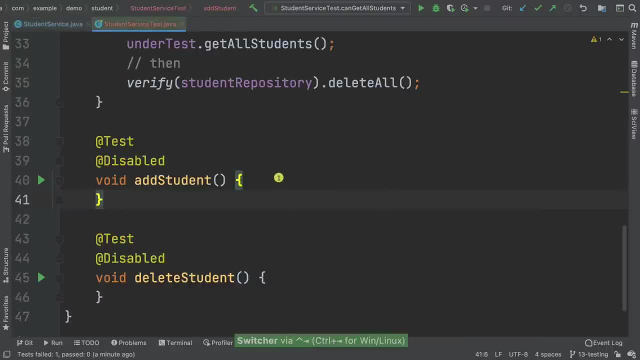 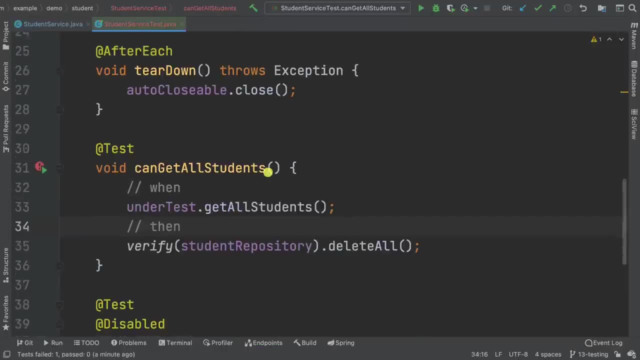 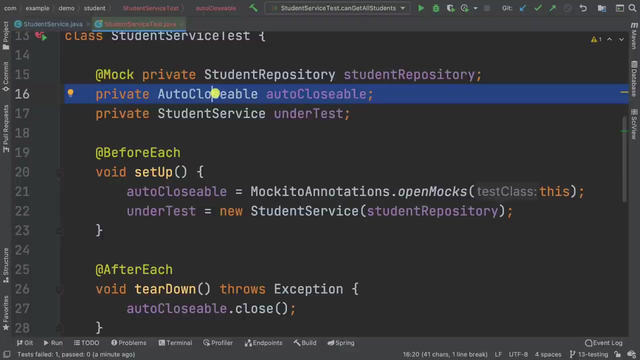 So there you have it. This is pretty much how you test using Mokito. Now, one thing that I want to improve here is, you see that this can be like a little bit confusing and some boilerplate code, So let's just remove this. Let's remove this. 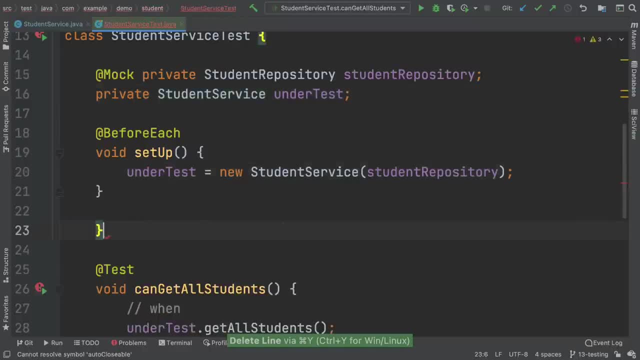 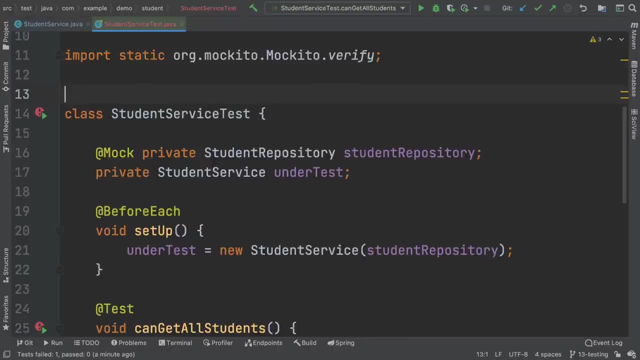 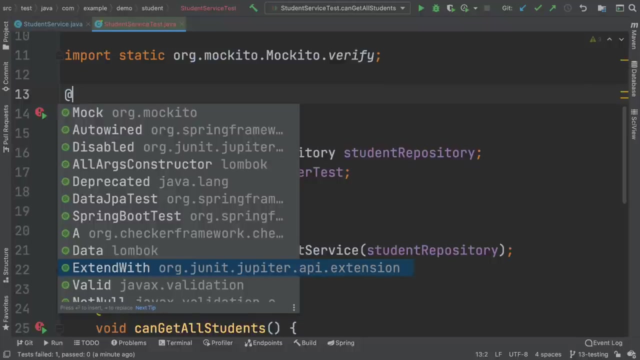 as well, And let's remove this, this, this and that line. And then in here, so for this class, we're going to say at, and then extended with org dot J unit, dot Jupiter, API extension. And then here I'm going to say Mokito. 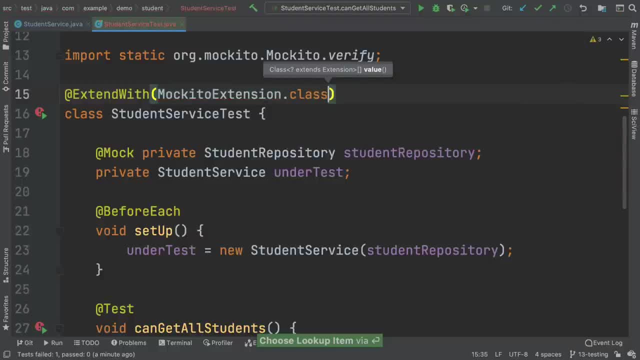 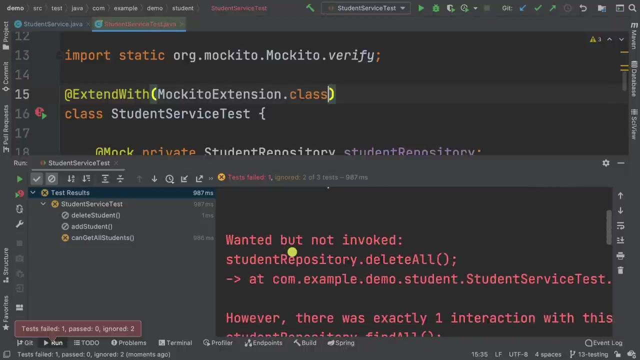 and then extensions, dot, and then class. So that will actually do what we had before. So you can see that this is much cleaner now. Now, if I basically run all the tests in this class, you can see that the test failed And that's because we have to change this. 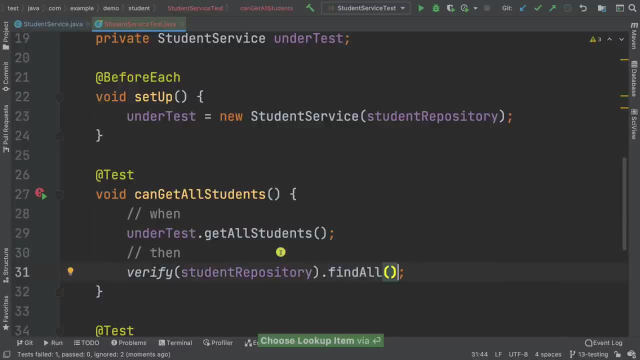 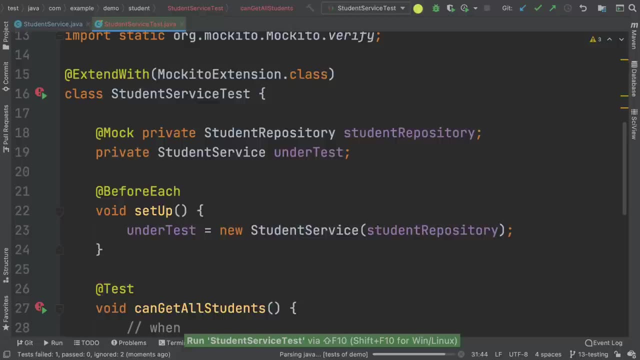 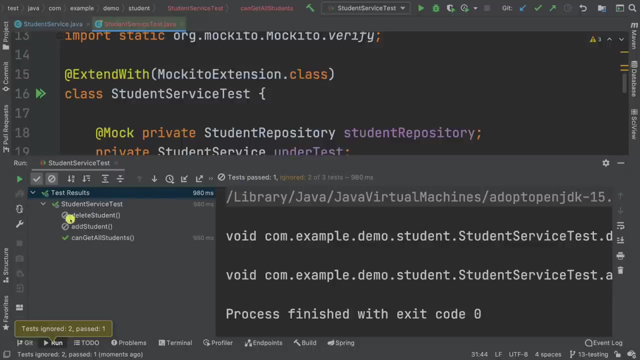 verifying here to find all. And let's run the tests again And you can see that it works And these two tests are disabled. That's why they're like that. And you can see ignored two out of three tests. So there you have it. 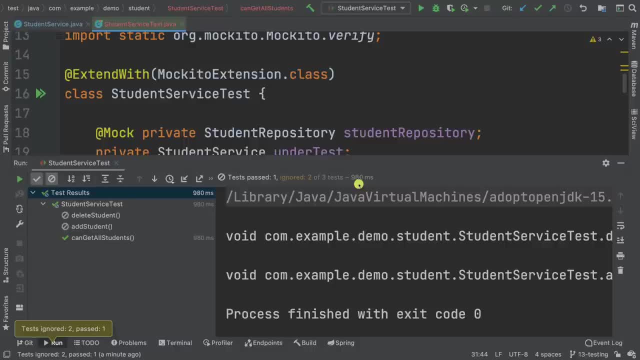 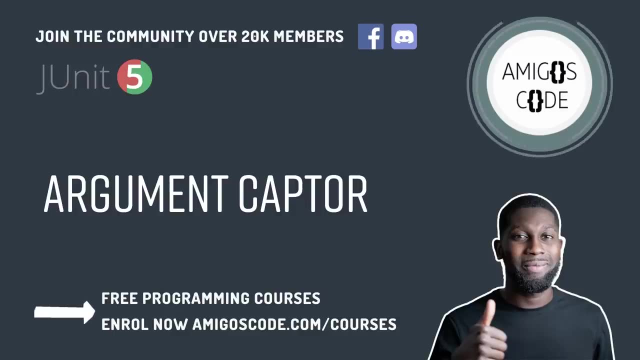 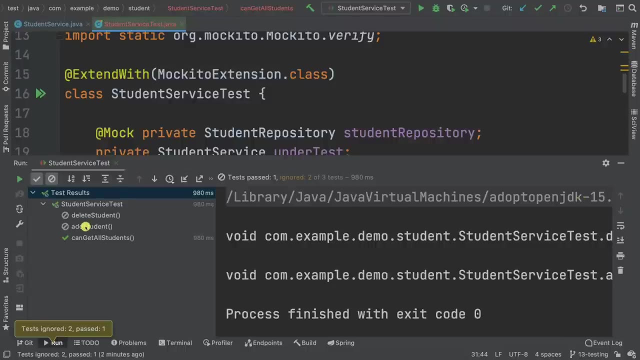 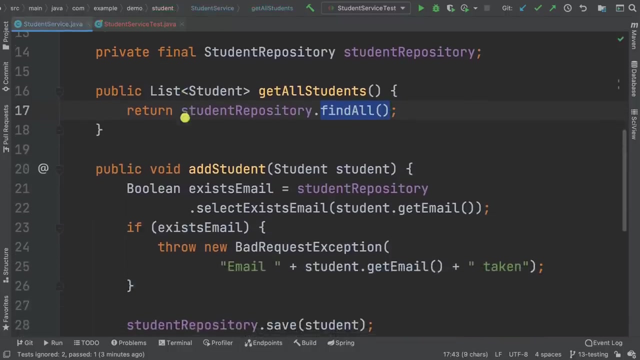 If you have any questions, drop me a message, Otherwise let's move on and test the add student method. Okay, Right, So let's test the add student method. So here let me just show you again. So if I go to student service, so add students. 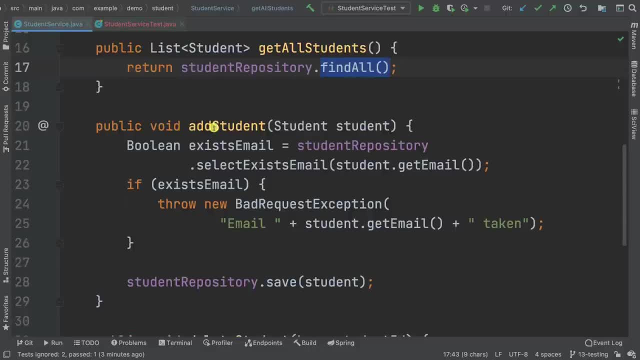 So this is what we want to test, Right? So add student. Now here we're going to use mocking again because, remember, we tested that select exists, Email works Right. So we have tested this method. So in here, remember before in the repository. 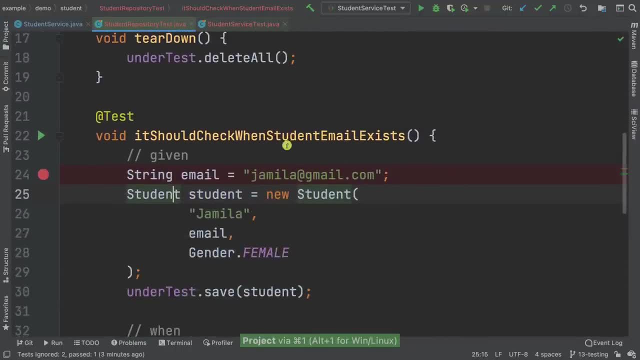 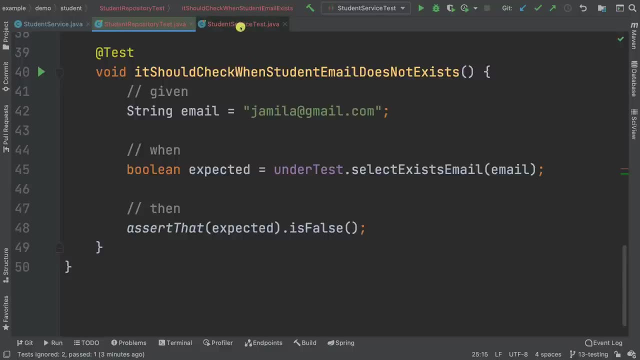 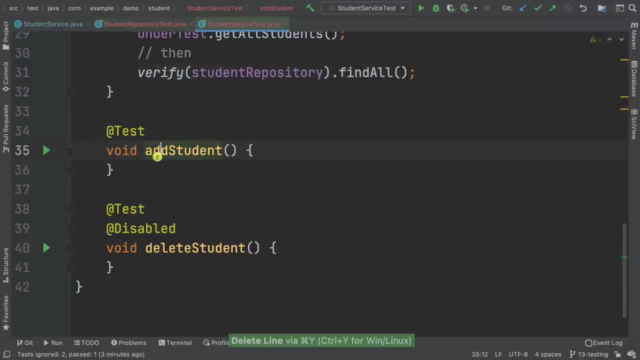 So we have two tests, So one that checks when the email exists and the other one that checks when the email does not exist. So, when it comes to test this, this is what we're going to do. So here I'm going to remove this annotation at disabled. 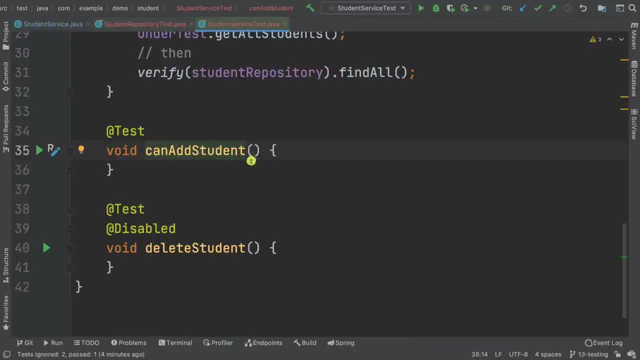 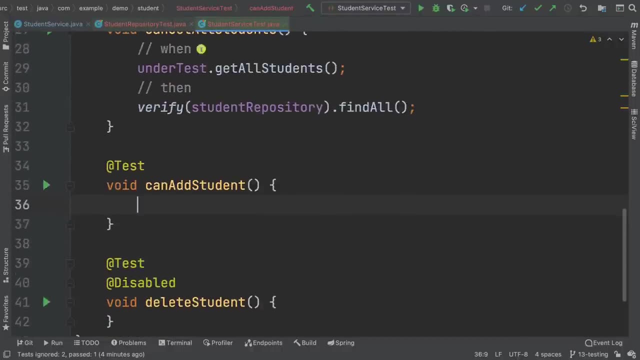 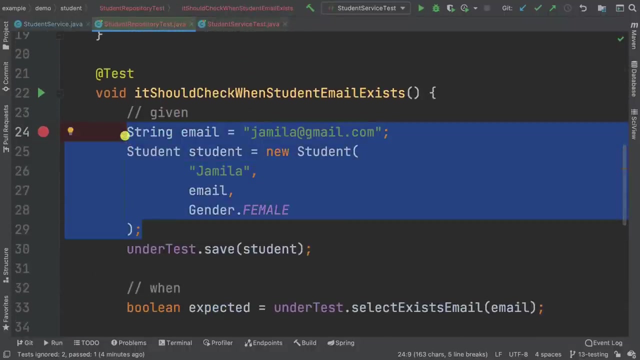 And then I'm going to say can, and then add, and then shouldn't, Okay, And here let's: basically we need to grab one student, So let's just copy some code. So from here we have this student, There we go, And if I go back so can add student, I'm going to paste that. 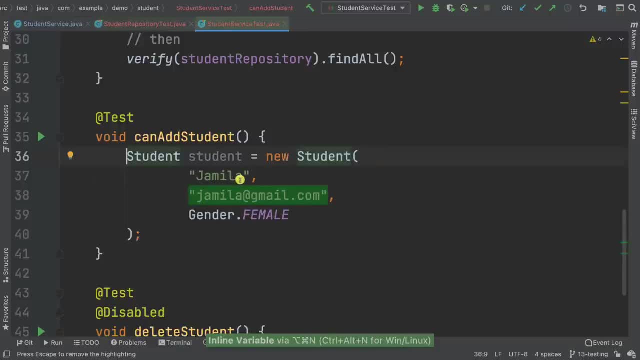 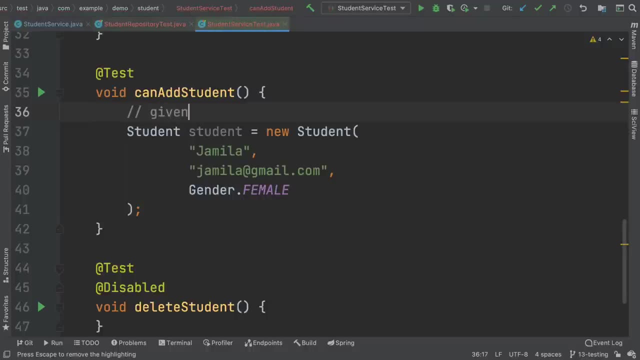 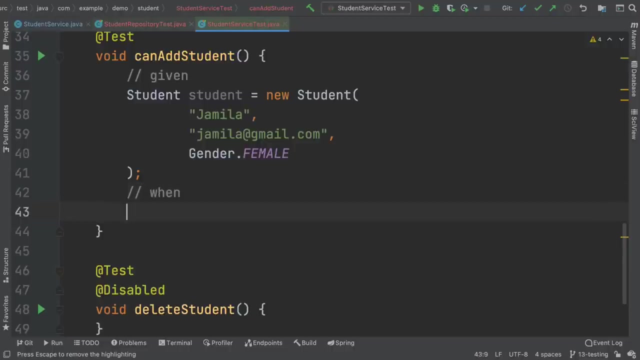 And then here I'm going to indent or actually inline that. So now I'm going to say given, So I like to have all my given, So given. And then here I'm going to say when, And here we're going to say under test dot. and then add: 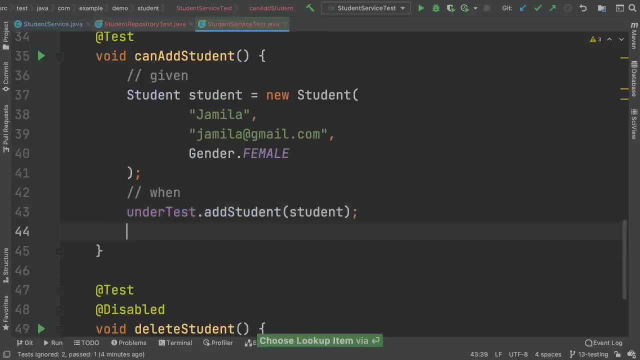 student, We're going to pass the student. And then here we want to say: then Right, So what we want to do? So what we want to do is we want to basically check that. So, student service, Let's go back. 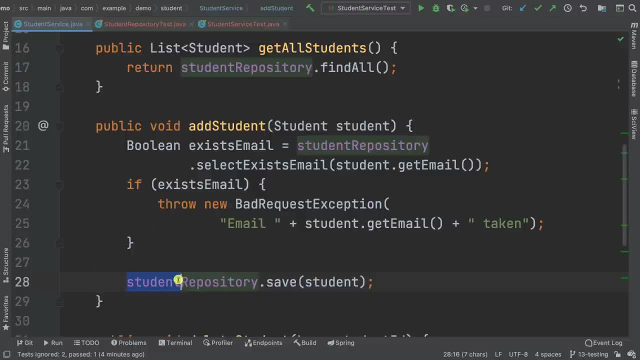 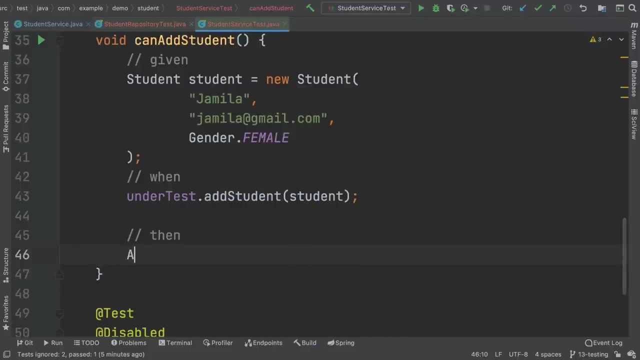 We want to check that the repository, So student repository- was invoked with the same student that we passed. So how do we test this using marks? Well, it's very simple. So here what we need is an argument, capture. So I'm going to say argument and then capture. 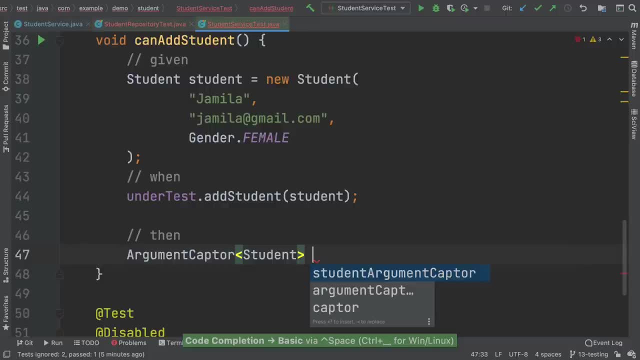 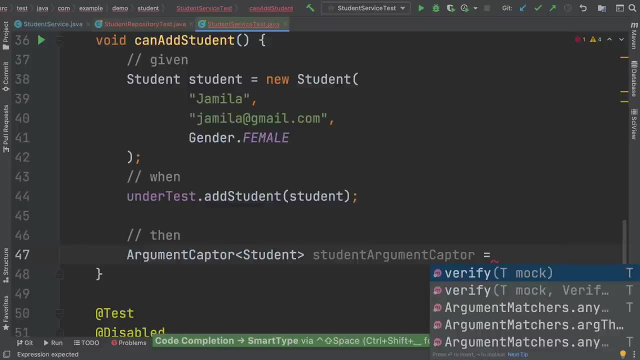 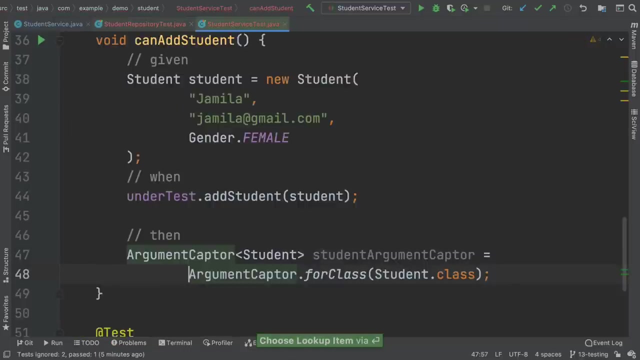 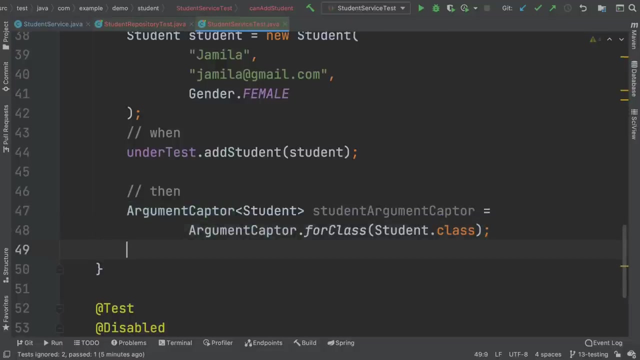 And this will be student, just like that. I'm going to call it student. argument capture equals to, and then argument capture, So oops, So argument capture for class, and then student- put this in a new line, just like that. So now what we want to say is: so here we're going to say: verify. 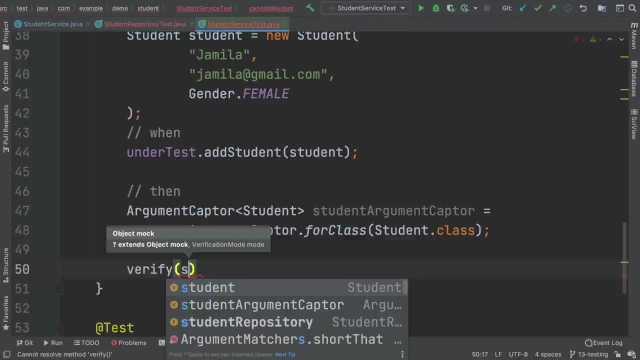 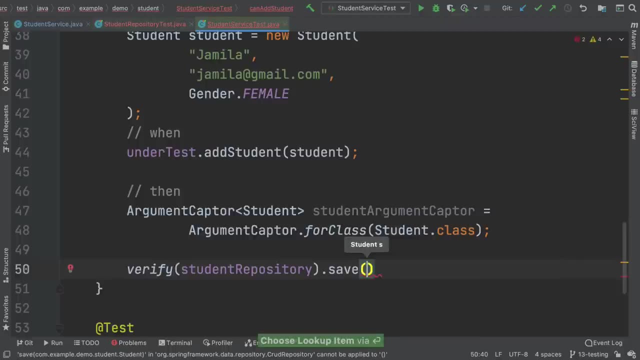 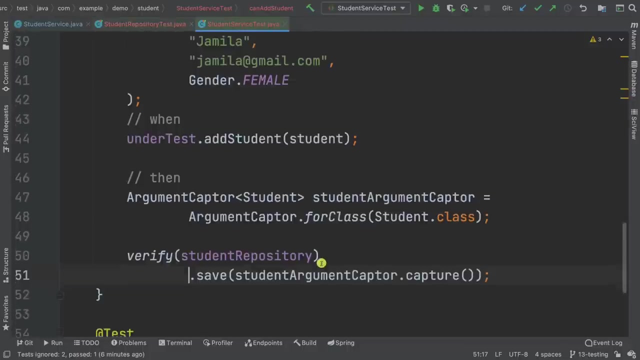 and then we want to have our mock. So student repository: dot and then save. And then here I want to say student Argument, capture, dot and then capture. And this might seem a little bit confusing, but the reason why we're saying right. 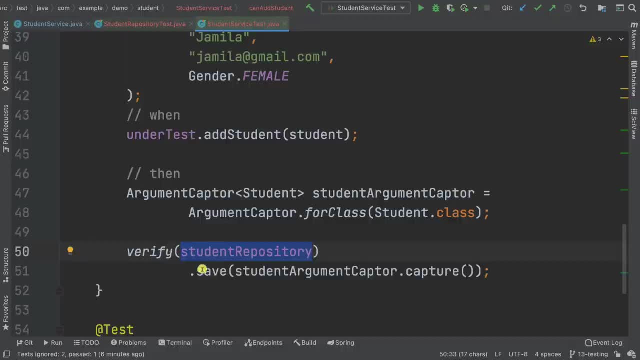 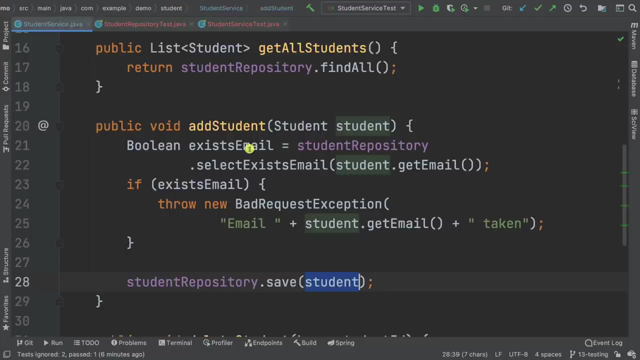 So we want to verify that the repository was called with save. But in here what we are doing, we are saying we want to capture the actual student that was passed inside of this save method, So in the student service. So here. So when we say repository save, we want to capture this value. 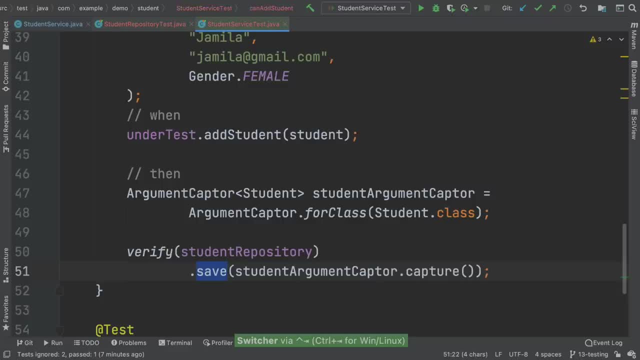 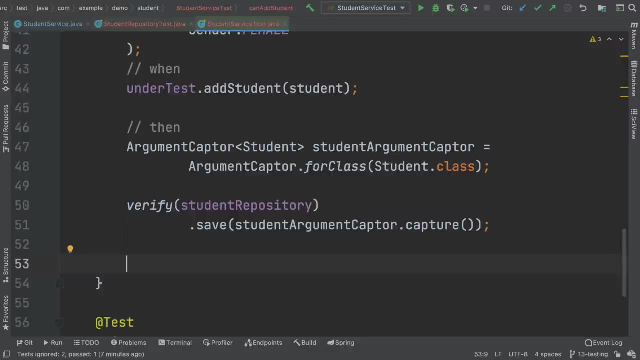 right here. So here let me just go back. And now the assertion that we have to do is the following: So now that we have the captured value here, using argument capture, we can say argument capture or student argument capture, dot, And then get and then value. 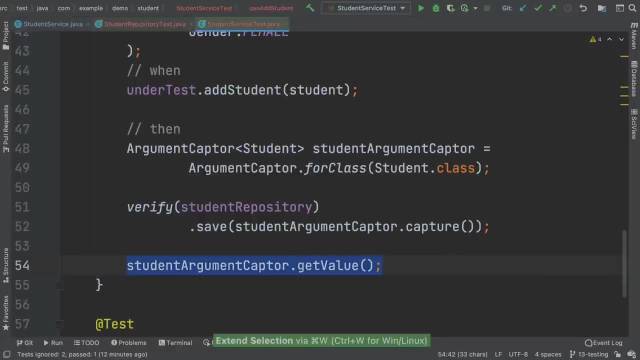 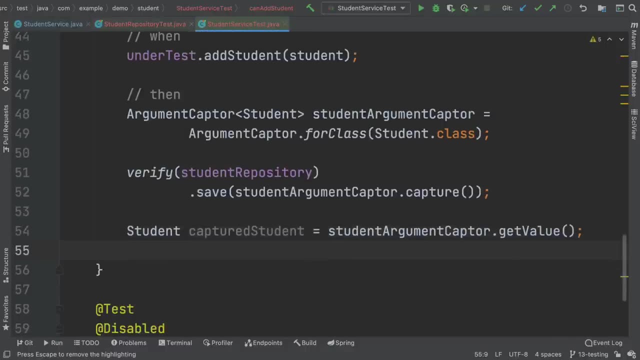 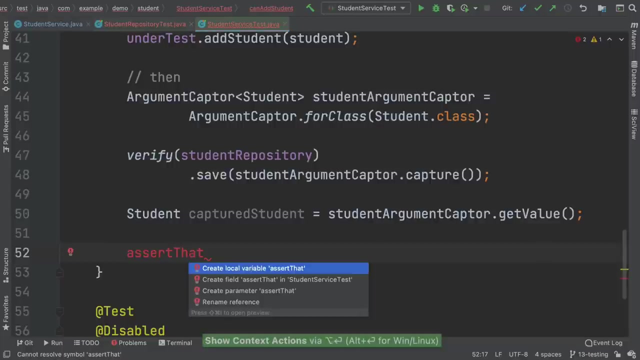 This will be a student, And now I want to extract this way variable. So this will be the captured and then student, And what we want to do is say, assert that, And then I'm going to press option and then enter, Or you can click on this bulb right here and then here. 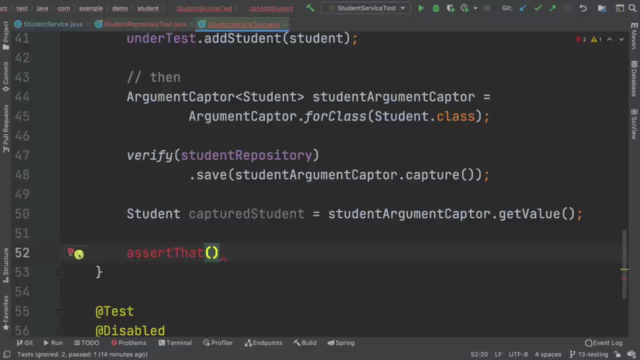 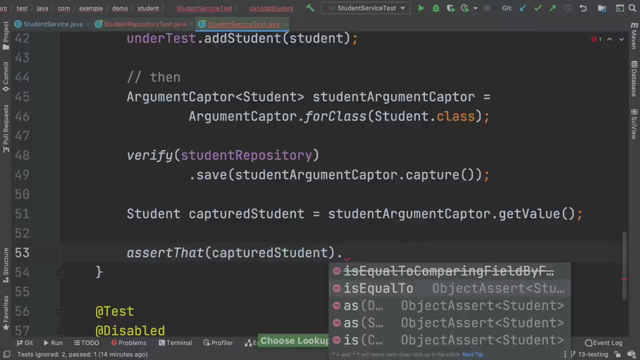 Actually we just need these parentheses so that this works And assert that. So import and then static method and then assertions for class types. So let's just pick that one And here I can say: captured student dot And you can see that before we used to use is equal comparing. 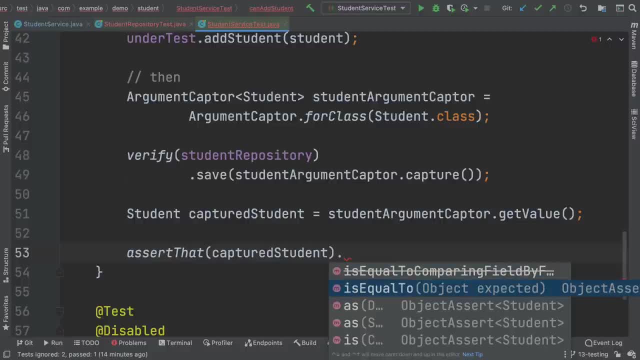 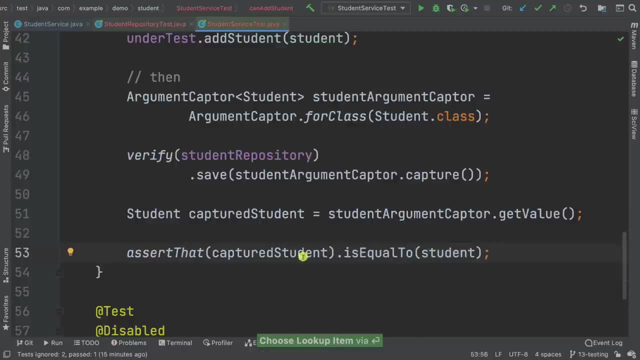 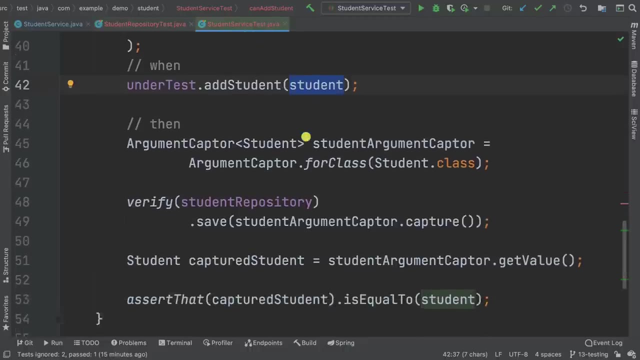 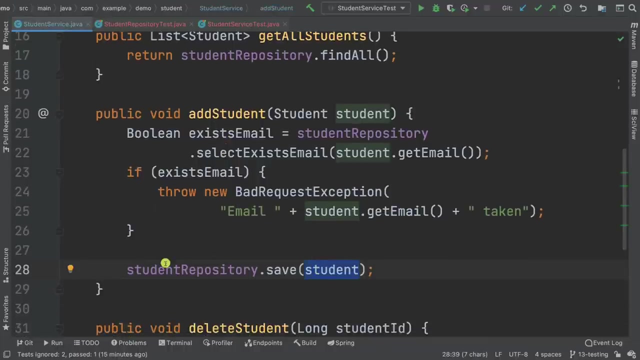 field by field, But now it's been deprecated and we can just say is equal To, and then student. So this student right here is the one that the end test receives, And then the captured student is what this service here receives. So the student repository save. 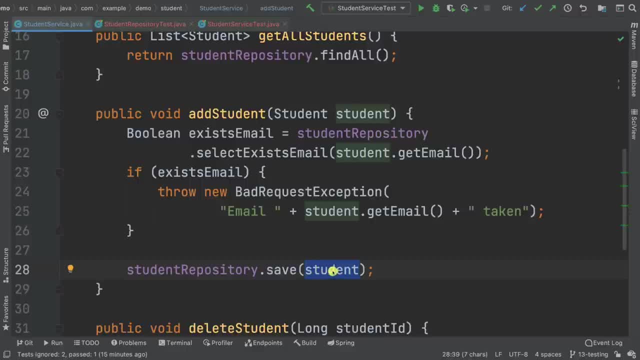 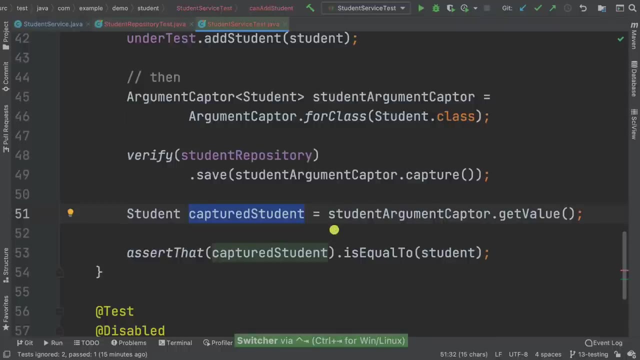 We capture this value And then basically we're just comparing that this student, what we pass in, It's the same one that the student repository save has been given as well. Now, if I go back to the test, and here let's run the test. 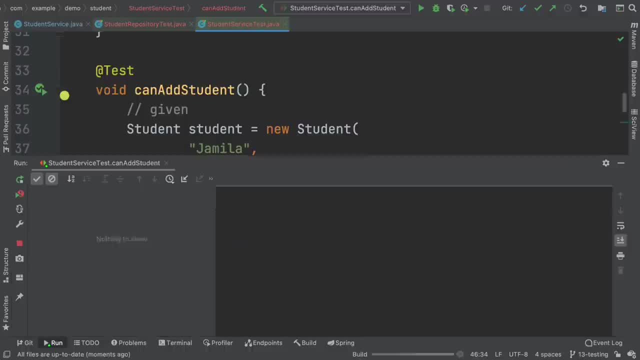 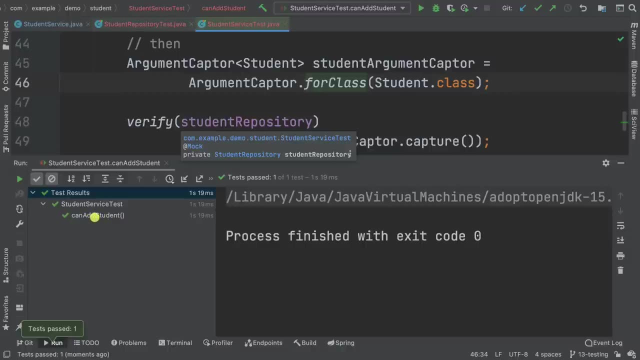 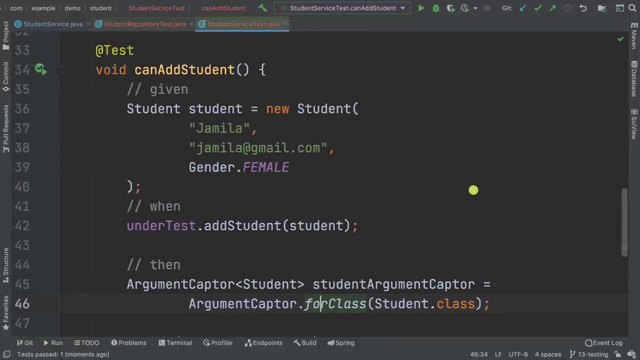 So here, just run this test And there we go. So you see that this test did pass, which is really really awesome, Right? So hopefully this wasn't too confusing, But But this is something that you have to get your head around. 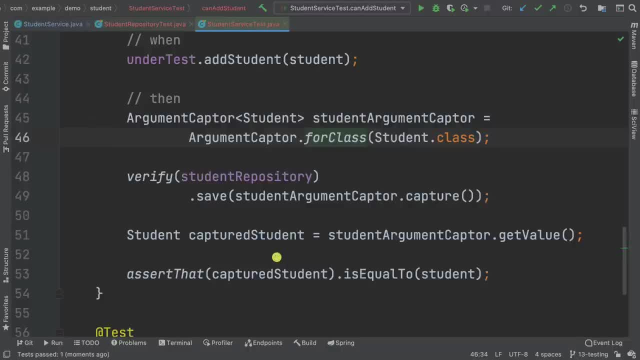 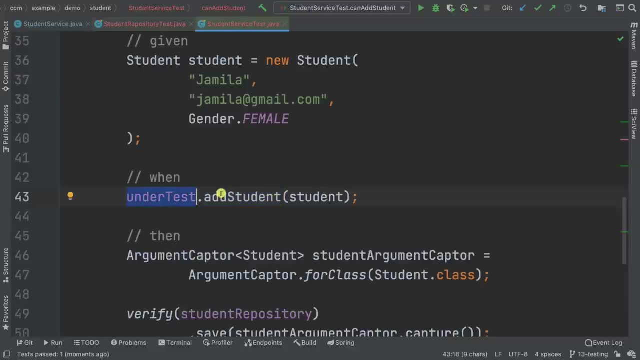 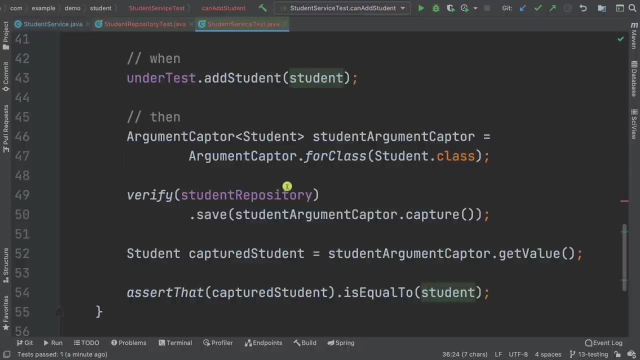 and make sure that you understand exactly what's going on. But, in a nutshell, we have the given And then when the end the test, though our student is given, this student right here, we verify, in here, So we verify that the repository and we actually capture the. 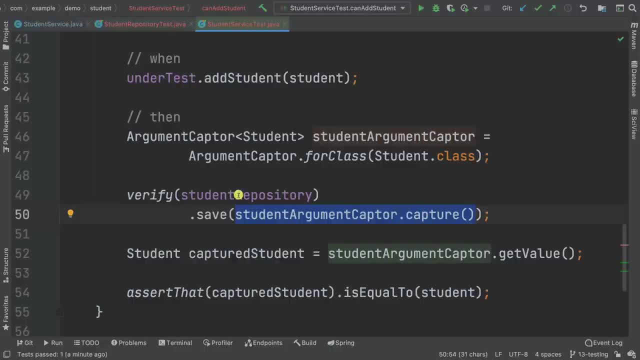 value. So we verify that the repository was invoked with the save method, But at the same time we capture the value so that we can actually make sure that the value is the exact same one which was invoked by the under test. If you have any questions, go ahead and let me know. next, 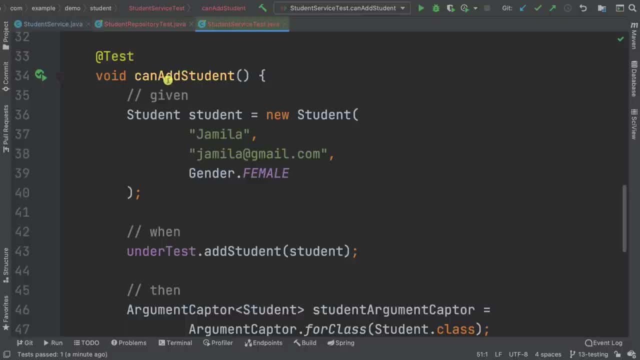 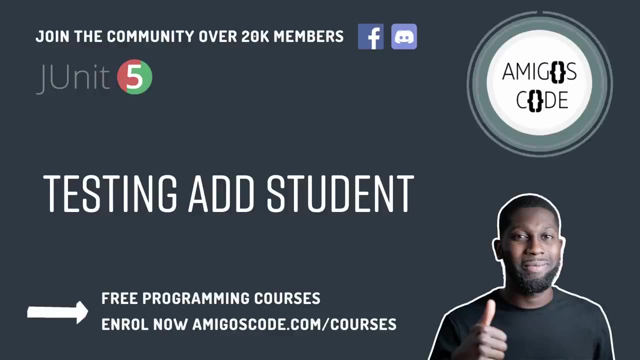 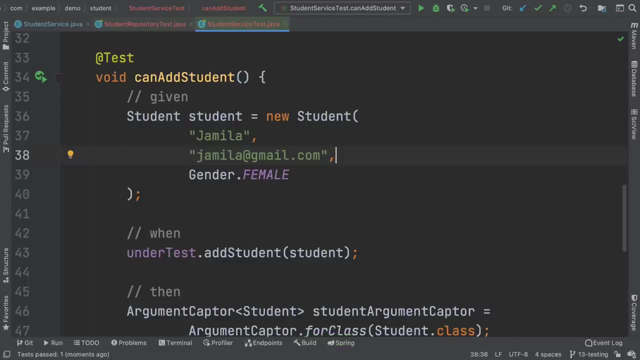 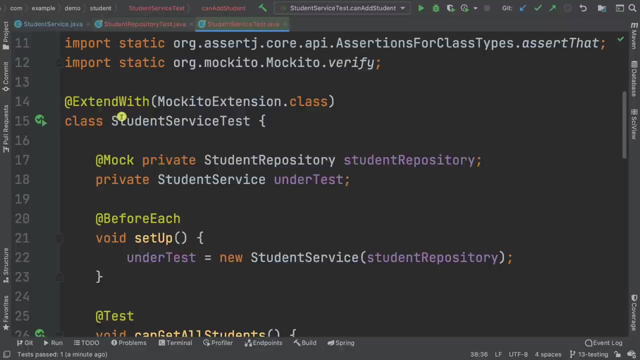 Let's go ahead and have yet another test for the opposite. So when the email is taken. Okay, Before we write our second test, what I want to do with you here is go to the top of this class and right click on this play button, right here or. 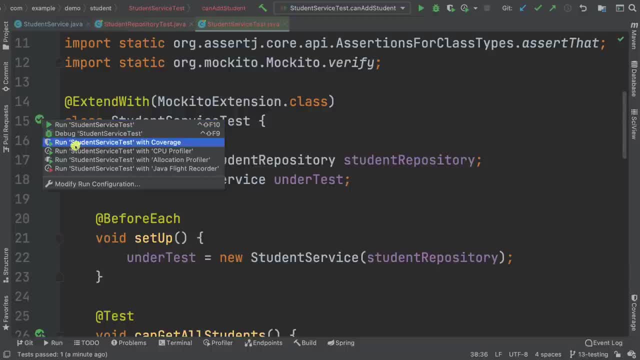 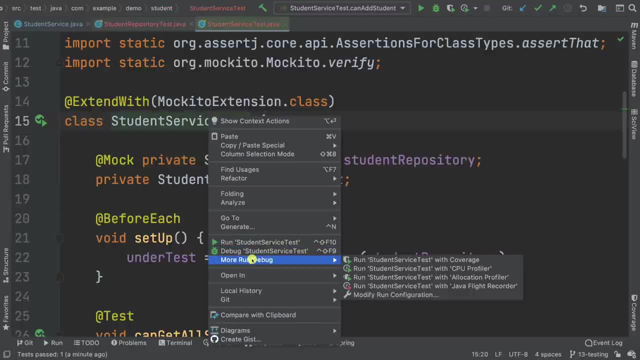 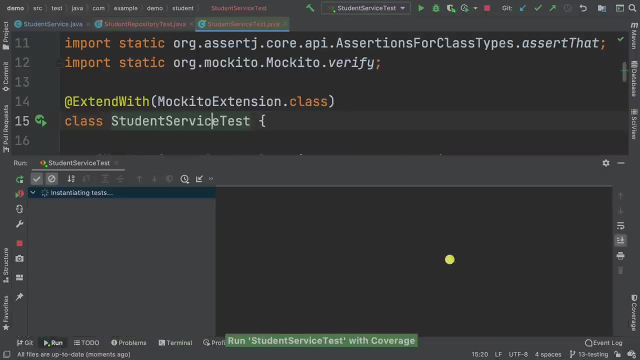 actually just click on it And then you see that we have run student service test with coverage. We can also achieve the same by right clicking, Go to more debug and then run with coverage. So let me just run with coverage and there we go. 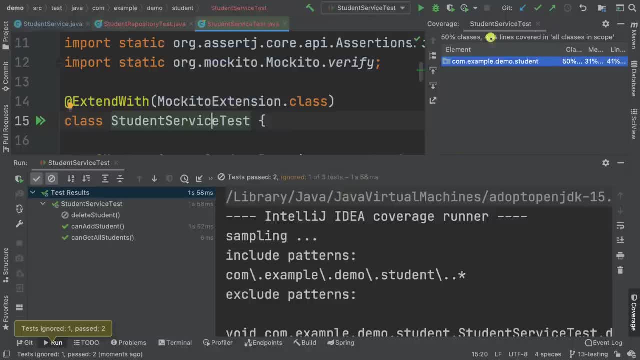 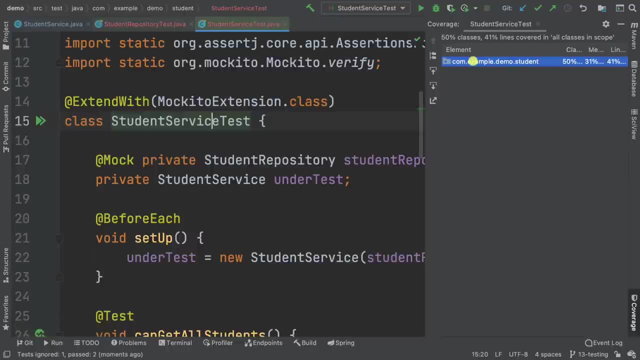 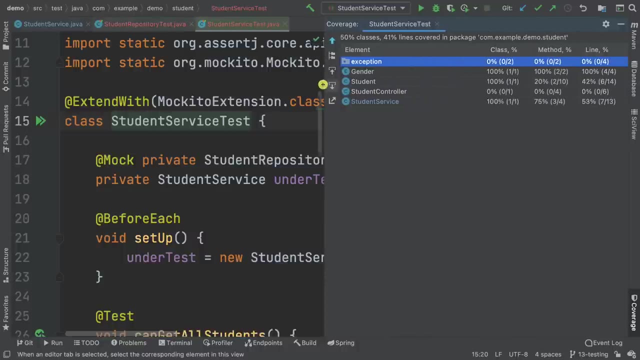 So you can see that we actually have this pop up right here And this is the coverage, And what I want to do is the following: So you can basically click on it and you can see that in here. So let's just zoom in a little bit. 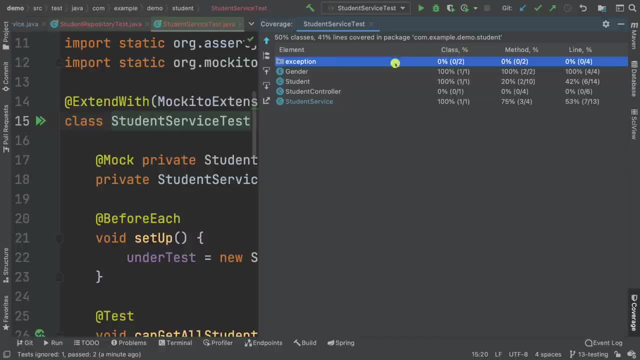 I'll actually expand this a little bit. You can see that we have- So this is the coverage, right. So the class student service, right here. So the class has 75% right here Coverage: The line coverage is 53%. 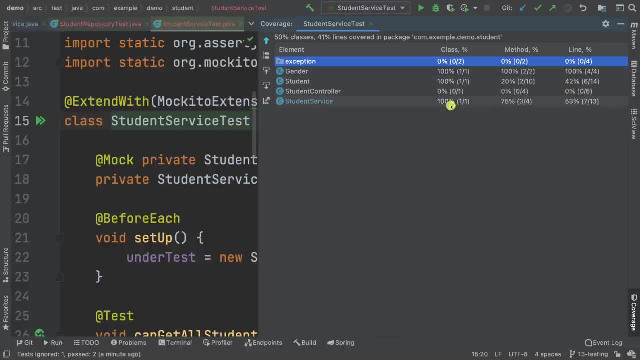 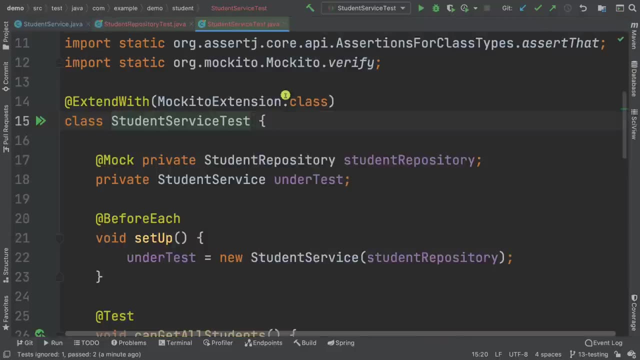 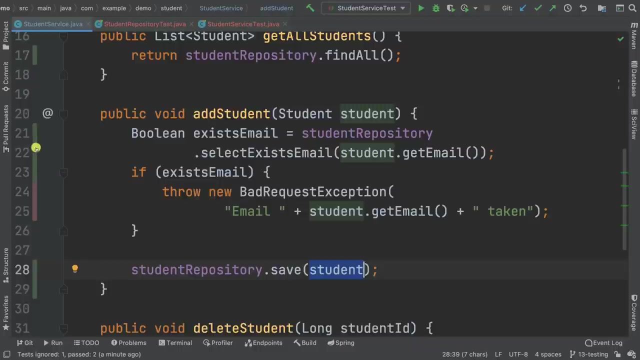 And then the rest. you can see we have some numbers here, but we didn't actually do much around this area, So let me just hide this and then go to student service, And what I want you to see now is: have a look, We have these lines. 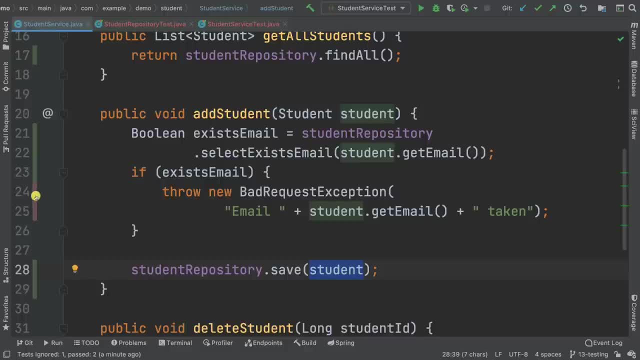 So green and red. So green means that this actually has been covered by our test, But red means that we are missing some tests. Yes, we are missing some tests, So we're not testing this scenario right here. Right, And this is what this coverage is telling us. 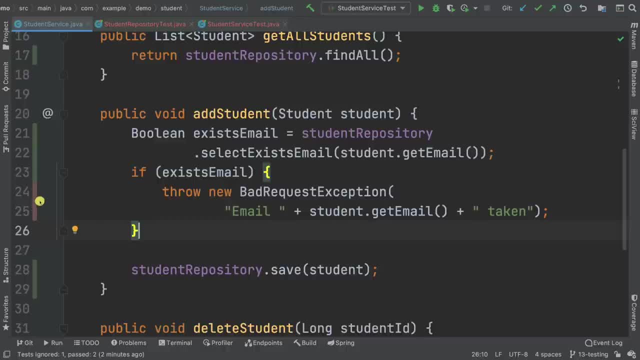 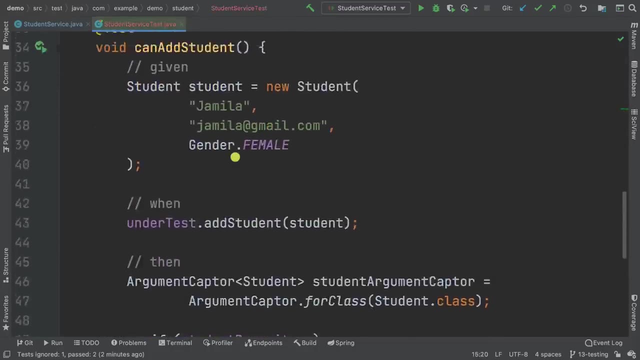 So IntelliJ is quite powerful and quite nice when it comes to testing and giving us information about what we need to test. So let's go back to the student service test in here And what we're going to do is test that when the email is taken. 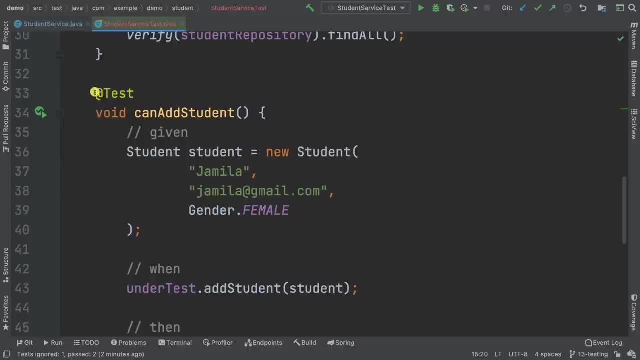 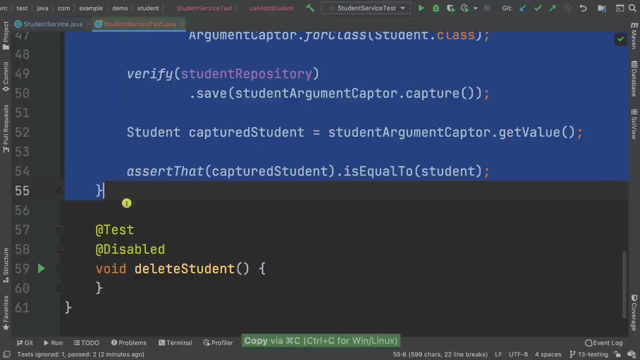 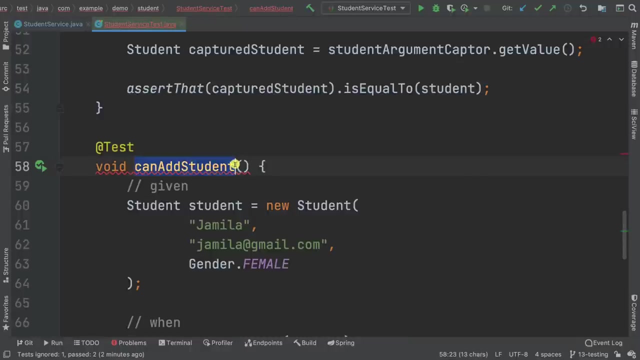 Our code will throw an exception. So in here let's just basically grab all of this, And usually we're testing. There's lots of copy and pasting, So paste that, And then we're going to change the name for So will, and then 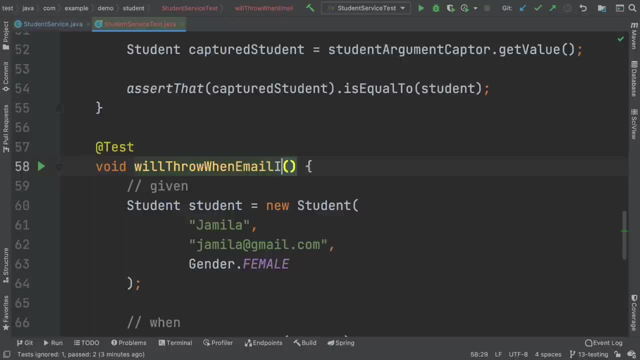 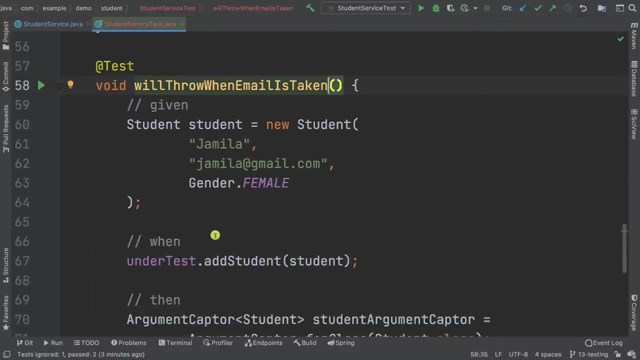 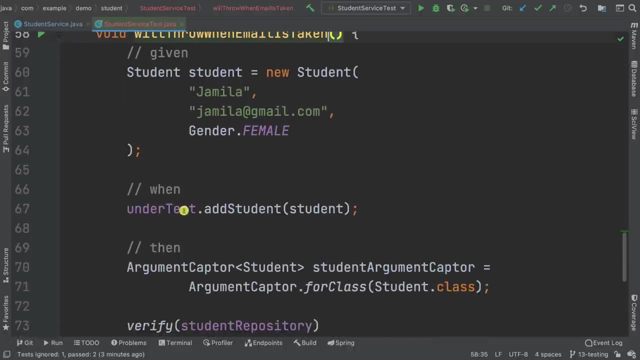 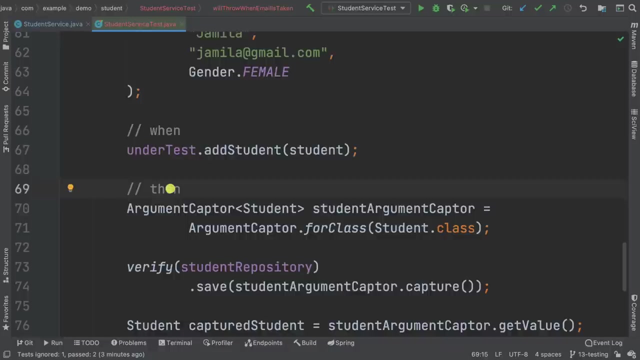 throw when email is and then taken. So here's what we're going to do. So this will be the following: So given the student and then when. So when this is called, we want to make sure that we have an exception being thrown. So this will be combined. So when and then. 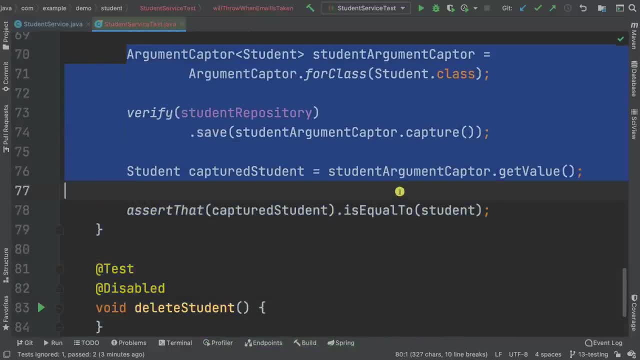 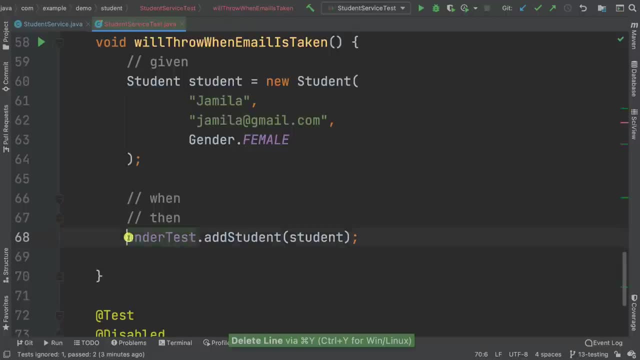 and at this point we can actually get rid of all of this. So just like that and that as well. So now with a search we have a set and then thrown and then by- And here should be assert, And then that and then thrown by. 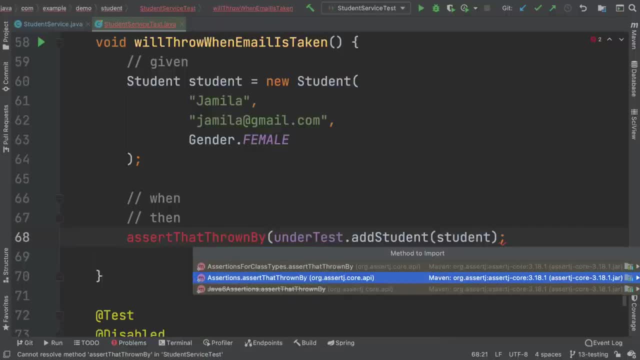 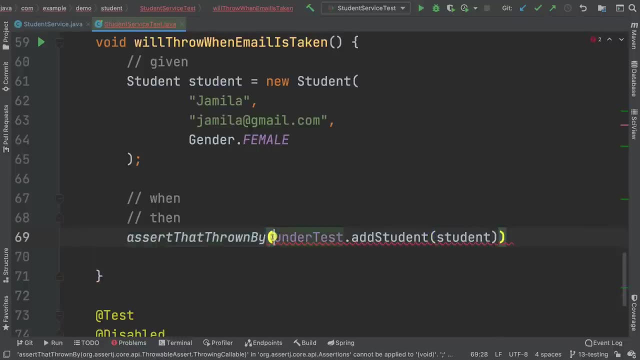 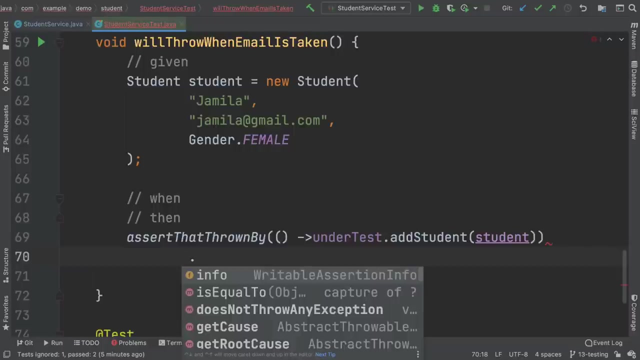 So import static And this will come from assertions And in here. So this works as follows: So this takes a Lambda, just like that, And then here we can say that, and then has, and then message, And we can say has. message containing: 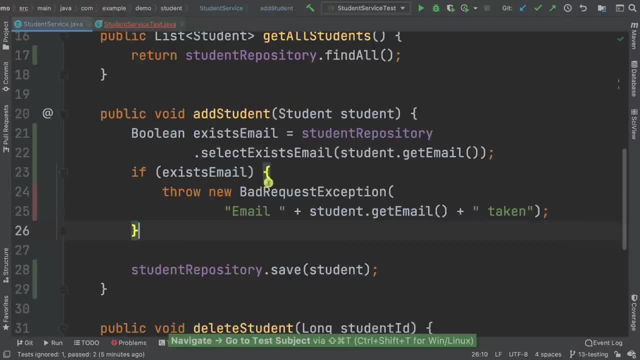 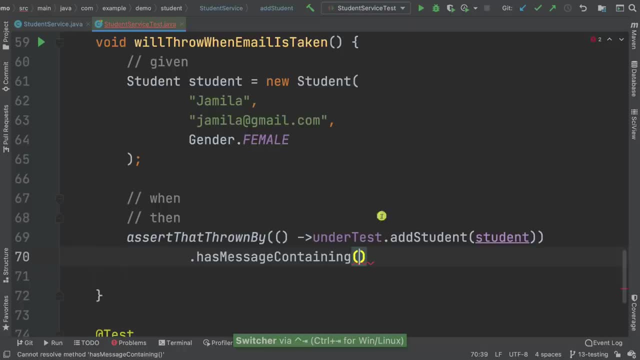 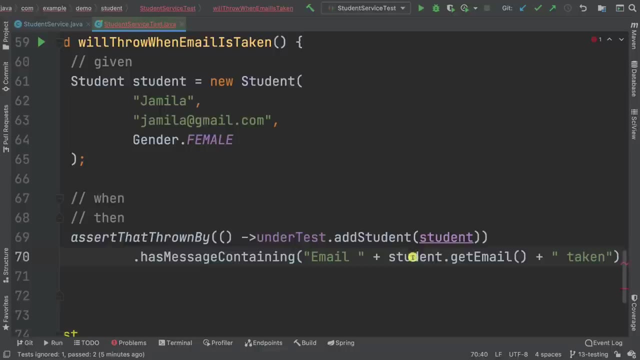 And basically. So if I go back to the actual test, so this is the message, So email, And then this is taken, So let's just paste that And then here I'm going to say that And this will be student email. So this is basically Jamila. 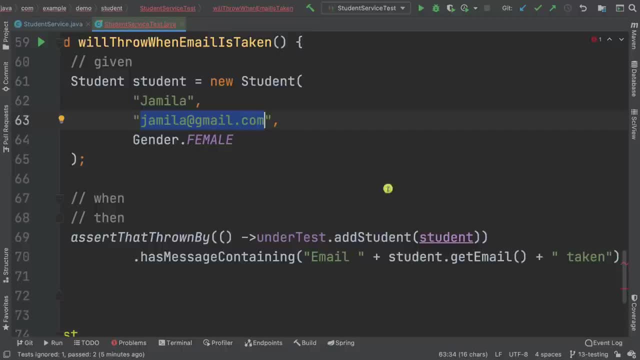 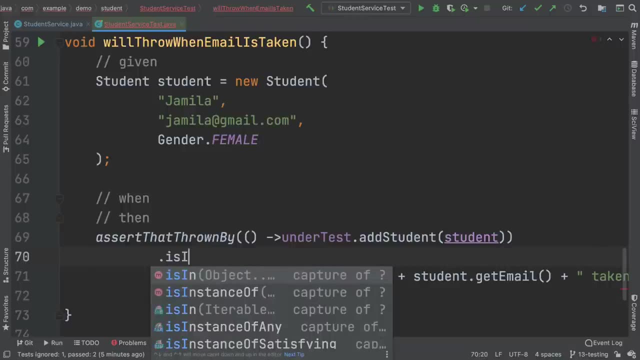 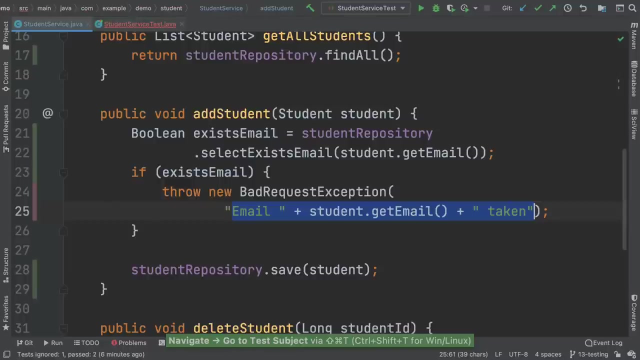 Right. So this email right here And also we can say so before that, we can say: dot is and then instance of And if I go back again to the basically shouldn't service bad request exception, So let's just take that, paste that dot and then class. 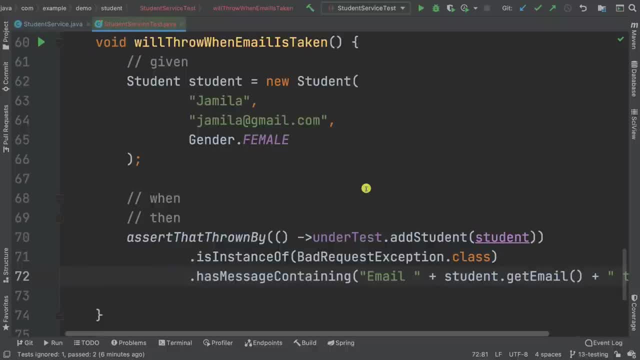 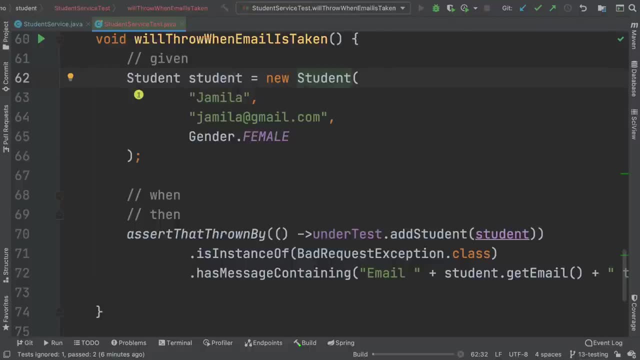 And there we go. So, basically, this is what we want to test, Right? But now, if I run this, I want to show you that. So let's just run this. This will not work, And you'll see why in a second. So there we go. 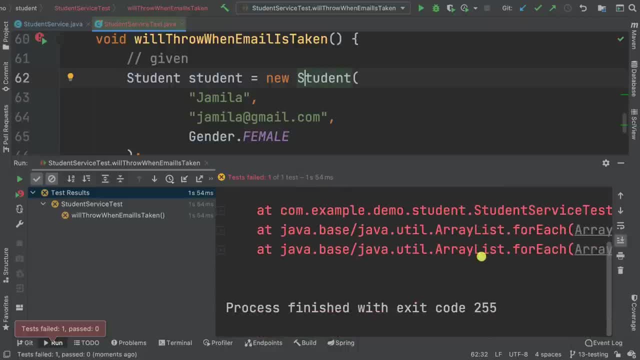 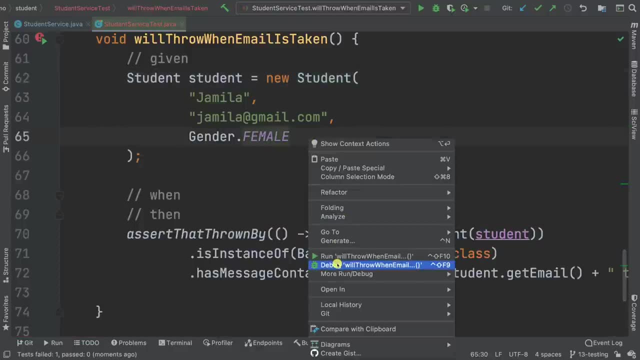 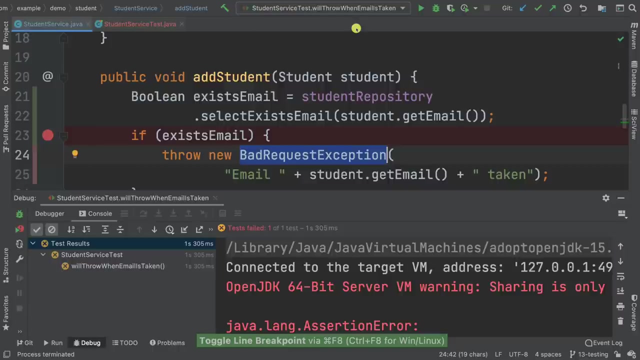 So expecting code to raise a throwable, But what is happening is. so let me actually just run this in debug mode. So debug, And let me go and put a break point just here, Right, So let's debug again, And this will make sure you understand exactly what's happening. 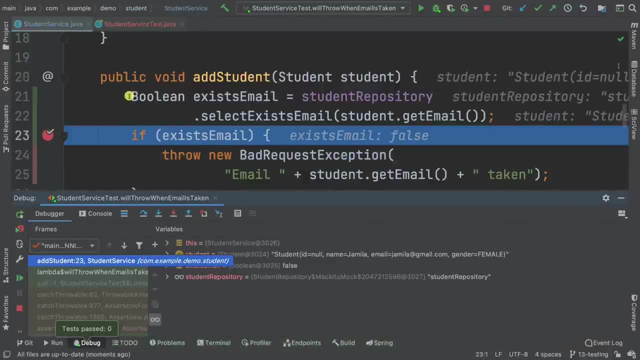 There we go And have a look, So Boolean, and then exists email. So this exists email is false. Right, This is false And we want it to be true, But currently we're not telling our mark that when this method is called with 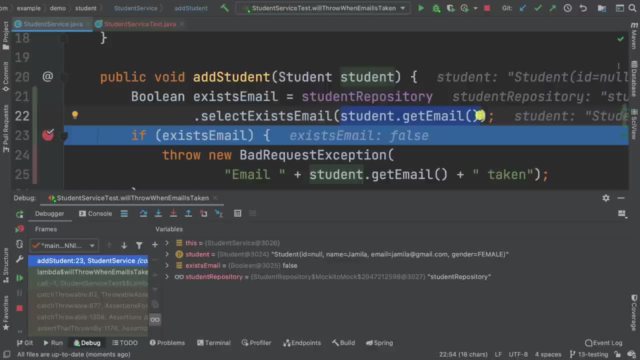 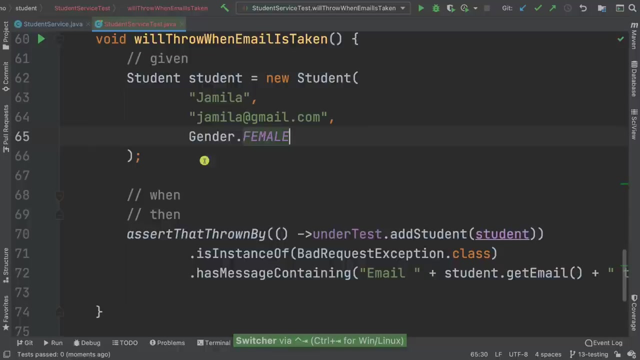 this email, or any given email, to return true. So by default, if you don't specify a return value, it will just default to false, which is our case. So let's just stop this and then go back to the test, And in here what I want to do is say: given 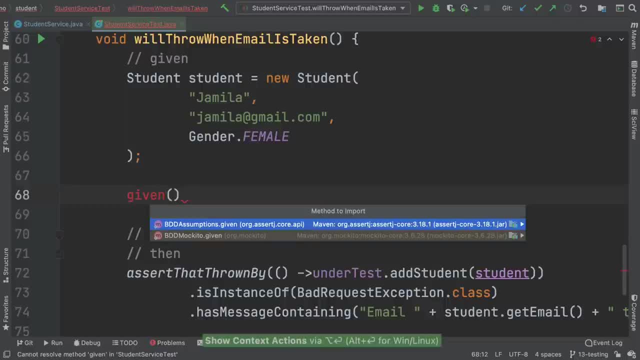 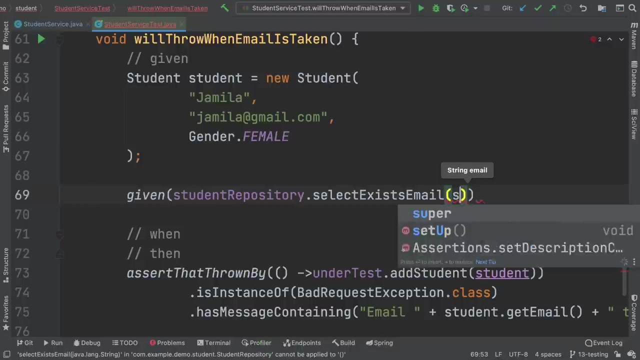 And here let me just import the static method, And this will come from Mokito. So BDD, Mokito given, And here I'm going to say student, repository dot, and then our method, So select, exists, There we go, And then we can pass the email. So here I'm going to say student. 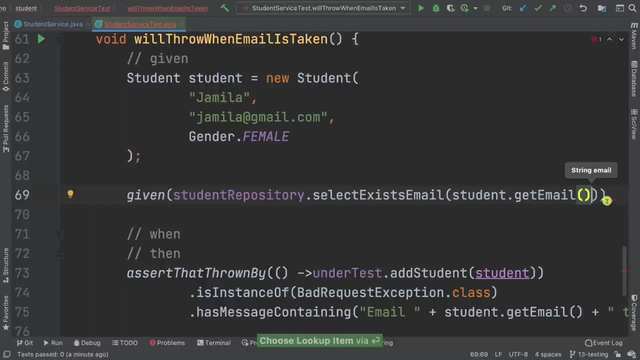 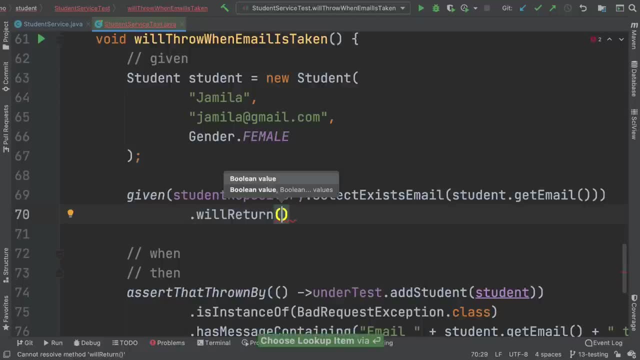 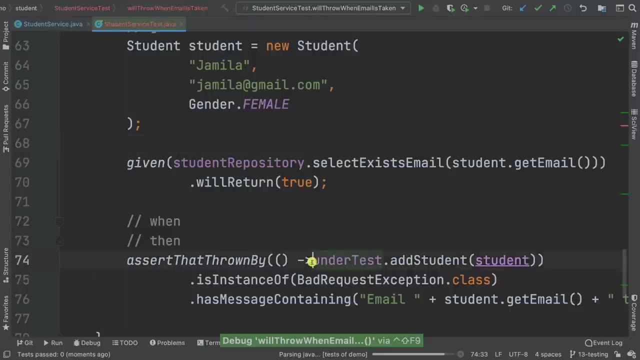 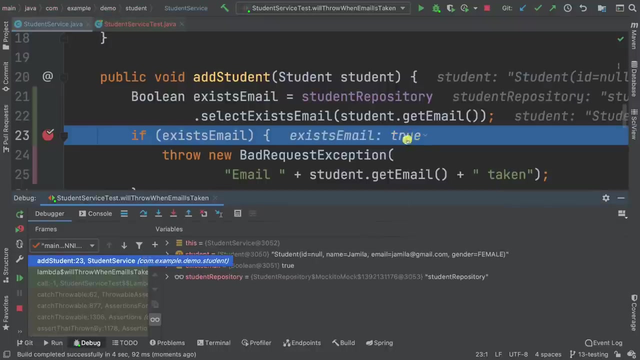 dot get email And after this I want to say dot will return, return And then the boolean value, which is true. So let's run this again in debug mode And now check this out. We said true, And which means that this will fall inside of this. 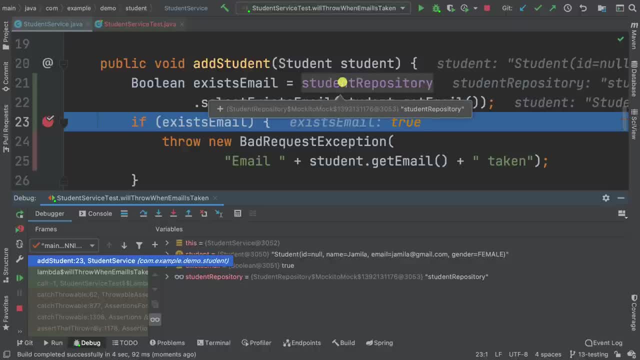 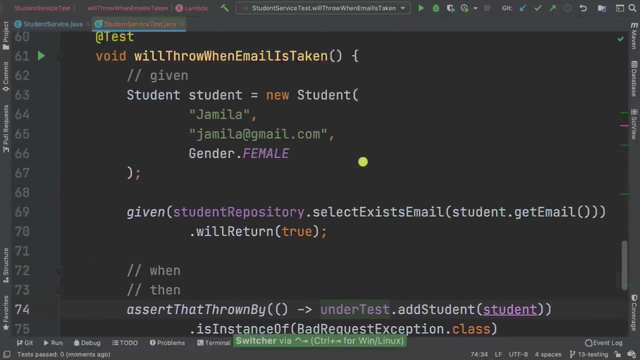 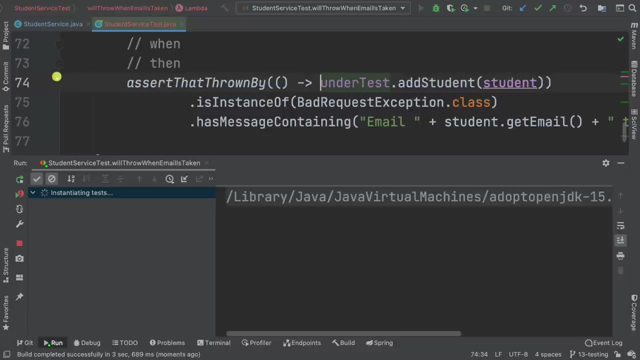 if statement. So now we are controlling exactly what happens when this select exists. email is invoked. So let me just close this, or actually stop this. And then here let me go back to the test and we can run the test. And there we go. You can see that the test did pass. 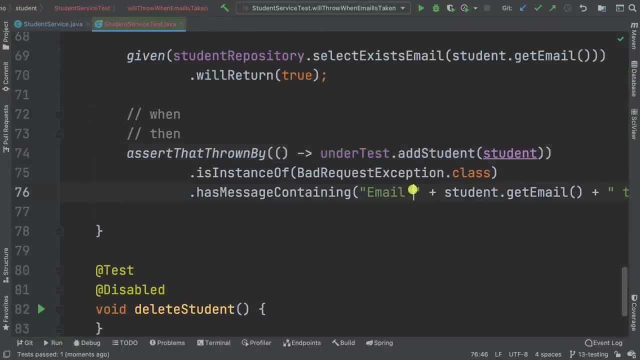 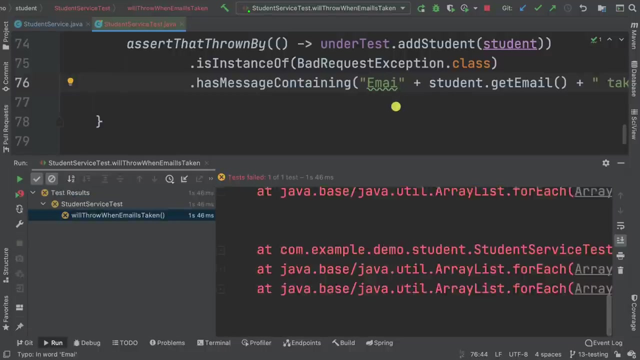 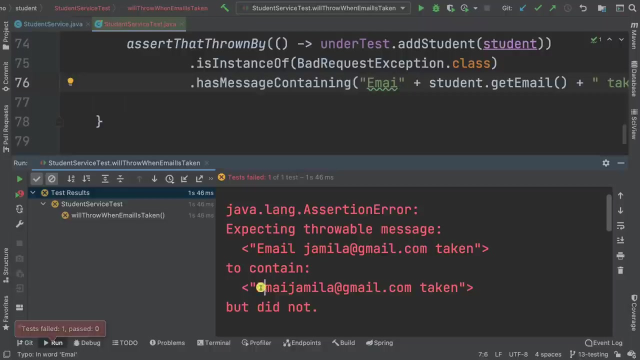 Now here I could also say: let's say that I do have, for example, basically I said email, Right, So if I run the test again, this will fail, And there we go. So you see that expecting trouble, message, email, Jamila taken, And then basically this: 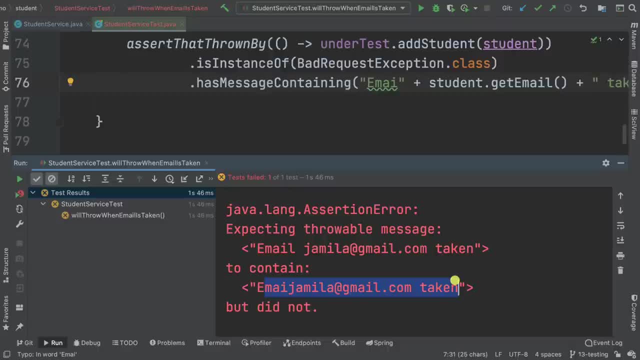 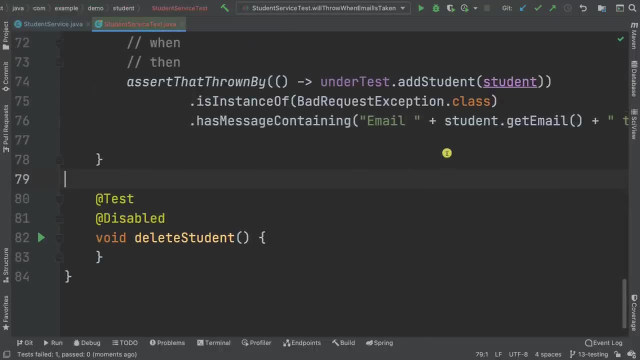 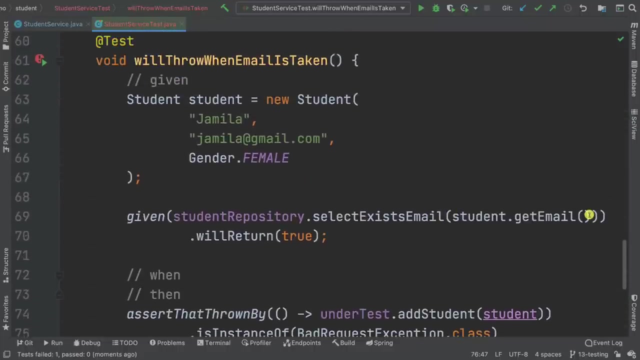 was what we are expecting Right, Which is incorrect. So I just want to show you that this is actually working. So email and then space there, and we are good to go. So one thing here also is: what you can do is, if you don't want to pass. 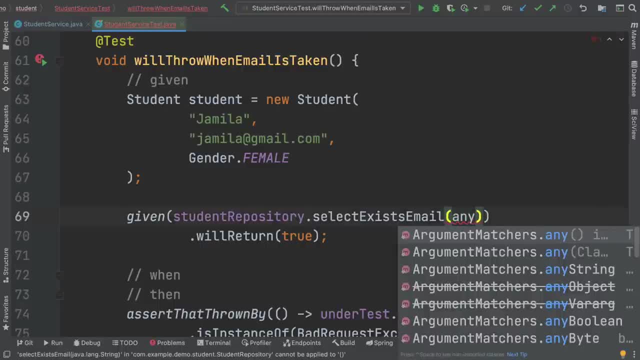 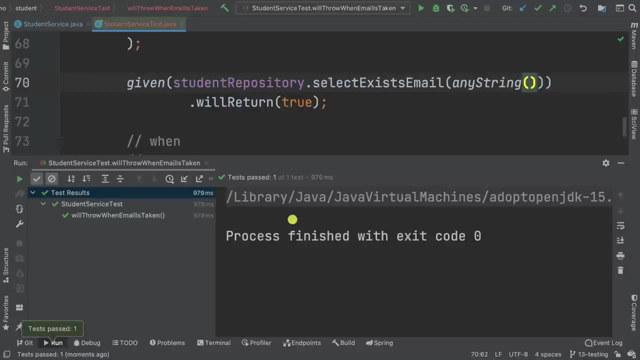 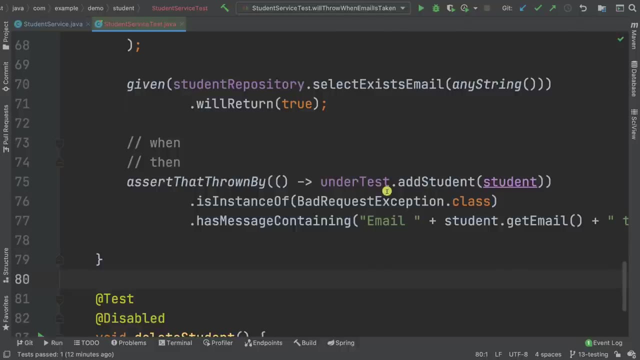 for example the email. here you can say any and then string. So if I run this again, you can see that this works. And there you have it. Finally, one little improvement that we can do with this test is that right here you see that we are asserting. 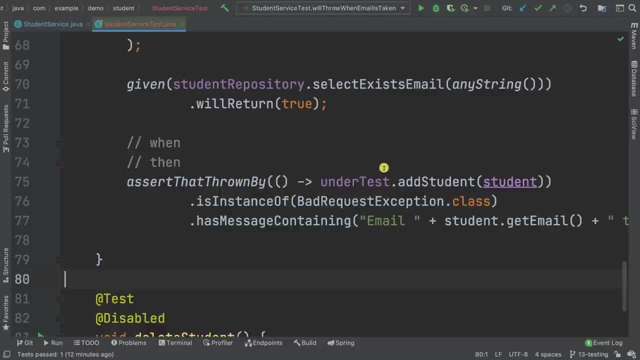 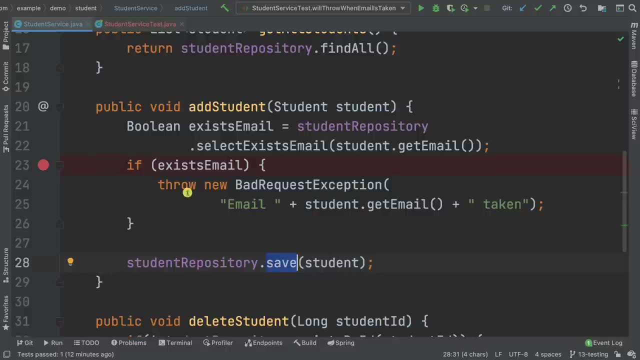 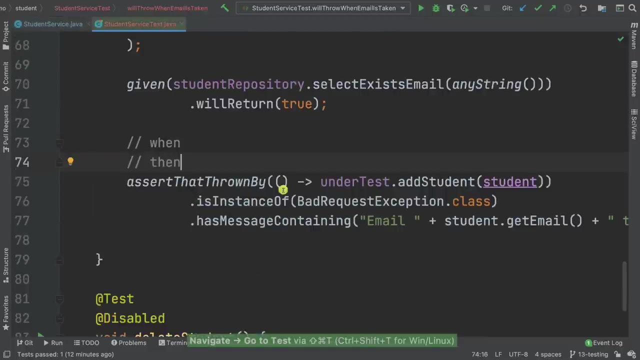 that thrown by, which means that if I go back to the service in here, this method is never called Right Because we throw this exception right here. So let's go ahead and actually reflect that in our test. So here, after this line, right here, I: 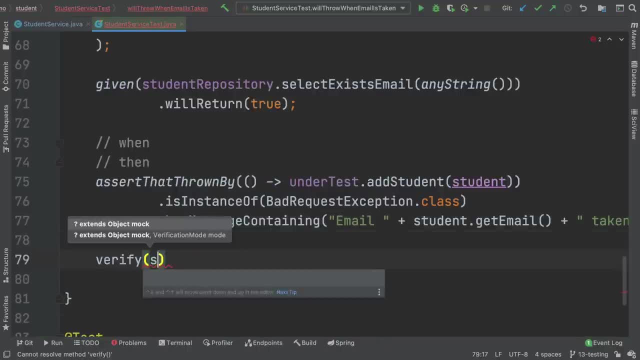 can say verify, and then I'm going to pass the mock, So student, and then repository, And then I'm going to press comma in there and then the verification mode, So this will be never dot and then save, And we can say any. So just like: 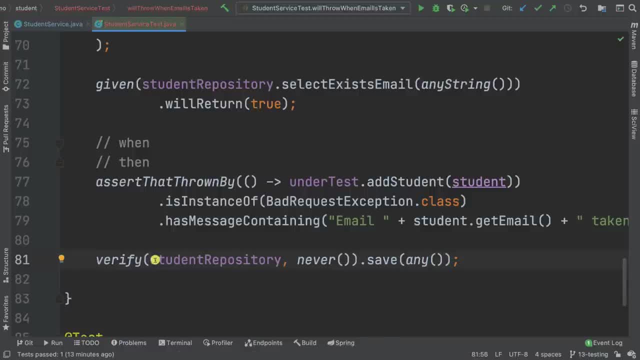 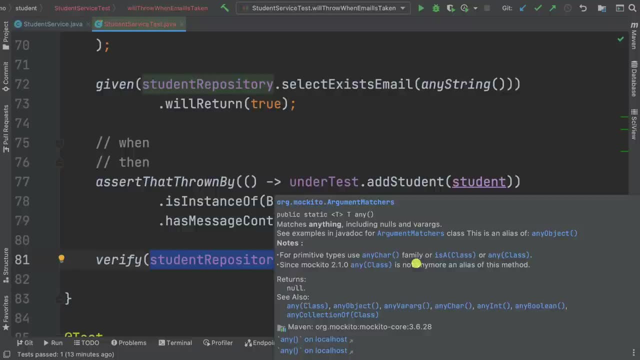 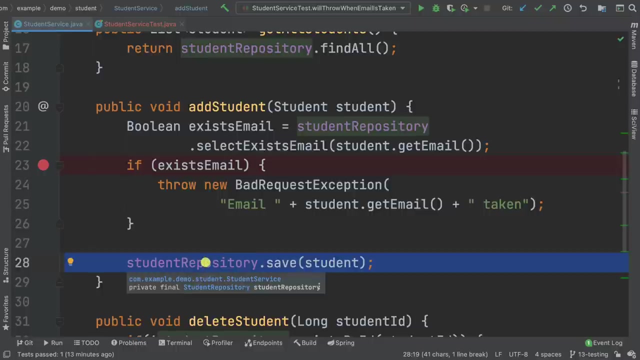 that Right. So we are saying that this repository right here, So our mock, it never saves any student. So again, if I go back to the service in here, you can see that this method right here, it's never executed, And this is what I'm actually saying in here. 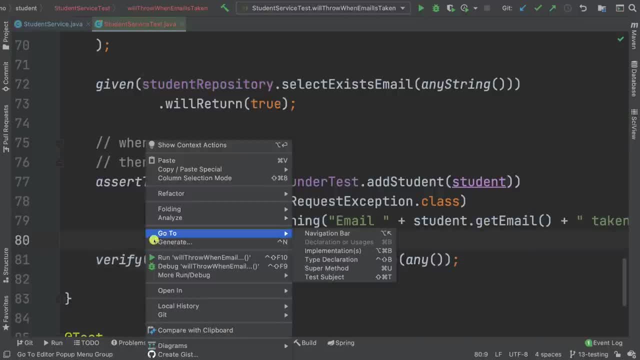 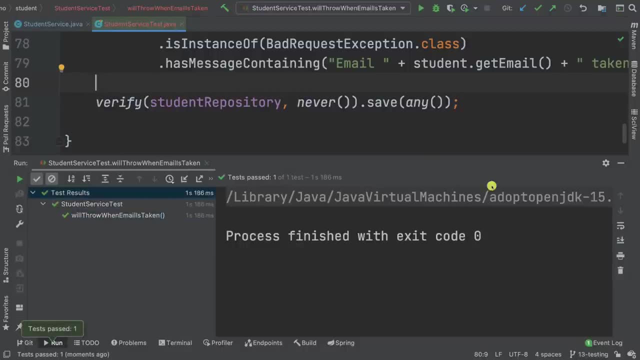 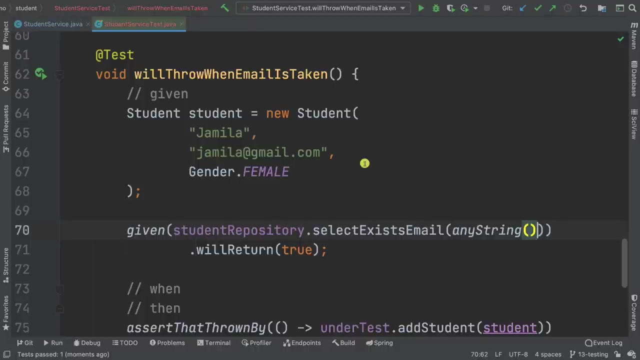 So if I run the test again and you can see that this also works now, if I collapse this and then scroll up, So the final thing that I want to do is let's run this class right here. So here we're going to run this. 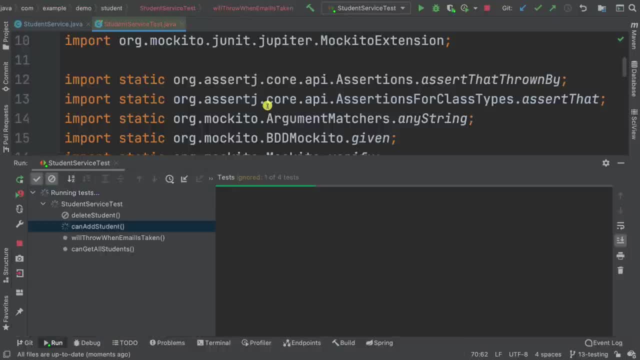 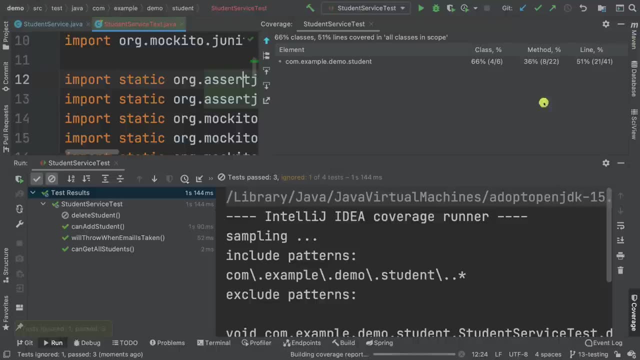 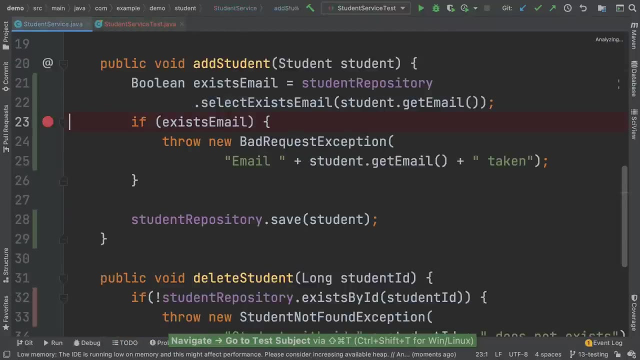 with coverage. There we go And let me collapse these stats in here and then close all of this, Go back to the actual service class And now you can see that before this line was red, But now it's been covered by our test, which is really, really cool. 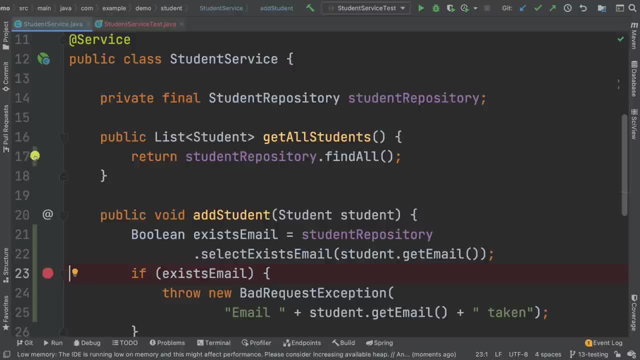 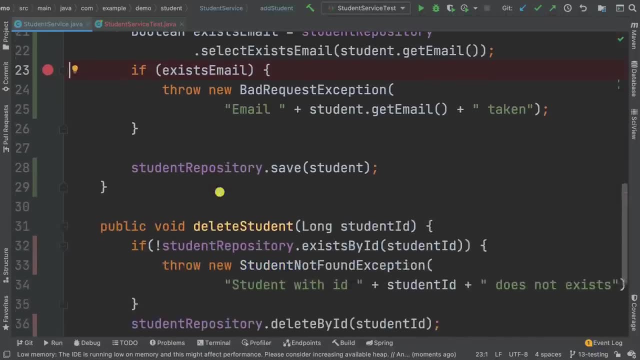 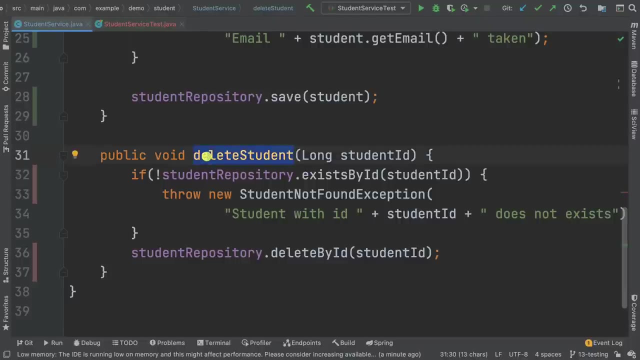 So there you have it, And also you can see that we have covered this test right here. This test is fully tested, Or actually, this method is fully tested And the only thing that we have to do is actually test the lead student. This, in fact, will be an exercise for 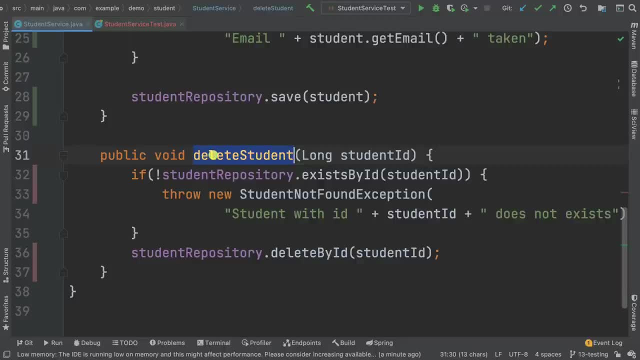 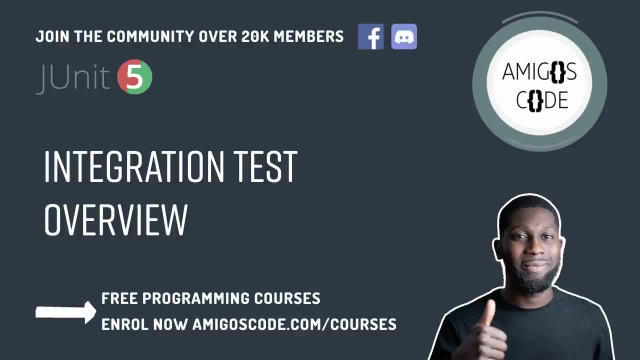 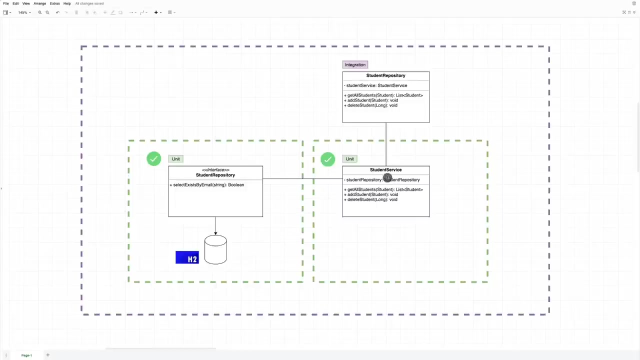 you Go ahead and implement the tests for this method right here, called the lead student. Now that we have the student repository and student service, both fully tested, now we can go and learn about integration testing. So, as I said before, unit testing it's about. 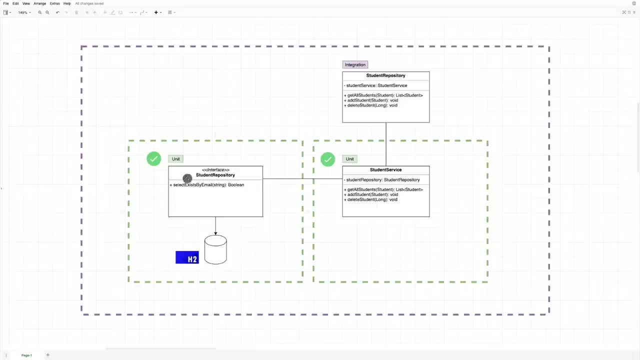 the unit itself right here. So we test it in isolation. So you saw that we tested student repository in isolation, all of the methods. Then when we tested it within student service, Right So because here you see that it's a private field for student. 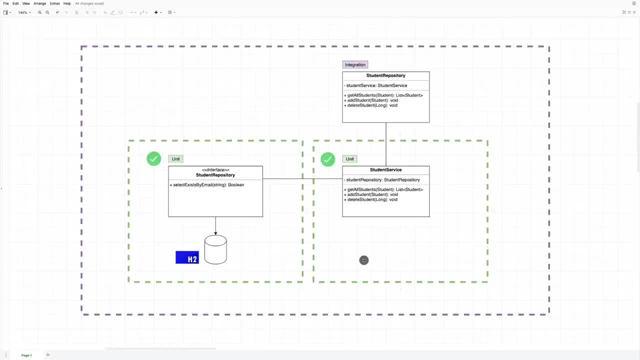 service. We mock this interaction, which means that we also tested this student service in isolation. Now, integration testing is when we test our application as a whole. So you can see the boundaries here, right? So the purple boundaries. So, basically, instead of testing the unit itself, right? 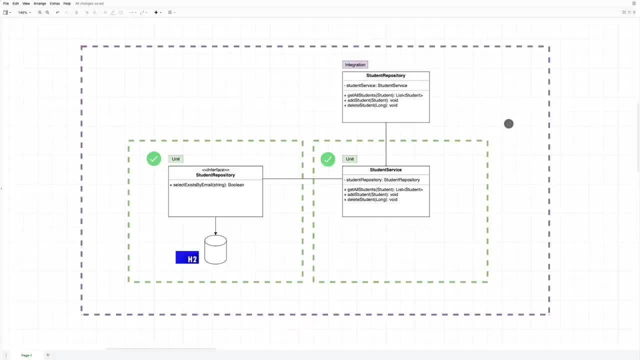 here we test the application as a whole. So what we do is we actually spin up The application and then we make sure that the integration between all of the components within our application does work. So it means that we actually fire a request into the repository making. 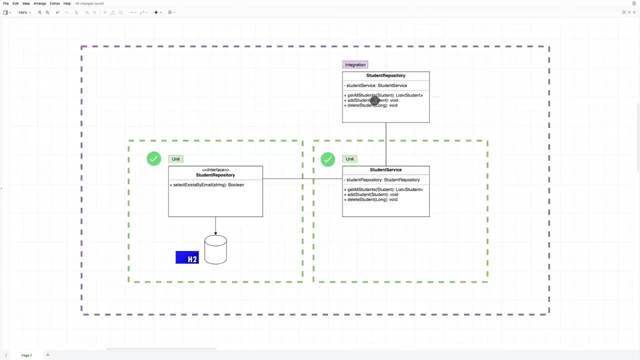 sure that the API layer is intact and then letting the request flow through the system to make sure that it does indeed work. So we no longer need to mock student service. no student repository, Because this is an integration test. So let's learn how to perform integration tests within our 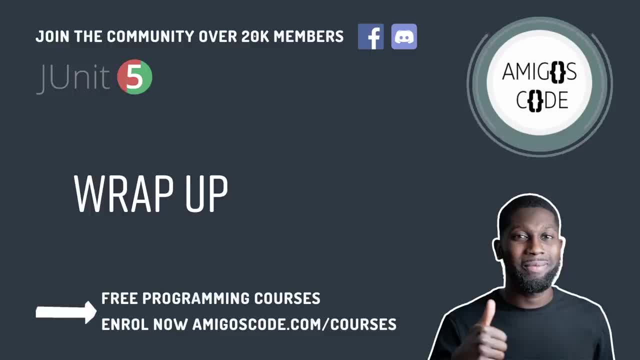 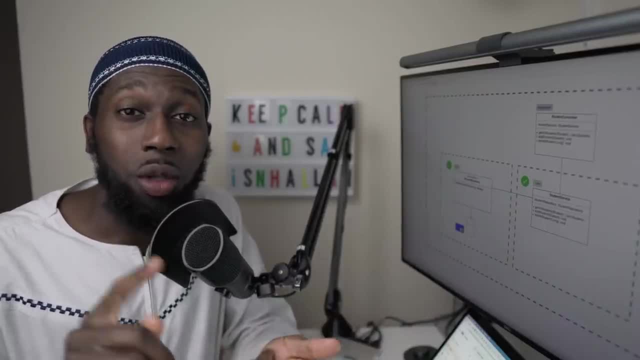 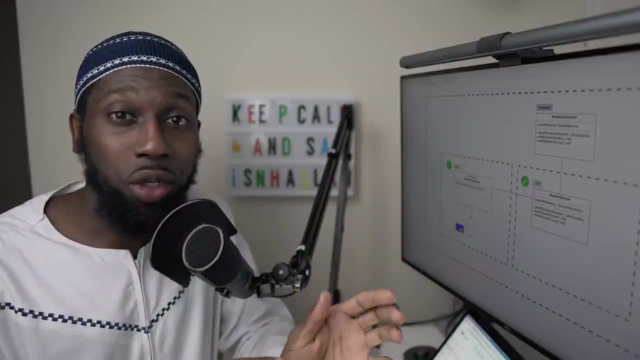 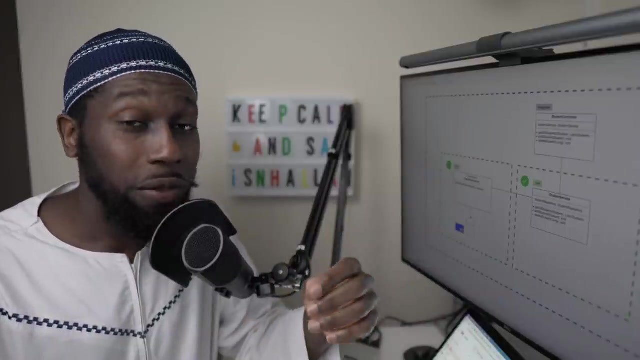 application Right. So we've covered quite a lot, to be honest, unit testing, mocking, and you saw how we tested each unit in isolation And yeah, so it's not really difficult to be honest Once you understand exactly how things are put together. 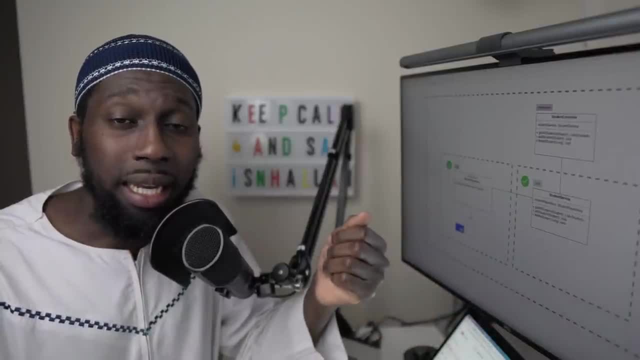 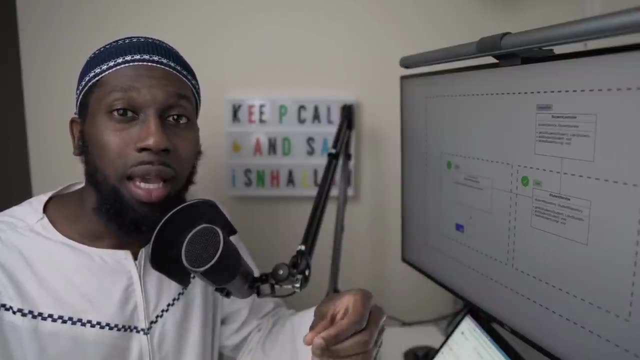 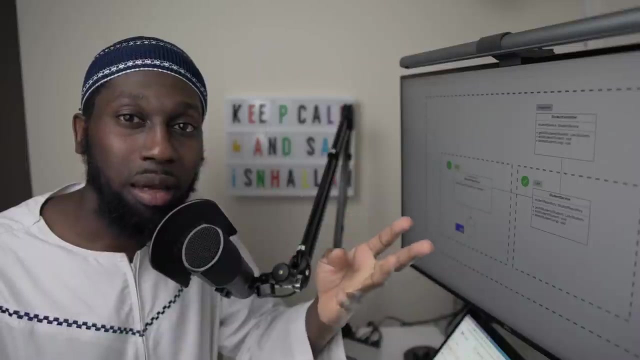 we've just scratched the surface- I got to be honest- And next what we need to do is actually focus on integration testing. So this is where you spin up the application and then you test your API endpoints Right. So if you have get requests put, delete and post. 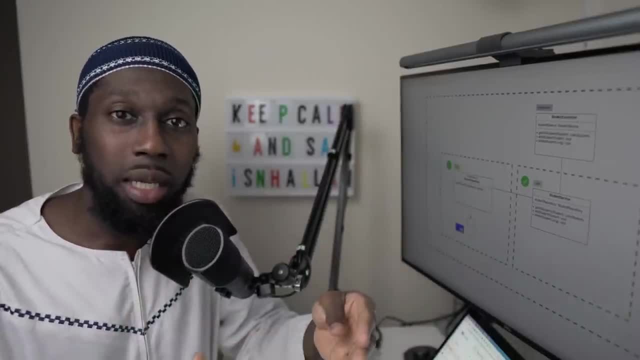 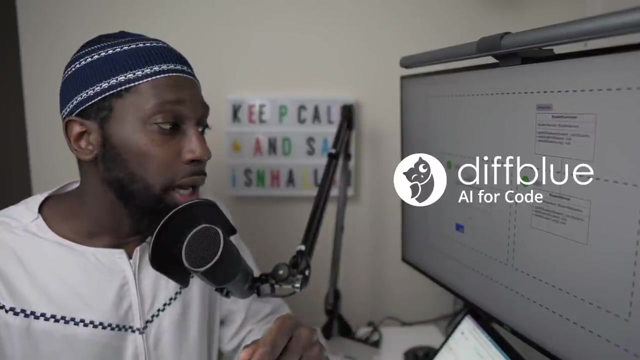 then you want to be sending real requests against those endpoints and making sure that the request goes through the system and then does what it's supposed to do without breaking anything. So also the sponsors of this video, Diff Blue. they have this awesome integration where you can pretty much just 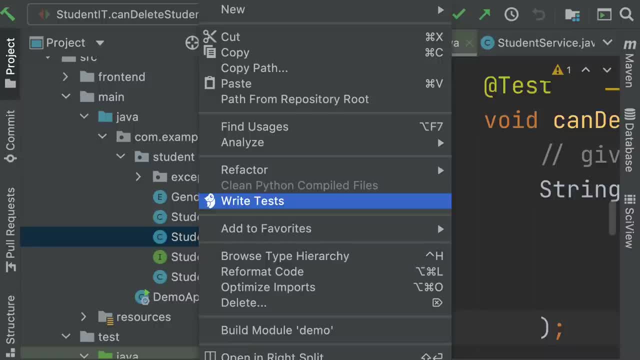 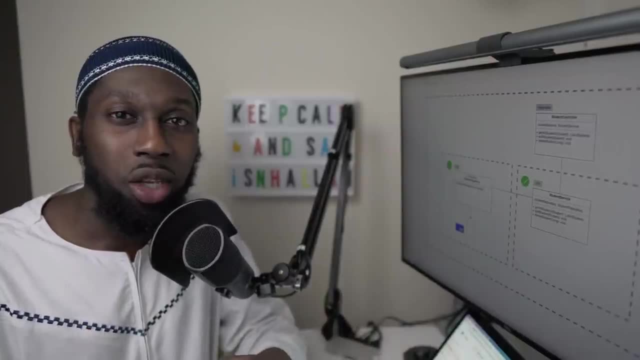 right click and then you can generate a test for your controllers, which is really, really nice. Now, if you're serious about becoming a software engineer, then I do invite you to enroll to both the Spring Boot full stack and react, which this crash course. 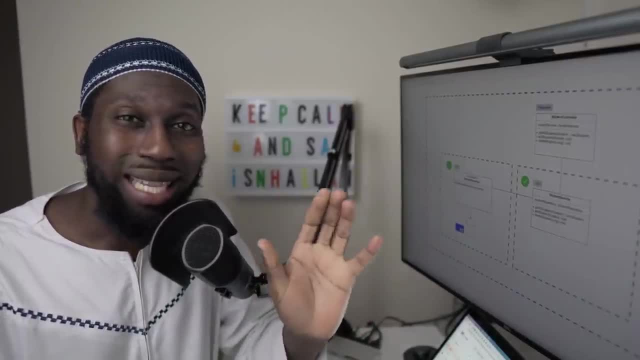 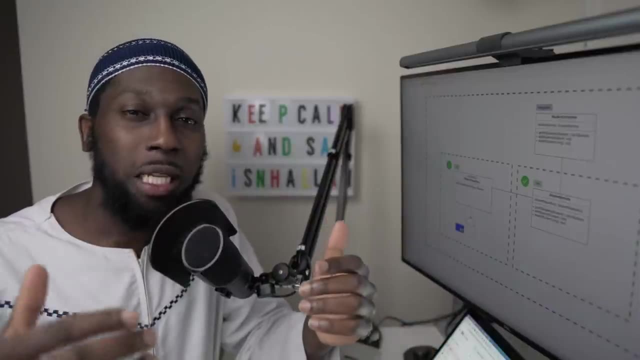 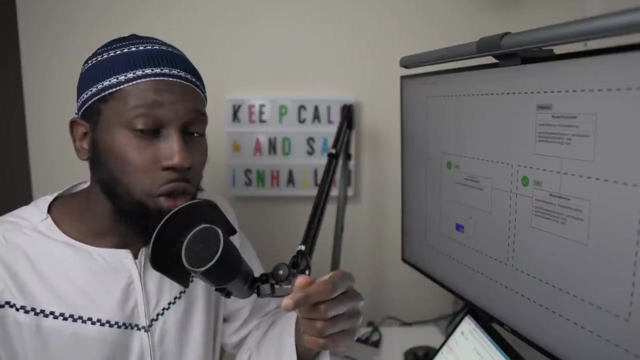 is a mini series of it, And also I've got a course just on testing, So making sure that you understand the overall picture Right. So this is where you learn about testing. You learn about mocking, how to properly write integration tests, And also I'm going to show you when you have, for example, external 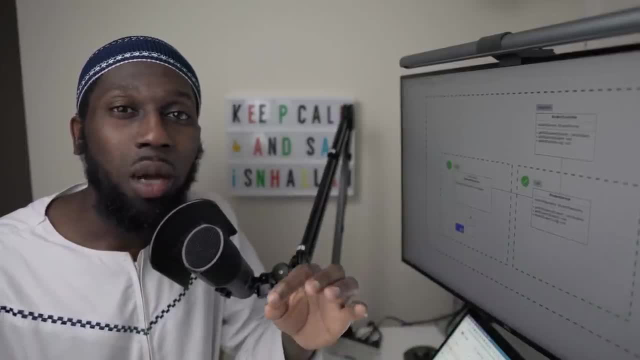 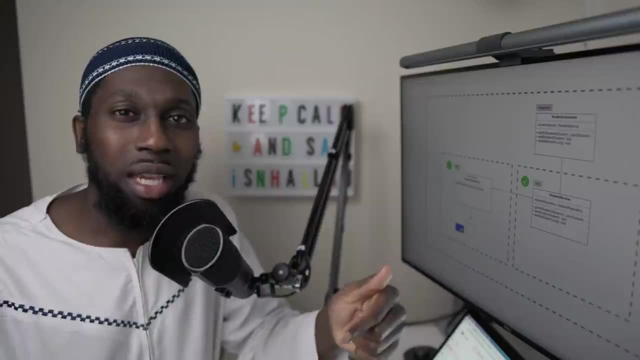 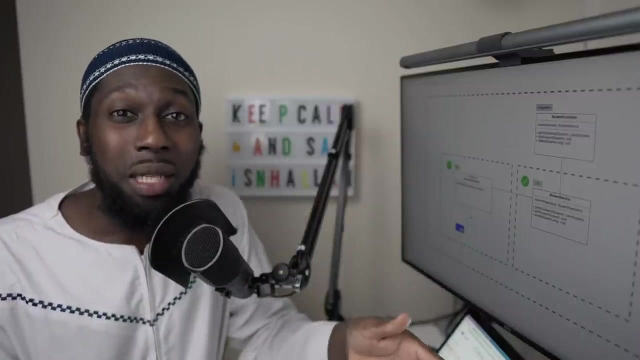 services such as Stripe and Twilio, and how to properly test those. If you are serious about becoming a software engineer, go ahead and roll to these two awesome courses. They are the best selling courses on my website and I'm waiting for you. This is all for now, If you enjoyed this video.